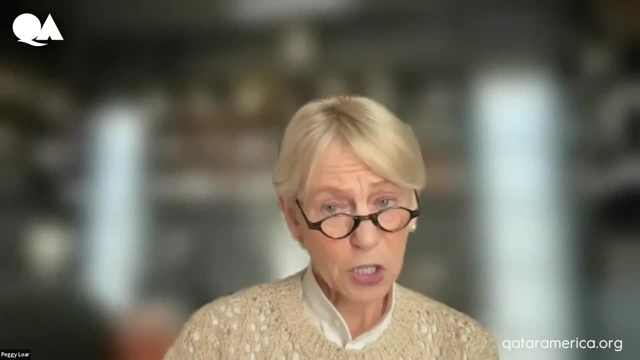 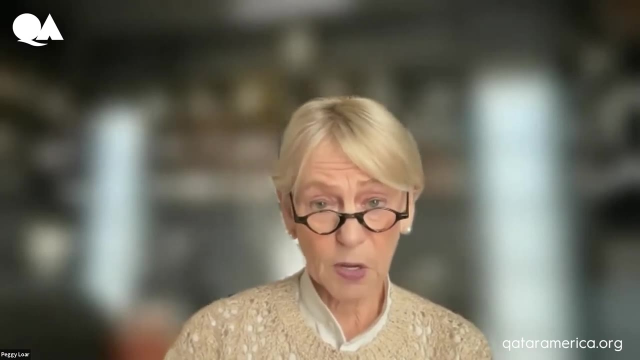 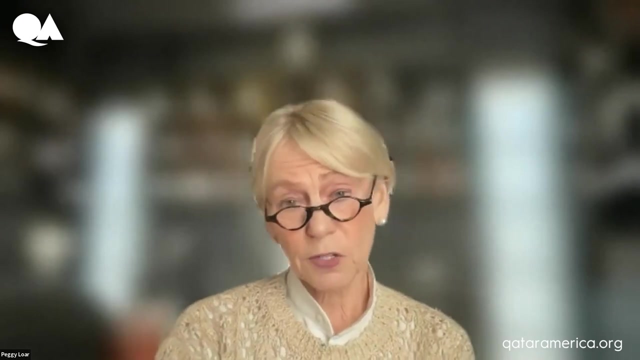 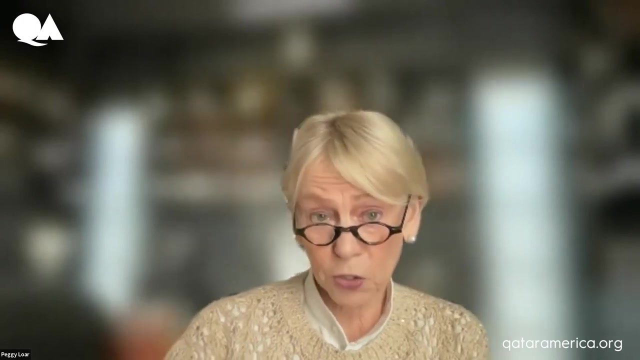 First, a word about CAIC. Our role is especially to connect the culture of Qatar and the US, but we also explore the culture of the broader Arab and Islamic world Through creative programming, working with artists and academics and a variety of professionals in the sharing of exhibitions, educational programs, film and interactive experiences that foster cross-cultural partnerships. 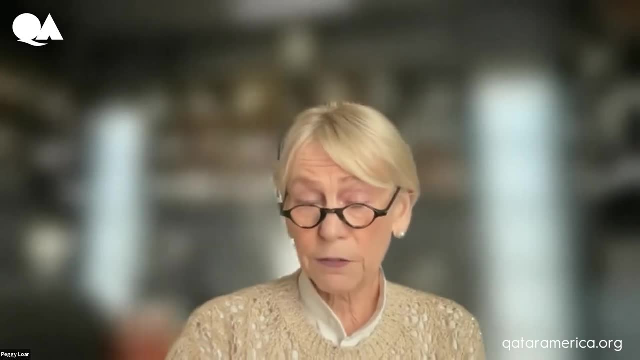 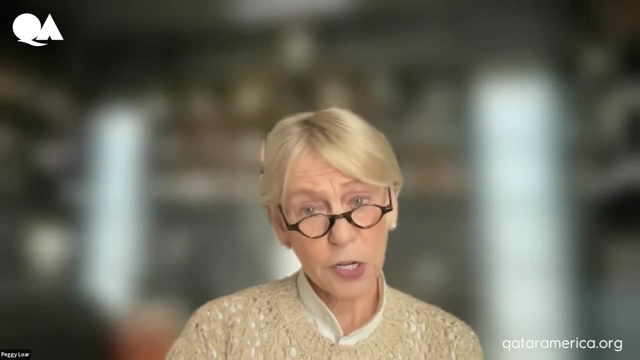 Today we will hear from three panelists on the creative, thoughtful process of museum programming for youth and families. Now, the idea of a children's museum started in America at the turn of the last century and the Brooklyn Children's Museum left. 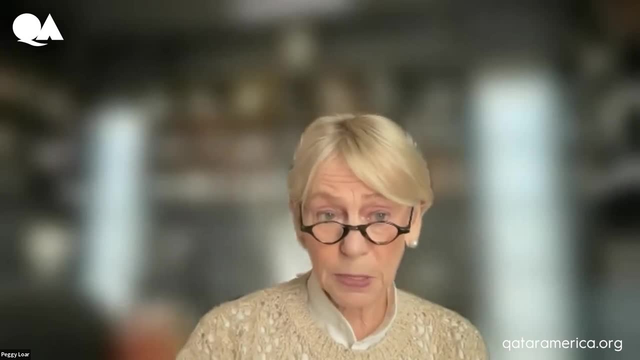 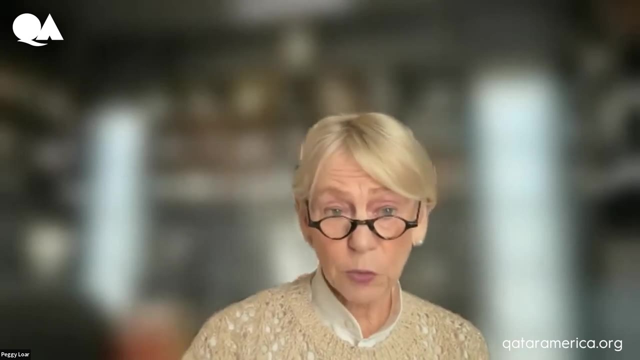 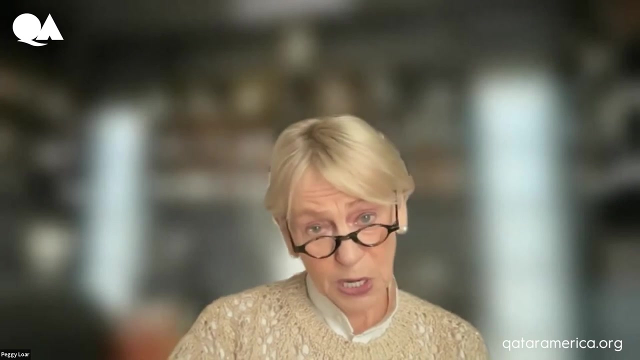 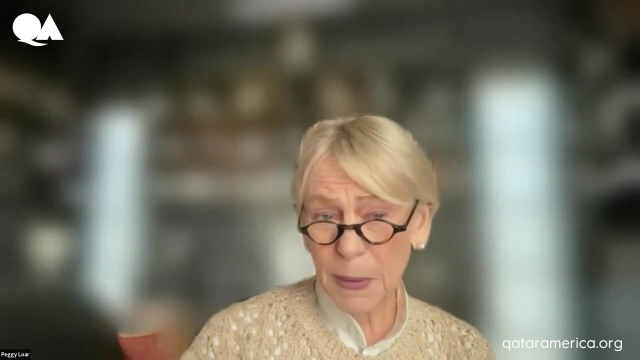 It is considered to be the first children's museum in the world. Soon after institutions such as the Boston Children's Museum influenced the establishment of a children's museum in Brussels, others in Europe and still others in South America. The largest children's museum in the world, and one that is loved by its community, is the Indianapolis Children's Museum, founded in about 1925.. I happen to be working at the Indianapolis Museum of Art decades ago. I am a director of the Children's Museum in New York City. I am also the director of the Children's Museum in New York City. I am also the director of the Children's Museum in New York City. 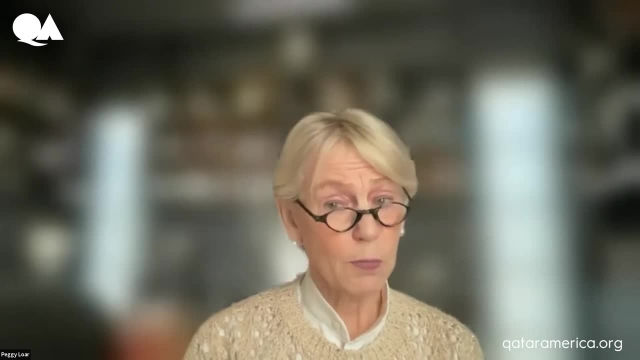 later, in the days of the Children's Museum's new emergence with its new building. Its programs were celebrated then and continue to be respected and admired by the profession. Of course, Lloyd Hezekiah of the Brooklyn Children's Museum and Michael Spock of the Boston Children's Museum. 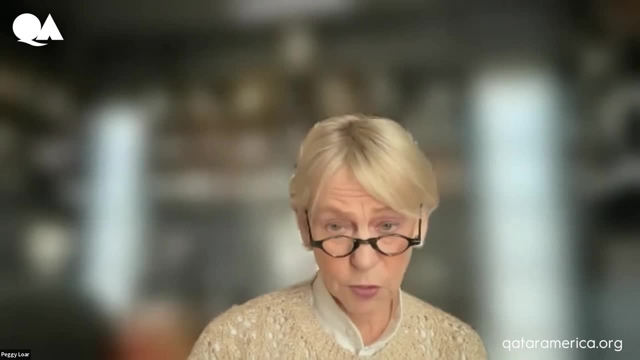 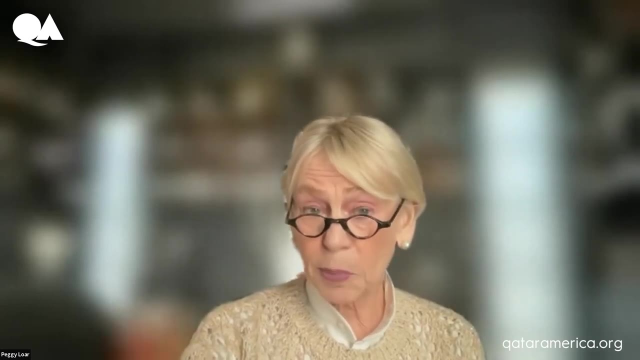 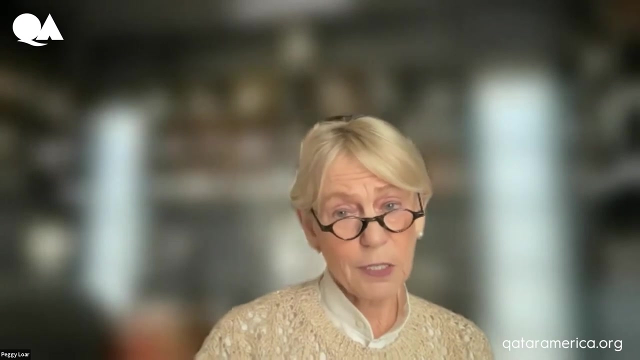 were two of the early pioneers and I'm so pleased to have known them both. We knew then, as we do now, that early interactive learning and the encouragement of play with learning encourages curiosity, makes long-term museum goers and results in good future global citizens. Of course, in 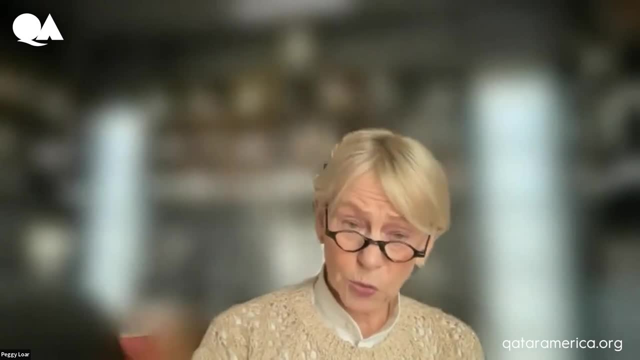 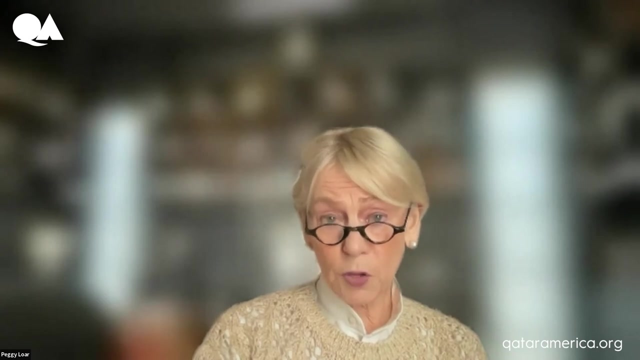 earlier days, most museums were simply not exciting for children, and that spawned a huge surge in museum education, such that major art museums and those others of other disciplines created specific programming for youth. We will engage in both of those perspectives today. I recall during my career as an 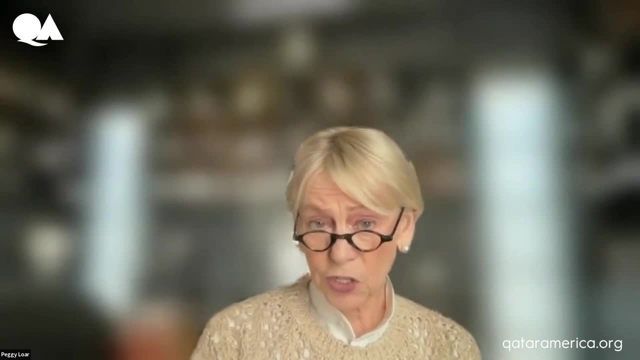 art museum director that I thought certain objects in the collection would greatly appeal to children if they were presented in the right way. So, over and above our children's programming, we built a special gallery and installed special objects just for them, creating an atmosphere that made 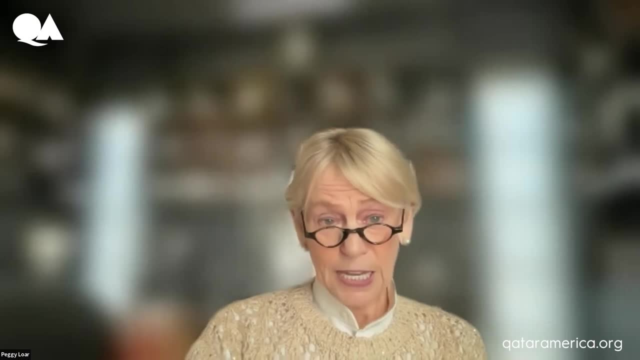 them comfortable, curious, even empowered. It had low ceilings and a low entrance door, so if you were not higher than about four feet you couldn't enter easily. Well, if you were four feet you could, but without parents, of course, and the kids. 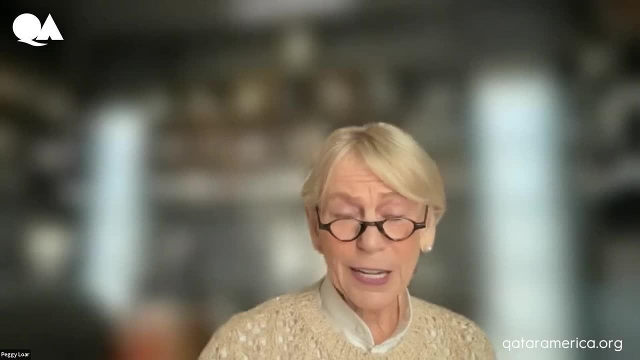 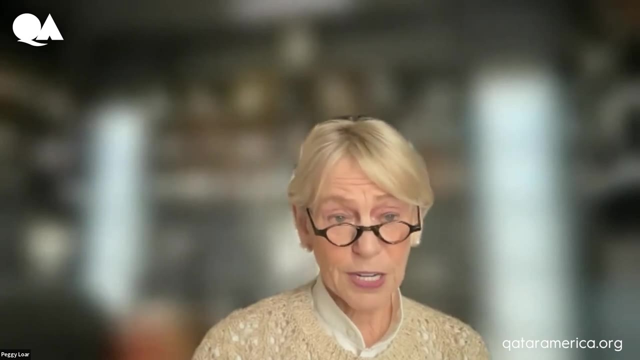 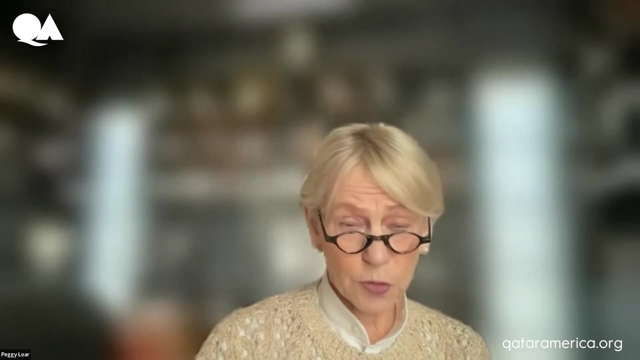 loved that. So let's introduce our panelists for their stories, their updates and their theories, And, following their presentations, we will have questions from the audience We have with us today, gerade Hanna Elwell, Vice President of exhibitions & Education at the Brooklyn Children's Museum. 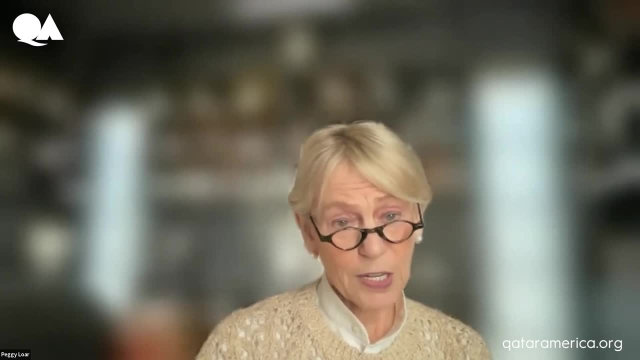 We have Clara Lim, Deputy director of Design & Development at the DADU, the children's resources museum community center, as I said earlier, and the actualcock distinguished throughout each of five years. Actually, without resources, But without parents, this could mean an much better level of. 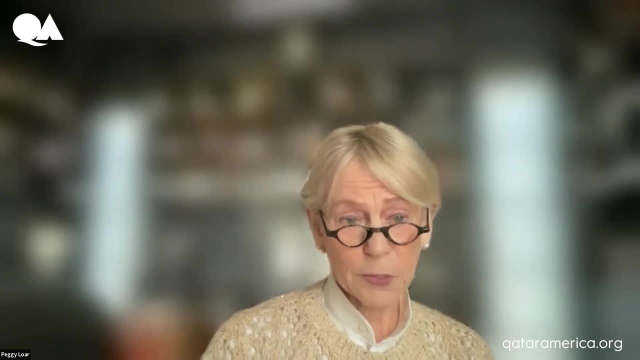 Museum of Qatar, Doha, and she is our replacement this morning for Iman al-Abdullah, who is head of schools and acting head of outreach, who was unable to make it. And our third panelist is Sheikha Nasser al-Nasser, who is deputy director of curatorial affairs at the Museum of Islamic. 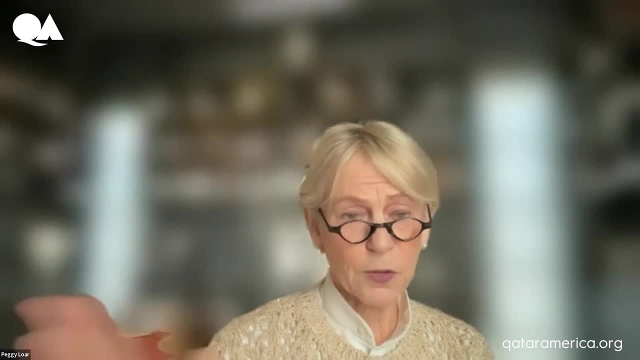 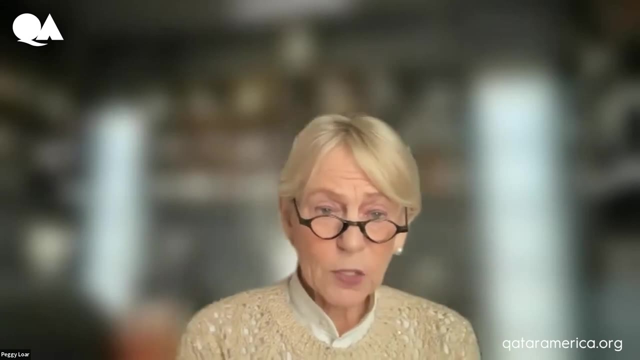 Art in Doha. So you can see, we have both perspectives from the Children's Museum side and also from an art museum that is doing children's programming. So we begin with you, Hannah, Hannah of the Brooklyn Children's Museum, and the screen is yours. 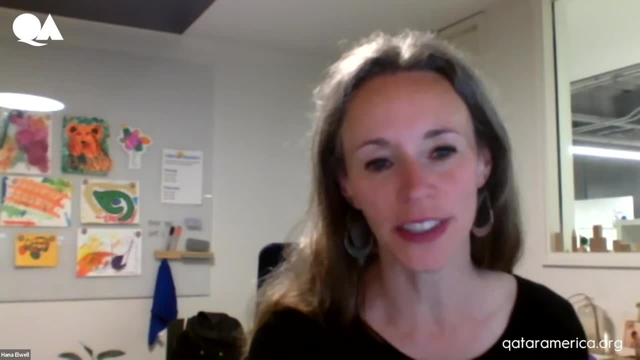 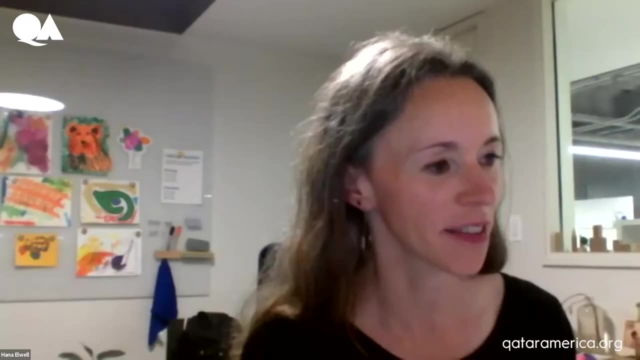 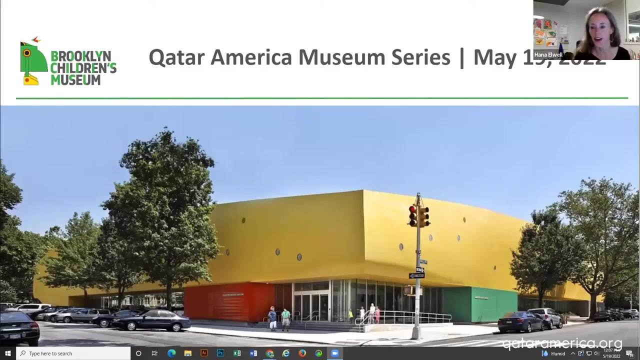 Hello everyone. I'm so pleased to join you today from Brooklyn, New York. I'm sorry it'll take me just a moment. It's not clear on the screen sharing. I should have confirmed this, So give me just a moment. Here we are. Are you all able to see? 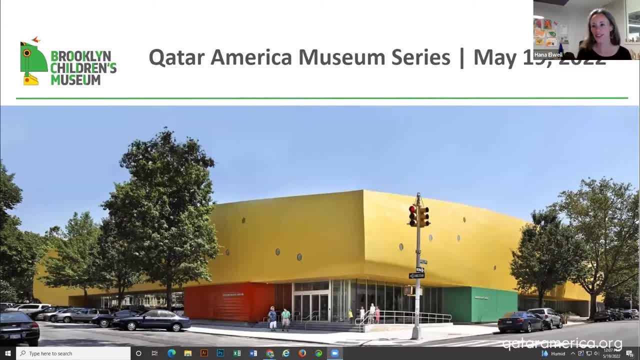 Yes, Apologies. Apologies for the delay. So so pleased to join you all from the historic, as Peggy said, the first Children's Museum founded in 1899.. We're very proud of our long history It represents. 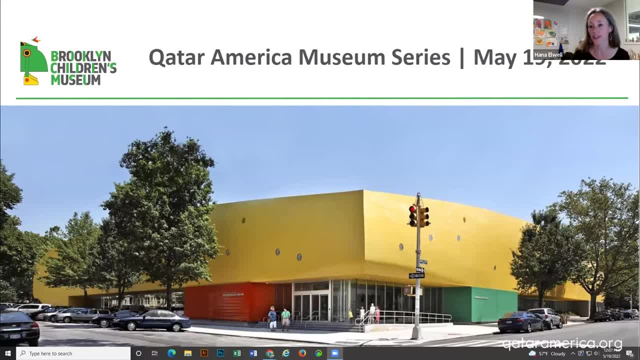 you know, so many arts of change within the field of education, ideas of progressive education and meeting families' needs and responding and engaging community- have changed so much over time and still very much remain at the core of the work that we do and the exhibits that we make and the programming. 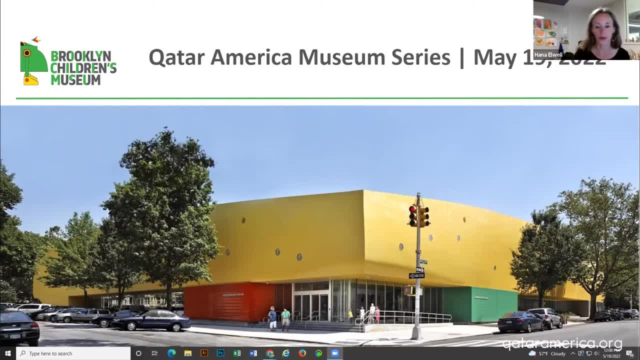 that we seek to present through, you know, engagements with partners and in the service of serving family audiences. So I'm going to show and share a broad swath of images and contextual information about our exhibits and programming, And we'll be happy to answer questions about any. 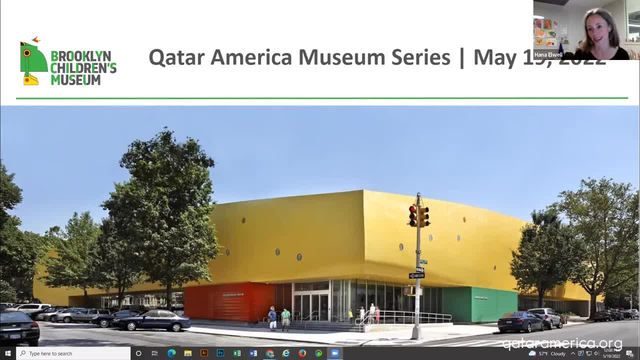 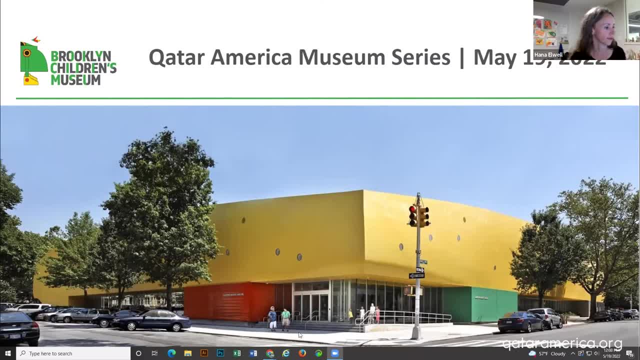 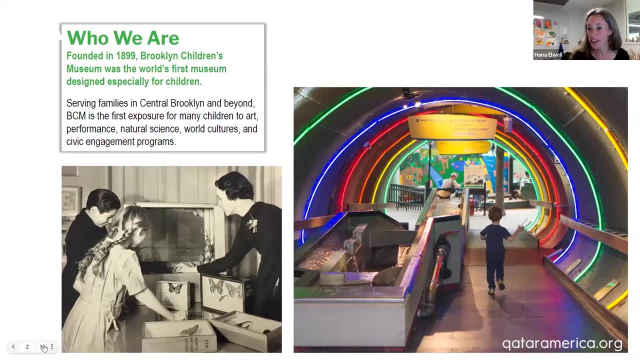 There's an image on the left side showing early activation of our collections. we've always been a collecting institution, which is rare for children's museums globally, but particularly within the US. our counterpart collection-based children's museums are Boston, as Peggy noted, and Indianapolis, both who draw on collections of cultural objects and 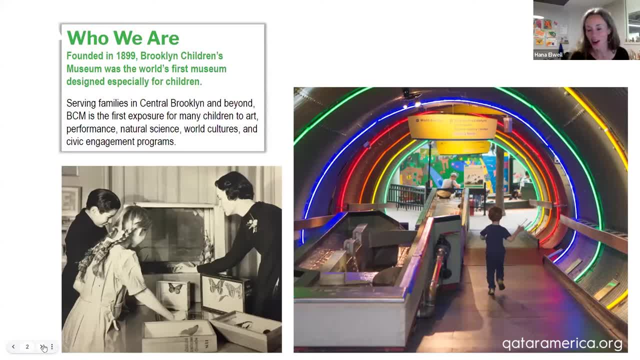 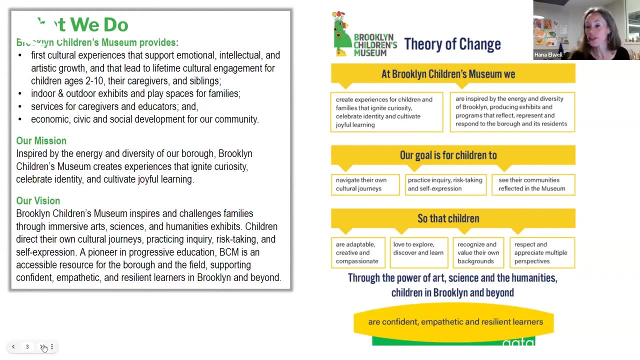 natural science material. So on the right side, this is our iconic people tube, this rainbow tunnel that usually has the thunder of children's footsteps running down it. What we do, We provide, first, cultural experiences that support children's growth, their socio-emotional 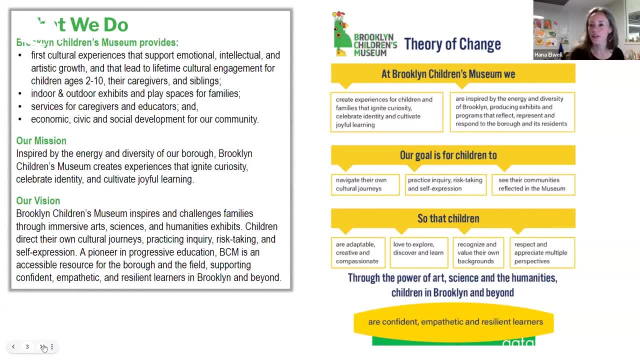 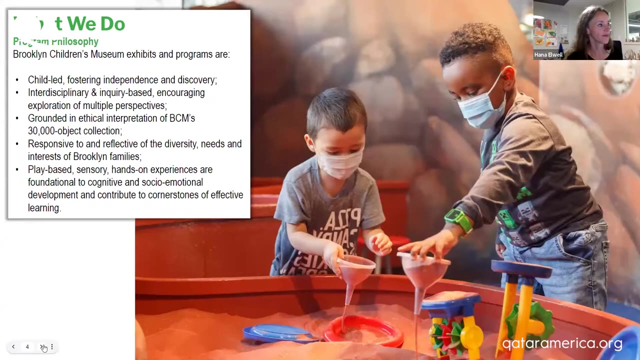 growth, their fine and gross motor skills, their curiosity, their creativity and their hands-on sensory exploration of the world. in all the ways We're inspired by the diversity of our borough and create experiences that spark curiosity and celebrate identity and cultivate joyful learning. 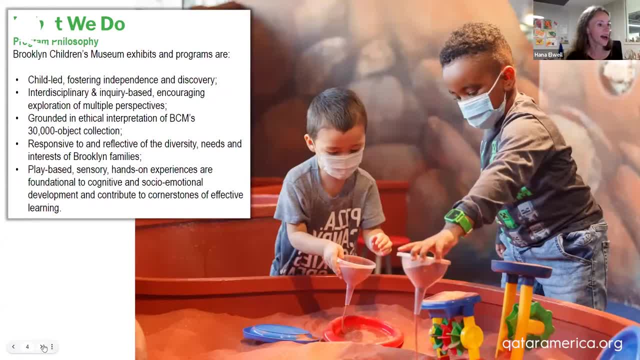 Our program philosophy touches on much of what Peggy noted. We foster independence and discovery. We activate our collection In a very intentional and ethical way. we think it's very important to honor the journeys of the objects that we're presenting and present them in an appropriate and respectful cultural. 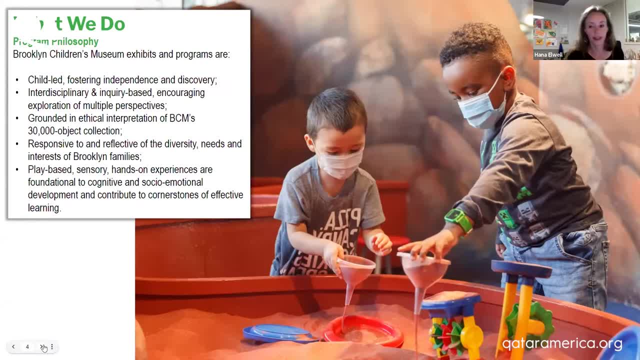 context. So we focus a lot of attention on that And we again want to be responsive to and really meaningfully engage the constituents in our communities, respond to their needs, what they're looking for and reflect a world that resonates with them. 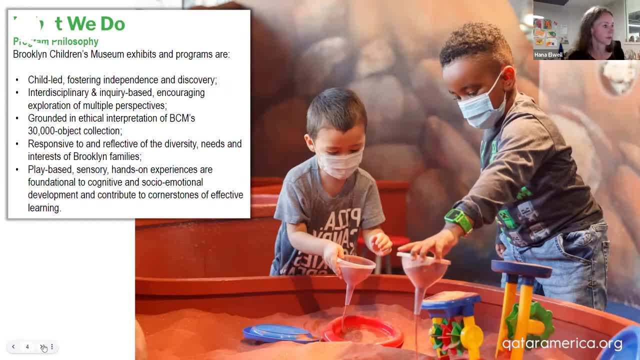 Through our exhibits and our programming. I'll walk you through our permanent exhibits. World Brooklyn is one of our iconic exhibits. It is a series of storefronts that represent real places in Brooklyn. Each of the places was created with based on first person narratives of the shop owners. 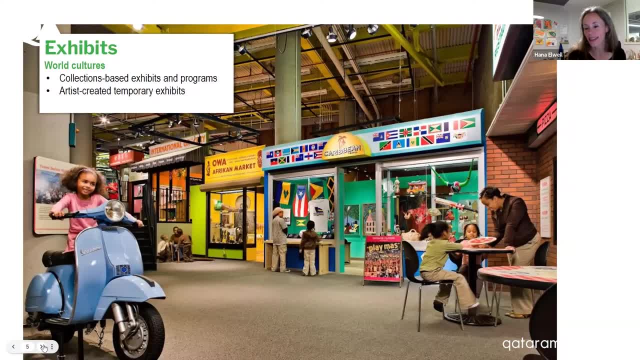 of the families who frequent those places, And so you can see the corridor of the storefronts. they have a little bit of a: There is a Chinese stationery shop, there is an international grocery store, there is a Mexican bakery, an OWA West African import store, a Caribbean travel agency and, of course, a pizzeria, the iconic Brooklyn institution. 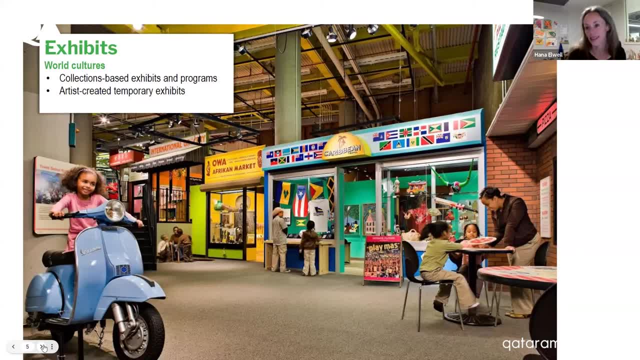 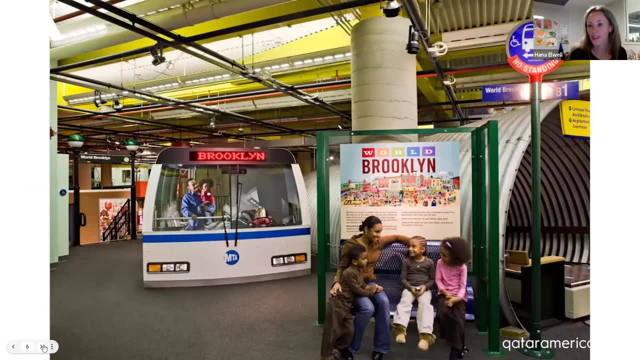 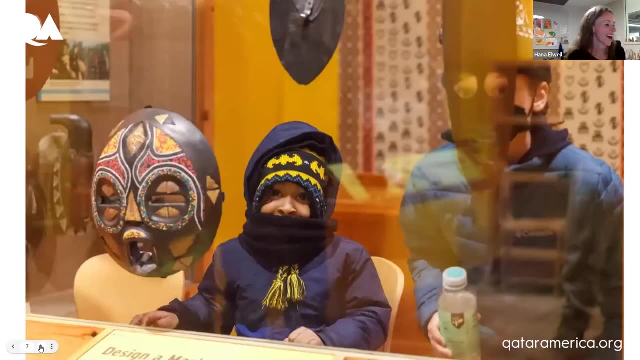 We partner periodically with these places that are also existing within Brooklyn. This is the threshold of the World Brooklyn Exhibit, which begins with a transit authority bus ride. I'm sure you know how much kids love vehicles And I'll just quickly go through some of the different interactive experiences within these particular environments. 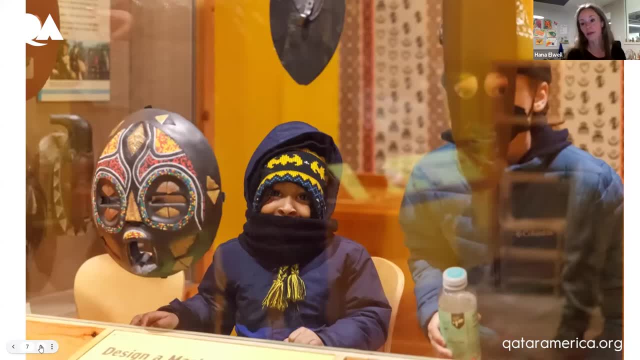 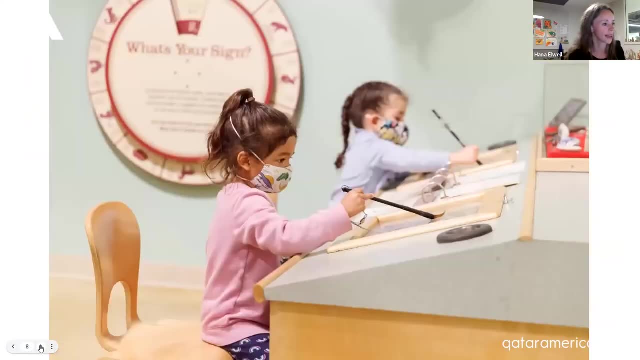 You're invited to look at a West African mask. look at the different shapes and textures and patterns used on the mask and then create one of your own along In the Chinese stationery shop. you're invited to learn a bit about Chinese calligraphy and try your hand at it with a water brush on a slate board. 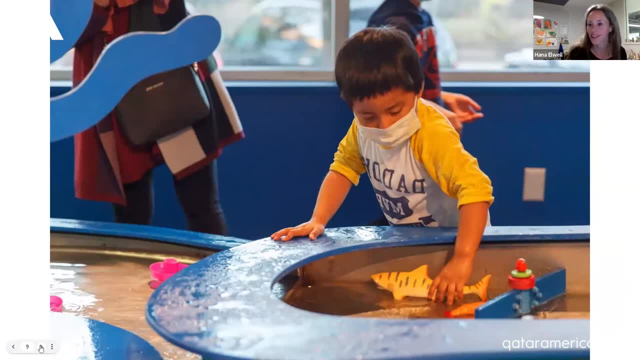 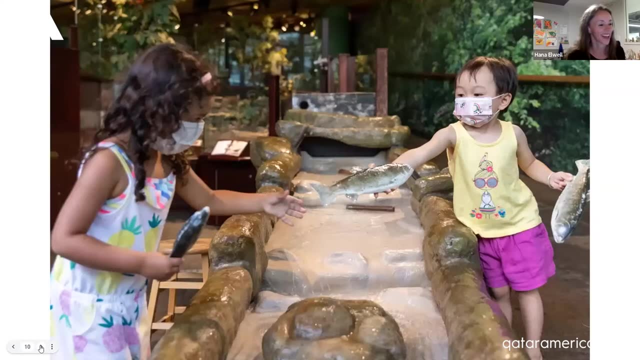 Sensory opportunities abound, whether it's water, sand, cork, You can make a mess here that you aren't making at home. The exhibit called Neighborhood Nature encourages kids to think about themselves as part of the neighborhood. We also do visiting exhibits in collaboration with artist partners. 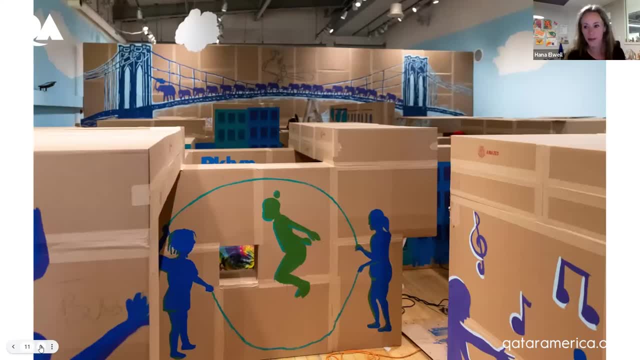 This was a corrugated cardboard maze in the works that we erected last summer. It was an inexpensive but very immersive opportunity for kids to explore and get lost, And we also partnered with an artist who created iconic paintings, representative of landmarks in Brooklyn that people would recognize. 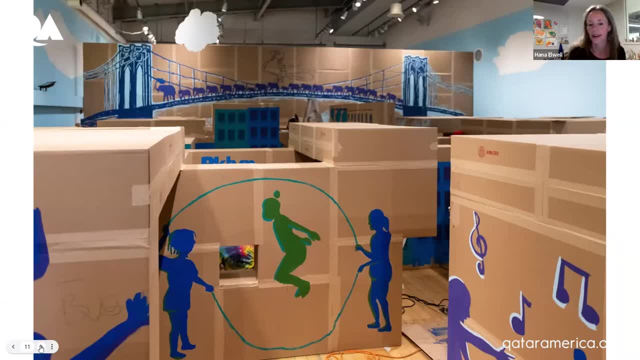 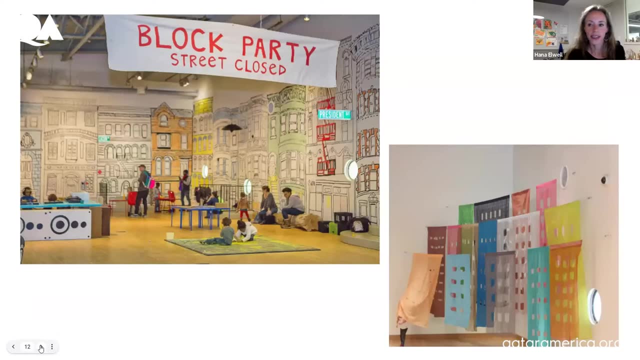 whether it was the public library or, you know, a building, landmark or the gateway to a park. And again, further examples of partnerships with artists: we worked with a local photographer who documents block parties, which are a very long-standing tradition in New York, and created an exhibit inside a block party within an under-arbor, which was a fun time. 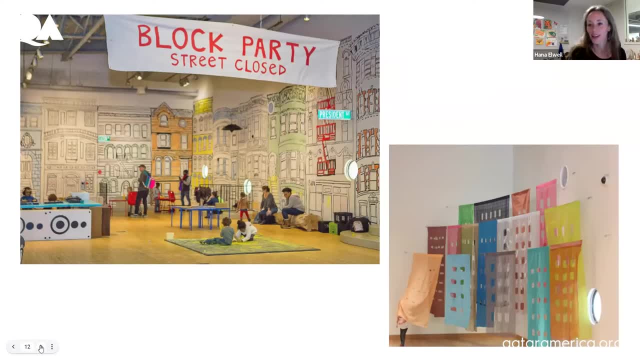 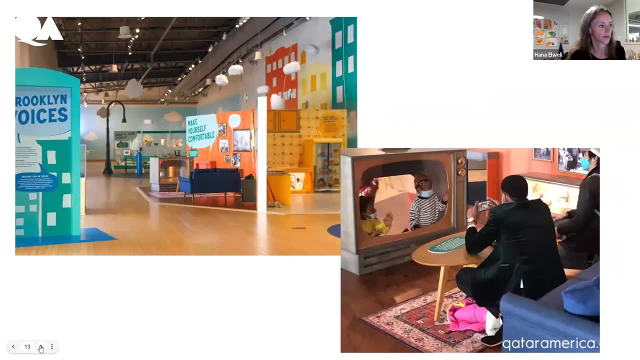 We had opportunities for sidewalk chalk or pretend, thrilling and, you know, serving food to neighbors and friends, music-making opportunities. This is our most recently erected exhibit, called Brooklyn Voices, which encourages kids to think about themselves and families to think about themselves as part of history. 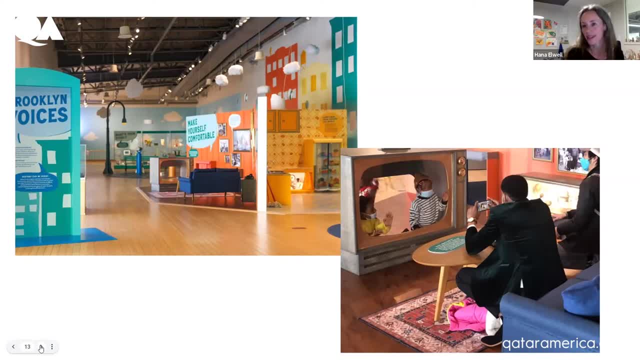 And the voices that contribute to this collective whole that is our community. So you can hear different voices through audio scapes. in the space There's a series of interior environments that are representing, you know, residential environments where you can engage in different kinds of role play. 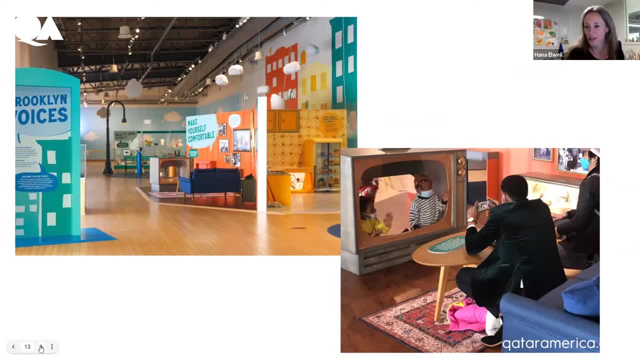 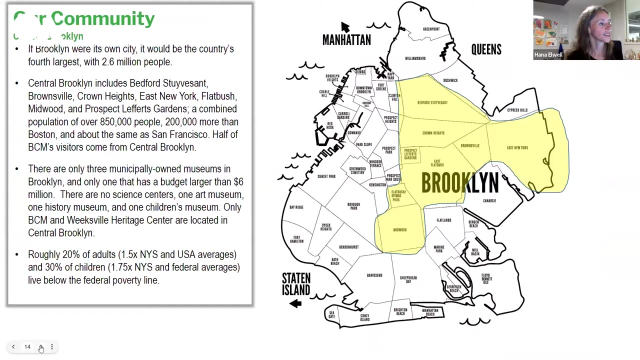 You see a couple of kids within the TV acting out the stories of their lives and it's been a really wonderful intergenerational opportunity for families to share experiences. Again, we serve central Brooklyn, which is about 8,850,000 people, larger than cities including. 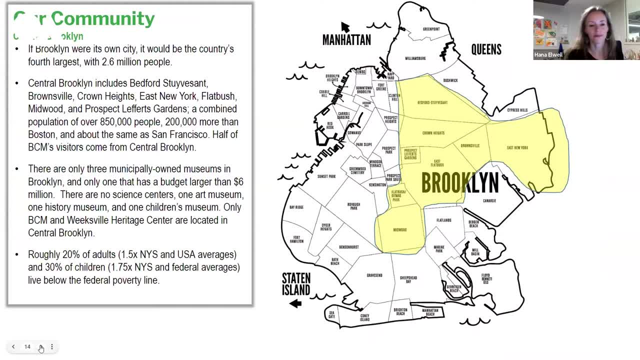 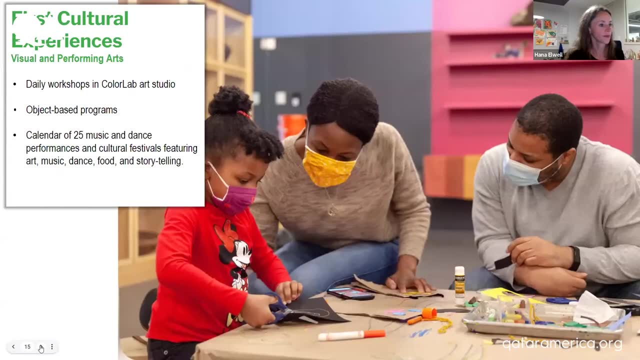 Denver, Seattle and others. So we're serving a lot of people within this small geographic area And we are one of the few places- one of the very few- that really are specifically targeting family audiences. So I've led you through the exhibits. I'll quickly share some of the programming that we offer on a daily basis. We have an art studio called Color Lab that highlights the work of Black artists. 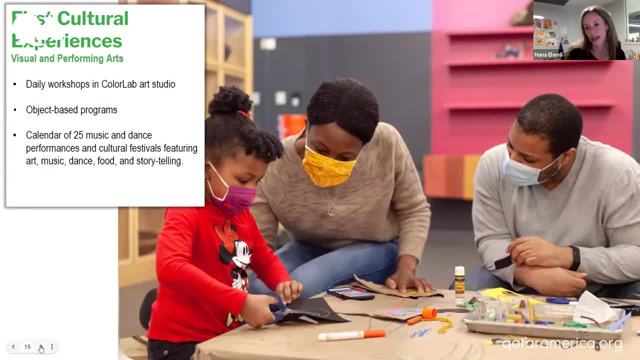 This was partially in response to school teachers and educators administrators expressing that there was an absence of art making spaces and that their students were not being introduced and weren't aware of artists that represented themselves, that looked like themselves And that felt something very important. 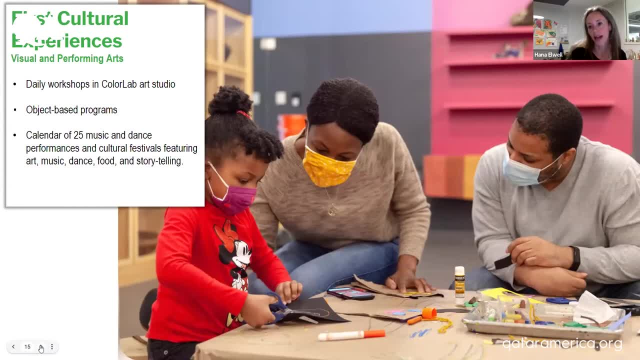 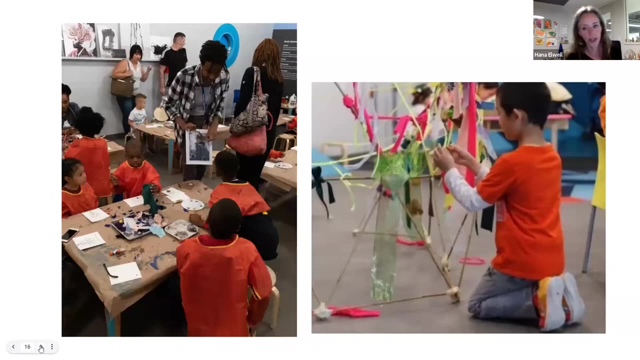 So we created the intention of this space: to highlight the work of Black artists, both New York based and globally, and present their work as news artists and do an inspired hands-on activity. each month We rotate them out. This is the studio space. You can see kids engaging in it. We offer school programs. We also offer rotating programs in a public program way. 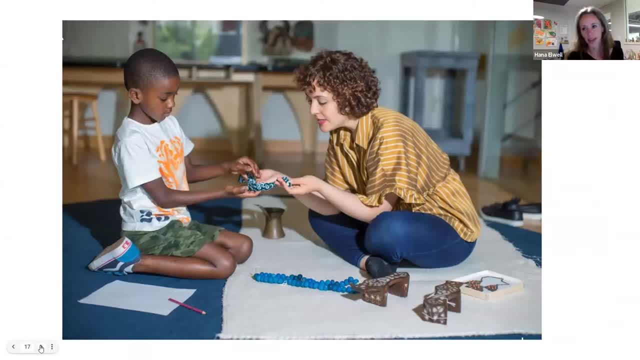 Here's a snapshot, a beautiful snapshot, of activating our collections. We believe that the utility of our collection is when it's in visitors' hands. That really the tactile experience of exploring objects, looking at their patterns, their texture, their touch, their feel, their weight, that that encourages both close-looking, expands visual vocabulary and really enables kids to activate their imagination to think about the path and travel of these objects. 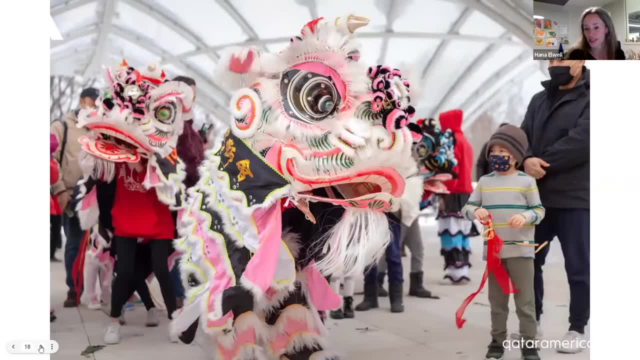 We also present a calendar of cultural festivals. We align our festivals with those marked by the Department of Education. This is an image from this past year's Lunar New Year. We partnered with the Golden Lion dancers from Chinatown and they brought their incredible puppets to our roof for a very animated presentation. 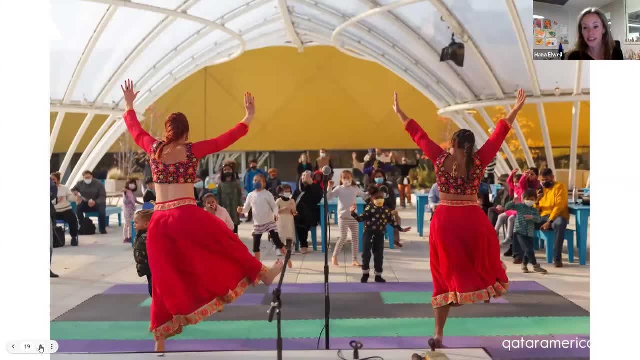 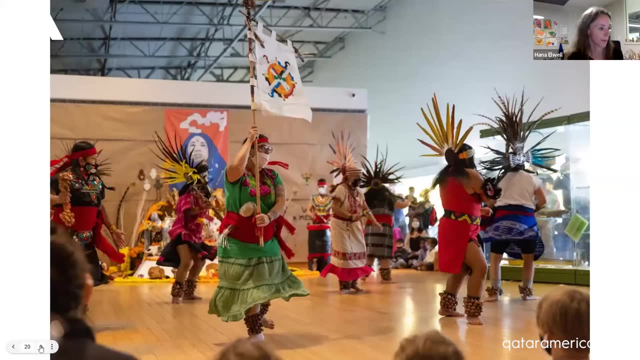 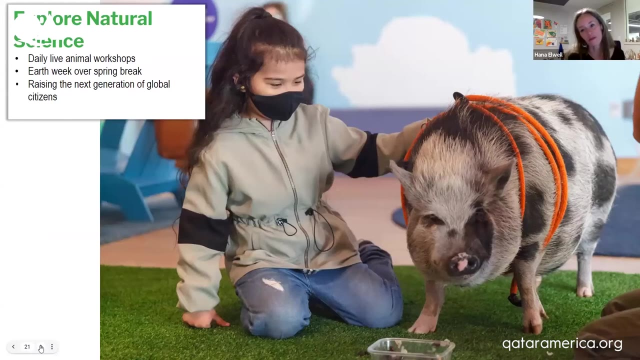 This is an image from last year's Holi celebration, The South Asian Festival of Holi. This is from Indigenous Peoples Day. We also have live animals. This is not one that's in residence at Brooklyn Children's Museum, but a special guest who came. 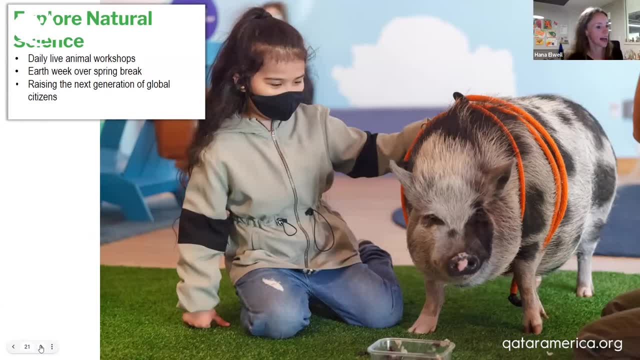 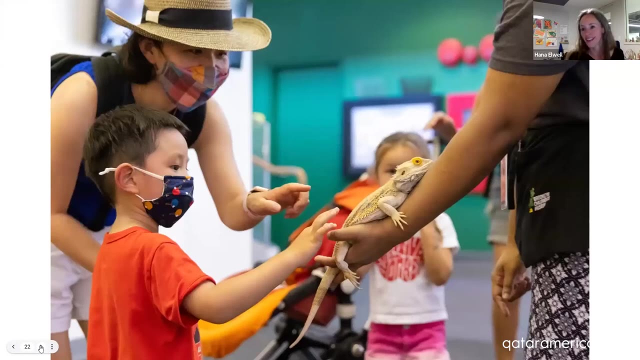 And was quite the sensation, as you can imagine. Who doesn't love to come to a children's museum and have the opportunity to engage with a pig, especially in an urban environment? Most of the animals that live in our museum are reptiles, so a little more accessible, and we bring them out for hands-on programming. 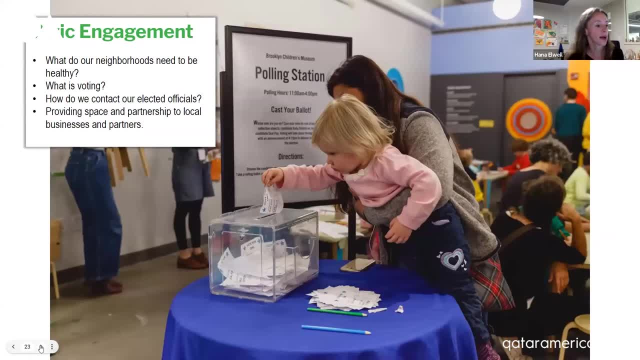 We also believe strongly in civic engagement. We do programming around Election Day We're really interested in. We're really interested in. We're really interested in cultivating the next generation of engaged citizens, Encouraging kids to really think about their voices and themselves as having agency and being able to impact positive change in their communities. 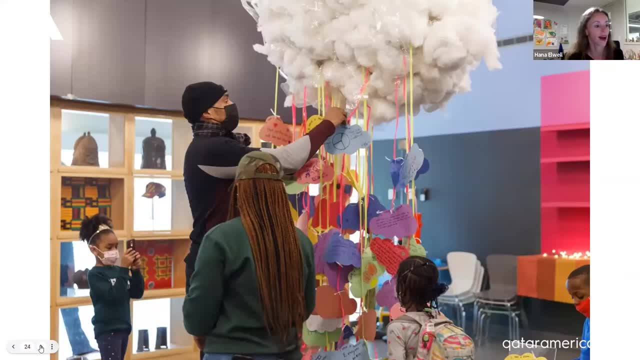 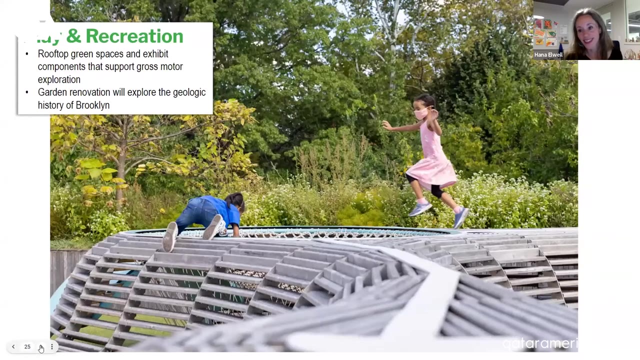 This is a dream cloud that we hung in our Keller Lab Arts studio for Martin Luther King Day and encourage families to think about their dreams- Dreams for themselves and dreams for their communities, for community betterment. We have outside spaces that encourage gross motor play. This is a play structure on our rooftop. The shape of it is actually inspired by one of the two chambered nests in our collection. 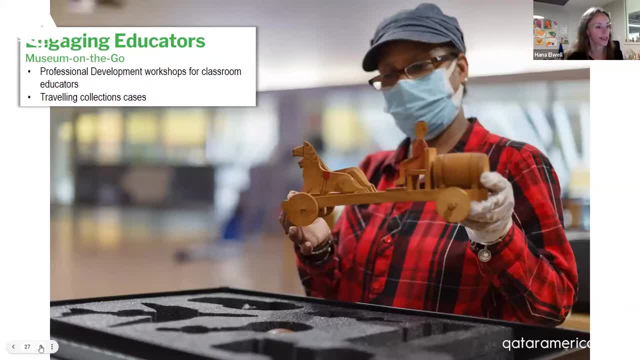 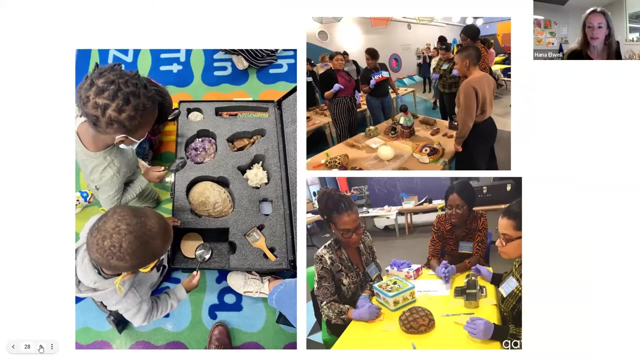 And we engage educators through a number of different ways. We do object-based programming, We have created collections, cases that they have brought to their classrooms. We do professional development workshops to encourage teachers to share with students- We have other teaching strategies- how they use these different objects in their classrooms, and I've put together a set of traveling cases, aligned with pre-K themes, that travel through different classrooms. 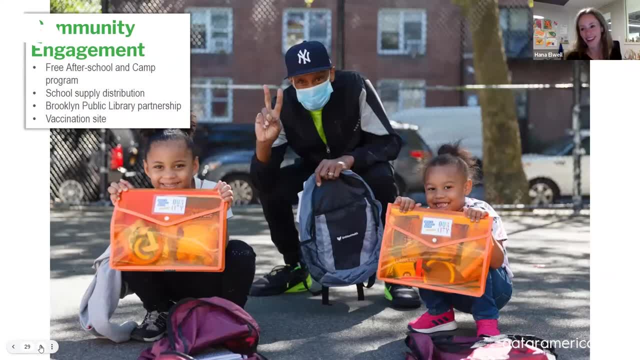 I don't want to be too long winded, so I'll quickly go through the remaining slides. We engage with our community in a number of different ways. During the pandemic, while many places were doing online programming, we quickly realized that tangible programming was really our best foot forward. So we put together art activity kits that we distributed to families through our community-based partners, and families really appreciated these. 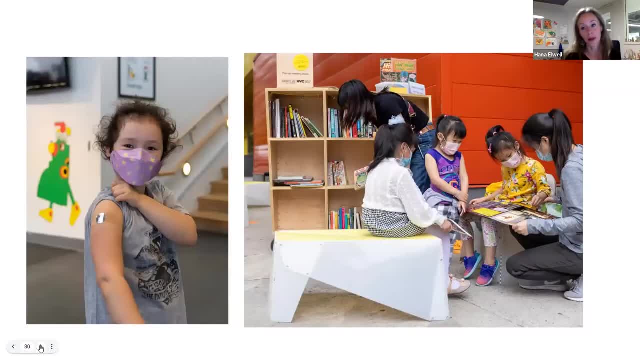 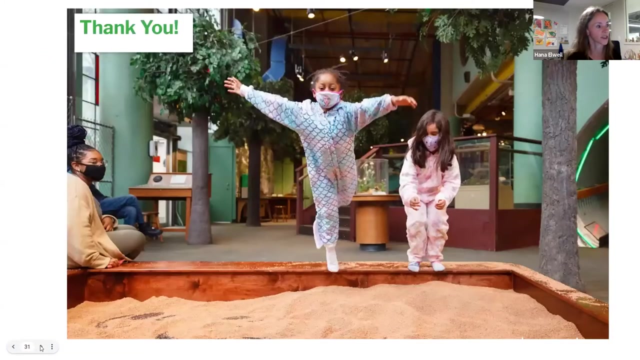 Adults appreciated them as much as kids. We have partnerships with the Brooklyn Public Library. They are actually moving under our roof and their branch will be in the same building, which will be a wonderful opportunity for shared programming And throughout the pandemic. on the left you see an image of a child who has gotten vaccinated. We've had a vaccination site which, for our community, has been a really powerful offering and an extension of community service. 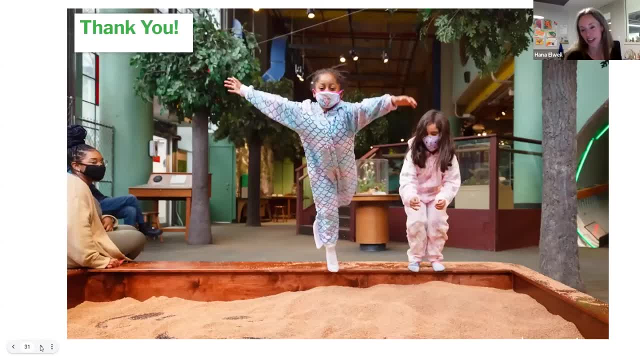 And so that is it in a nutshell, a very large nutshell- the scope of programs and exhibits at Brooklyn Children's Museum. Thank you, You know the museum has it does such a good job with programming and you have a very strong connection to the community. 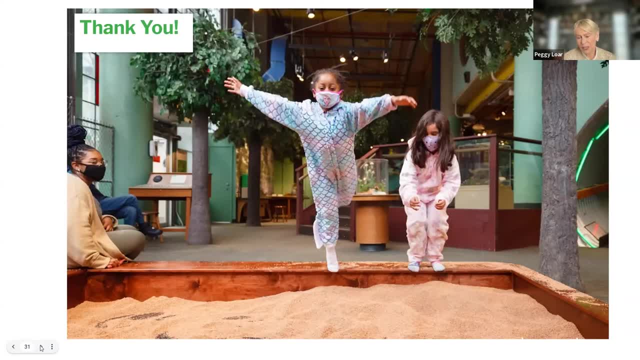 I'm just wondering how you get their feedback. Do you have any kind of evaluation or what do you do with that? I'm so glad you asked, because that's a facet of museum work that I have really grown to deeply appreciate in the time I've been here. 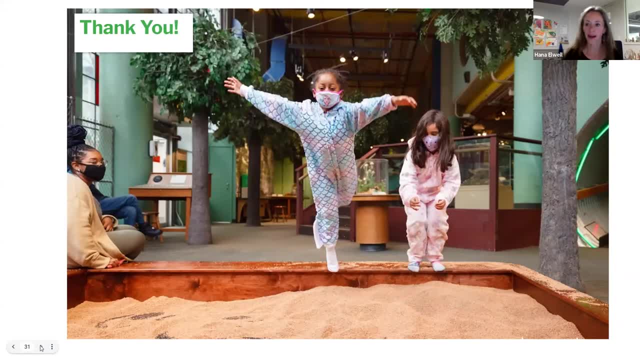 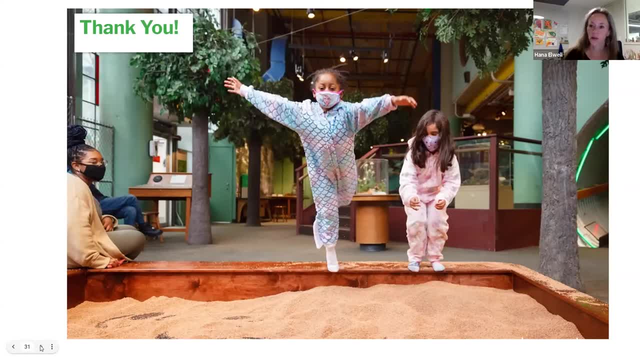 And so that usually counts to say, you know, whether we present an average aspect of ouravaliance to91 people Or whether we present a result one year later into our grants. So we are. we have the assurance that we'll be able to really measure up the goals against the outcomes and have both qualitative and quantitative data data points select. look at at the summation. 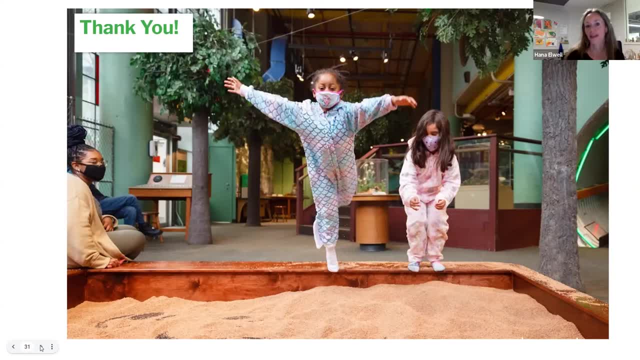 We want to be reflective about our practice and to build in evaluation steps along the way, So we've worked with a number of different independent evaluators and we also do our own evaluation when it comes to our community partners and visitor experience, As visitors are, you know, enjoying exhibits or coming for, particularly for a targeted program. 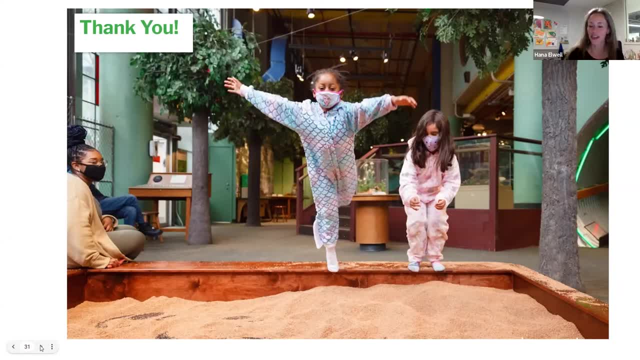 One of our cultural festivals, for instance. we're interested to hear if they are seeking celebration of that particular festival in other places And, you know what, how we might grow and expand our programming to meet their needs. That's great. Thank you very much. Stand by, but there'll be more questions later, I'm sure. Okay. 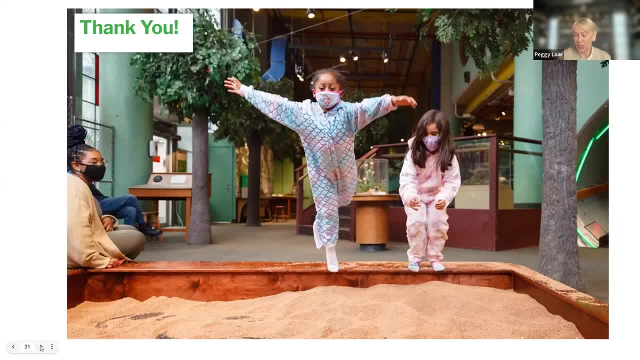 We're going to move on to Clara Lim who, as I mentioned, is from dadu, the Children's Museum in Doha, and she's deputy director of design and interpretation. so I hope she also gives us a window into the connection between the two, because design and interpretation. 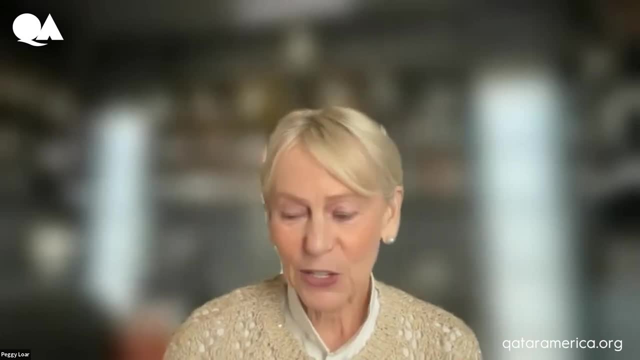 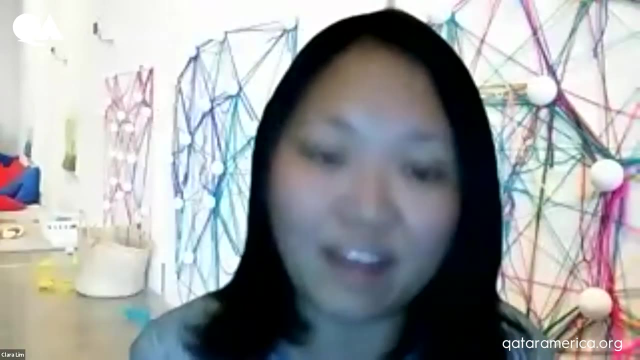 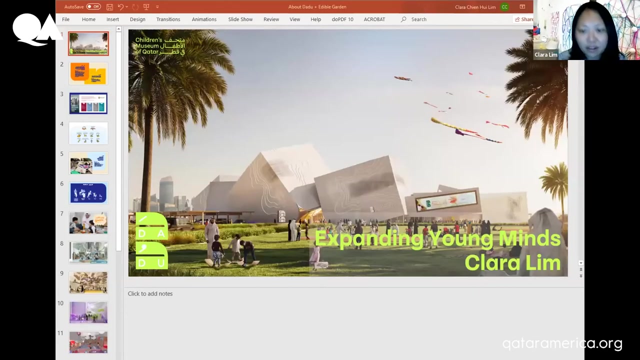 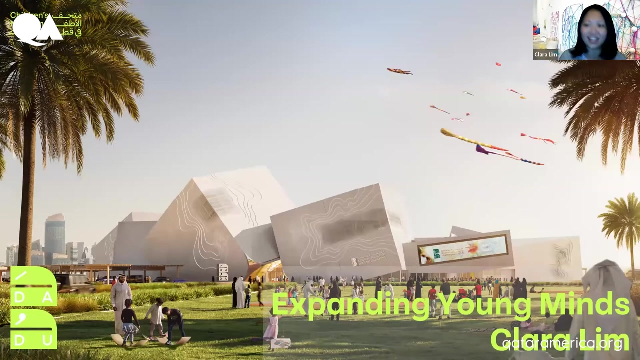 absolutely go together, no matter what kind of a museum you're doing. So there we are, Clara, The screen is yours Right, thank you. Welcome everyone. good morning, good afternoon and good evening. I'm just going to get my presentation up on screen. bear with me for a second and can I check that you are able to see it? the presentation for street Hannah's nodding, so taking it as yes. 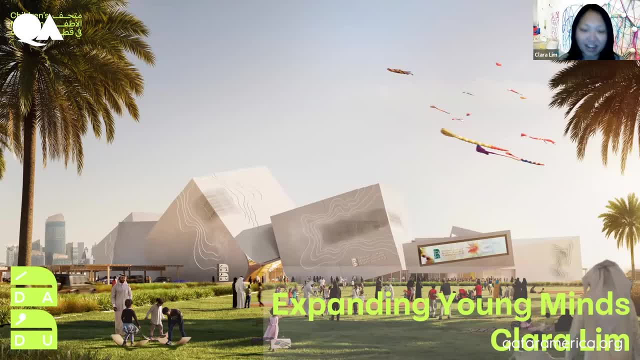 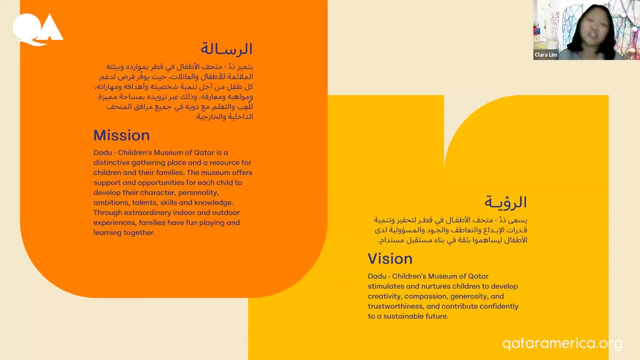 And so, firstly, I'm here on behalf of a man, Abdullah, my lovely colleague, who unfortunately is unable to make it today, But I try to live up to expectations, So that'll do. the Children's Museum of Qatar. What is our mission? our mission really is: we want to be a resource for children and the families in Qatar, and it's about supporting families, about giving opportunities to each and every child here in Qatar the opportunity to develop their character, their personality, ambitions. 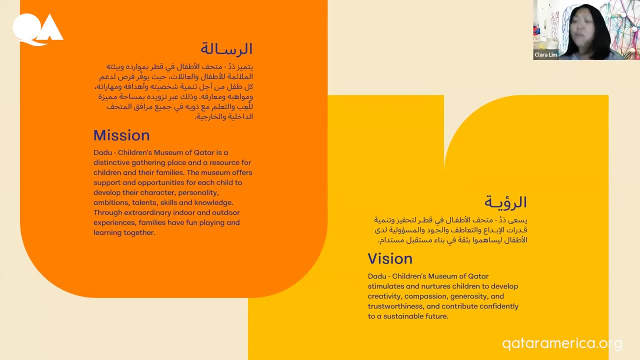 their talents, skills and knowledge come into play as well, but also really being a space of family bonding. And if we look at our vision statement, And I'm going to read it out to you, so that the Children's Museum of Qatar stimulates and nurtures children to develop creativity, compassion, generosity, trust with us and have the ability to contribute confidently to a sustainable future, 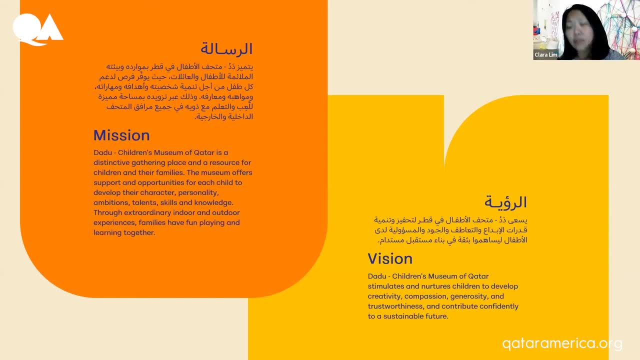 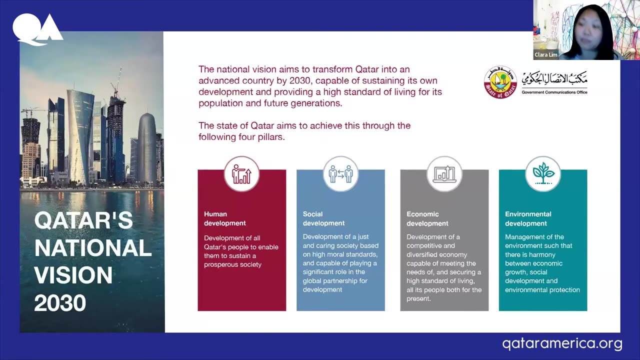 So a lot of these, all of these came really from stemming from the Qatar National Vision 2030.. So there is a vision that's there, has been set up by the government but the leadership of the country. So there is a vision that's there, has been set up by the government, but the leadership of the country. 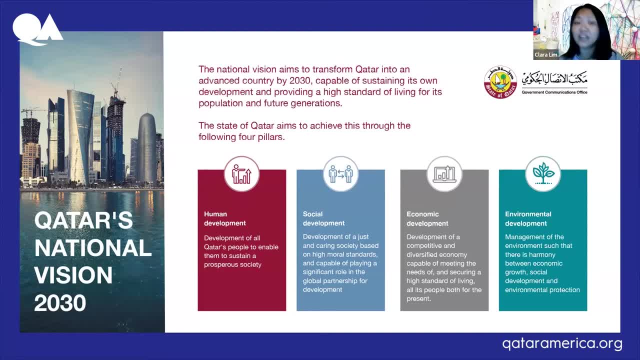 So there is a vision that's there, has been set up by the government, but the leadership of the country, To transform Qatar into the kind of country that it wants to see in, with full development pillars: Human Development, social development, economic development and environmental development. 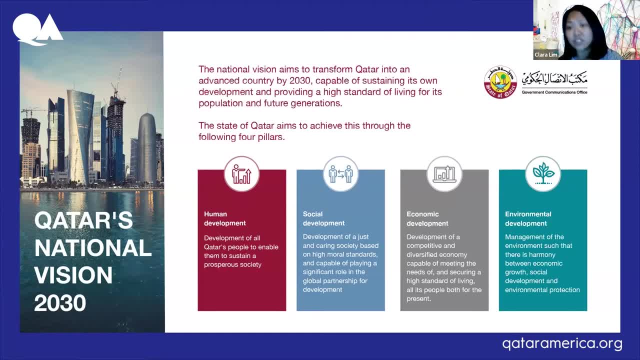 So a lot of work was taken to look at the national vision and delivery plan to say, okay, what does this actually mean in the context of children aid, who will be adults in 2030, who will have their own ways of contributing to the 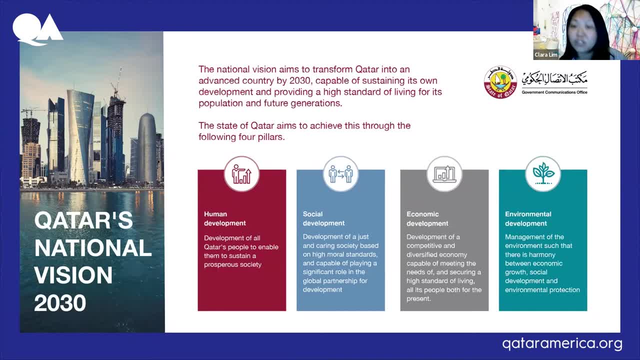 So a lot of work was taken to look at the national vision and delivery plan to say, Okay, what does this actually mean in the context of children contributing to the human, social, economic and environmental development of the country? what does that actually mean now? And through a lot of consultation with parents, with teachers, 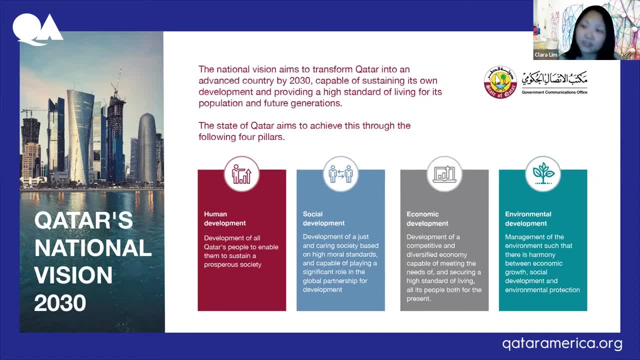 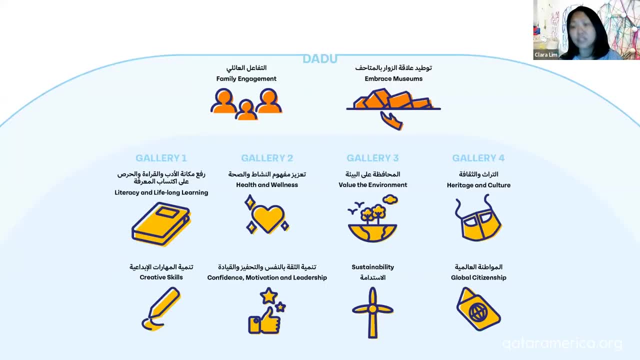 with community leaders, with thought leaders in the museum's field, in the education field, in the child psychology field, doing a lot of horizon scanning, we came up with our strategic aims for the museum. So I'm going to go through this with you. So family engagement is a huge. 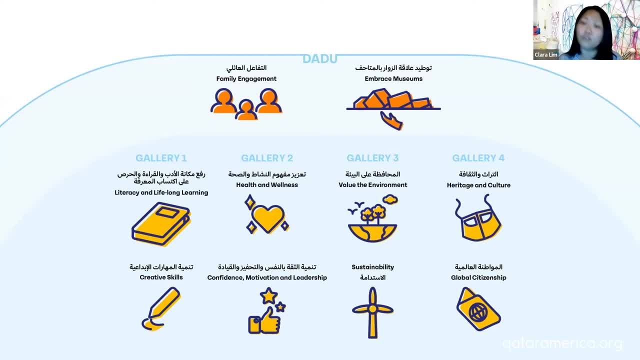 part of it, because a lot of these values were also drawn from Islamic culture, but also the Arabian culture. So bringing family together, bringing families together and giving them opportunities to bond and spend quality time together through playing is absolute key. Now we're part of Qatar Museums. I have my lovely colleague Sheikhan Nasser here today. 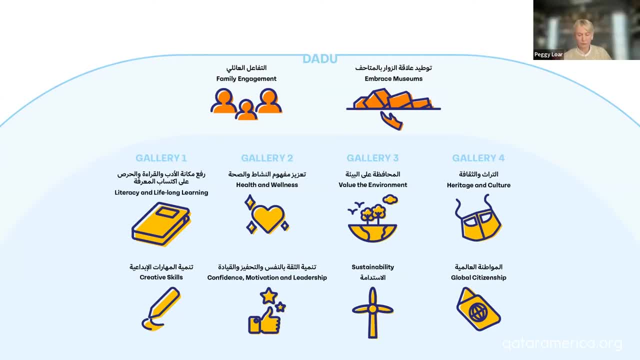 And we have other museums like the Museum of Islamic Art, the Qatar National Museum, the, the Contemporary Art Arab Art Museum And really what we see ourselves as is almost the stepping stone to our sister museums. From a young age, we want to bring the vocabulary We want to bring 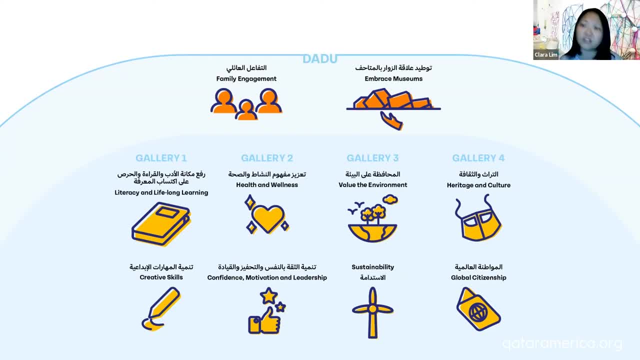 the habits of visiting museums. We want to bring it into the vernacular and the vocabulary of the children in the country. Now we then also look at eight other strategic aims. We are looking at literacy and lifelong learning, And when we talk about literacy and lifelong learning, we do not mean phonics, we do not mean 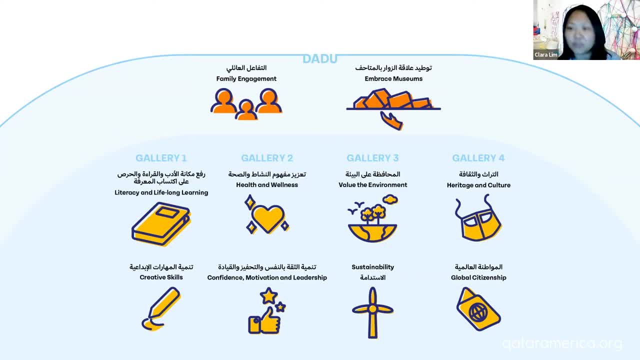 learning to read. We do not really mean you know the alphabets, Arabic or English. It's about us supporting the schools. It is about us demonstrating the value of literacy Using environmental graphics, using expression opportunities. Books are going to be, you know readily. 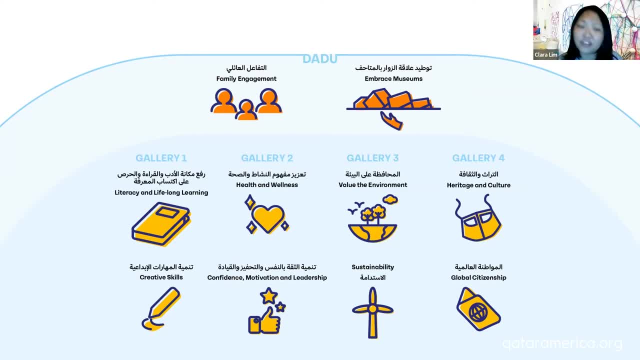 available spread out throughout the museum, But everything that we put in there is to serve as a, as a reminder of the importance of the learning process. I think this is an important time for us of literacy, of how enjoyable it can be and how it can support us in lifelong learning. 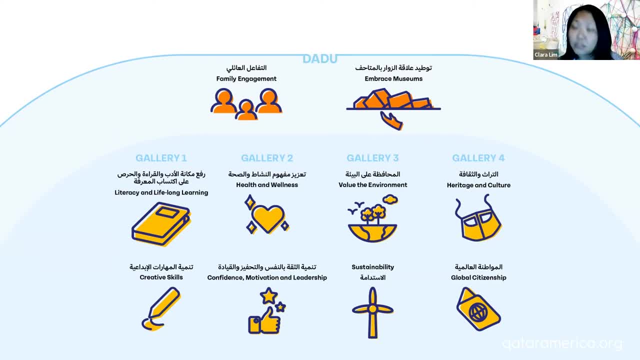 Creative skills is a huge part of Qatar Museums. We have our sister museum or fire station museum, Artists in Residence. We have M7, where a lot of design incubators are held, And we want to create the opportunity for children to not just develop their skills. 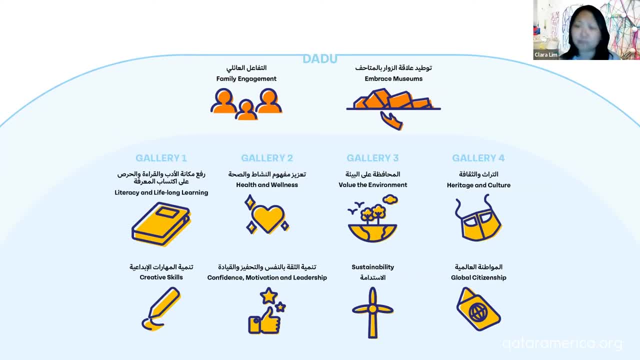 but to express their creativity from a young age. Health and wellness is another big aspect. I think after the last two and a half years, we all understand that physical wellness is as important. physical health is important, but really, you know, mental and emotional health is extremely important as well. 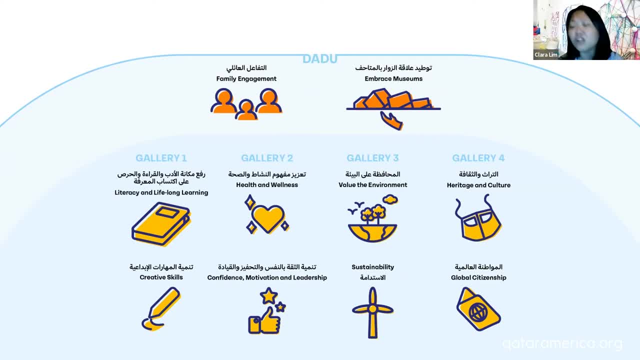 And so we've been working with the Yale Center for Emotional Intelligence to really understand how to be emotion scientists- And you know this is a part where we walk the talk of lifelong learning. A lot of us who have worked in the museum sector, a lot of us working in the museum, have been trained to really think about cognitive development. 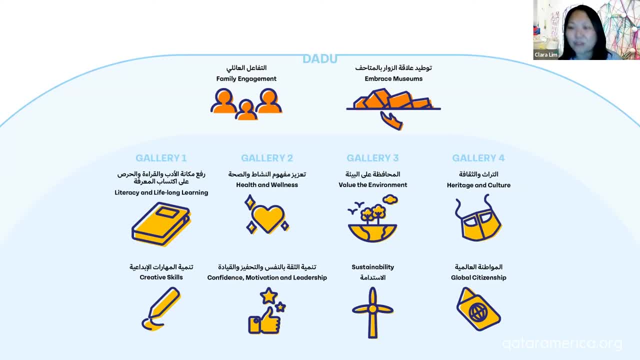 But we have not had the same amount of training and the same amount of research put into actually emotional well-being, And this is an area that we are very actively researching and very actively learning on our own. We believe that confidence, motivation and leadership is absolutely crucial to the children and youth for today. 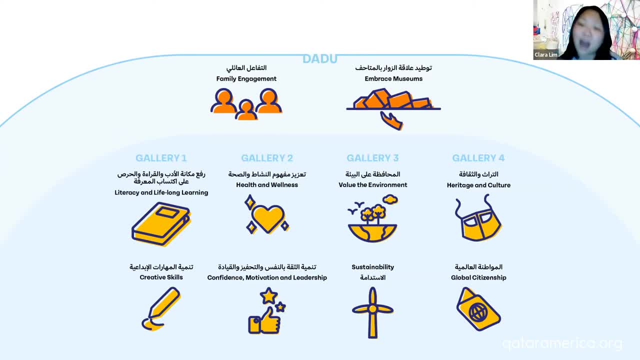 They need to feel connected. They need to feel that they have a part to play in the world. They need to feel that there is a future for them and they can be leaders. Working in the Children's Museum, we're often told: oh yes, it's so important to invest in children because they are our future. 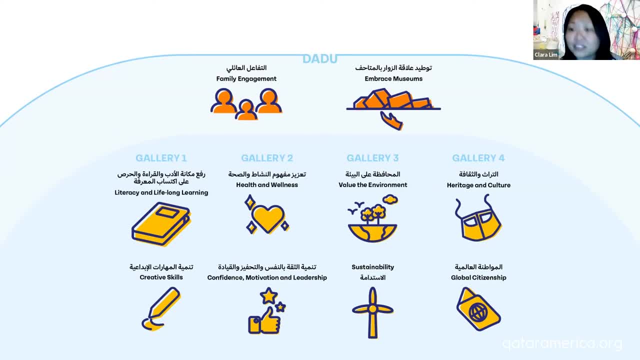 And we say, yes, they absolutely are. But they are also our present And they can be leaders today if we let them be. They have capacity, They have capability. They just need a platform to shine. Value, the environment and sustainability come hand in hand. 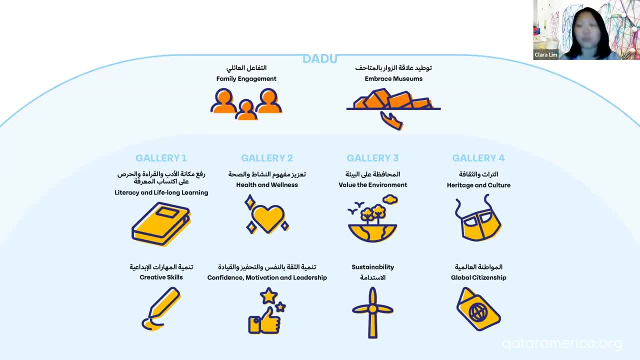 When we talk about value, the environment, we're stepping very much away of instructions of you have to reduce, you have to reuse, you have to recycle. But we are taking a different approach. We are trying to address nature deficit disorder. We're trying to have children reconnect to nature or at the very best, or at the very least, rather educate parents and talk to parents to say: listen, children do need to play in the world. 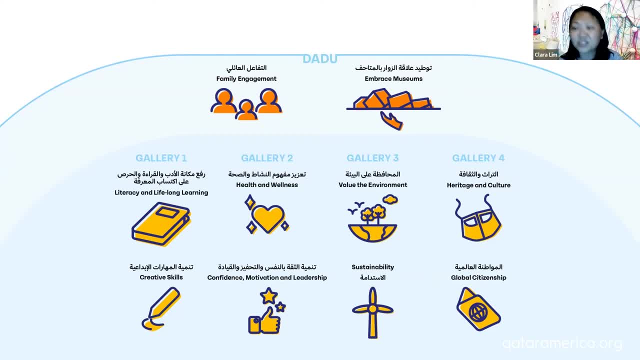 Children do need to play in the mud. They need to roll around in the sand. It's okay for them to fall off the tree. It's okay for them to scratch. you know pictures in the dirt with tree branches on their fingers. 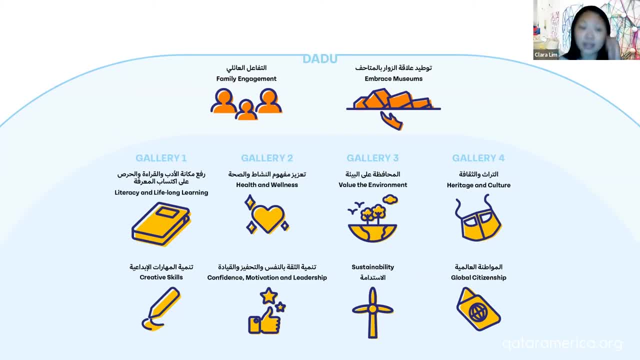 And to build this connection back to nature, Because it is this connection, it's this empathy, it's this value that they're going to be building for the environment and for the creatures living in the environment that will support them to make those decisions for sustainability. 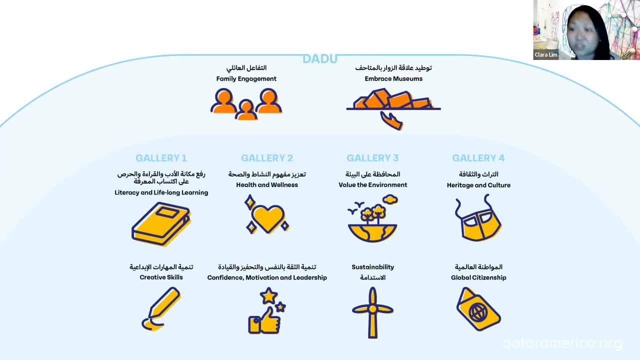 Because it's going to be economic, It's going to be sustainable, It's going to be economic sustainability, It's going to be social sustainability And it has to be environmental sustainability, hand in hand. We look at heritage and culture and global citizenship, again together. 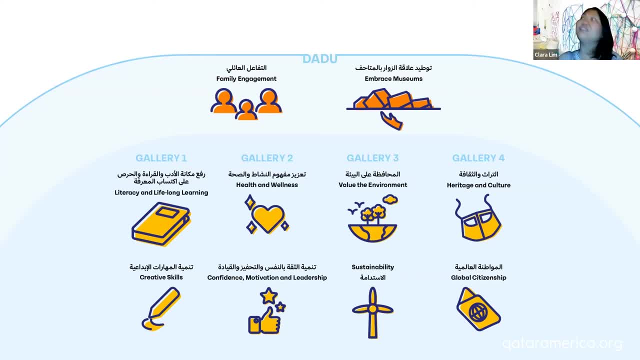 Now, there are so many different groups of children living in Qatar, whether it's in terms of nationalities or ethnicities. There are, of course, Qatari children, but we also have a great number of what we call the children of Qatar, not necessarily being a passport holder, but have been here living three generations. 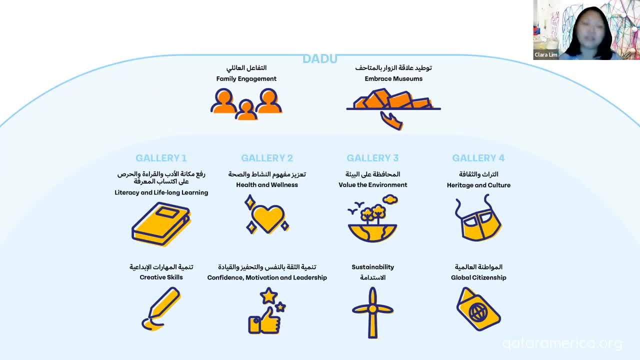 And this is what they know. You know they've got extended family here as well. There are also a lot of children who are on three-year cycles, So they're here while you know, dad's here on the oil and gas contract. 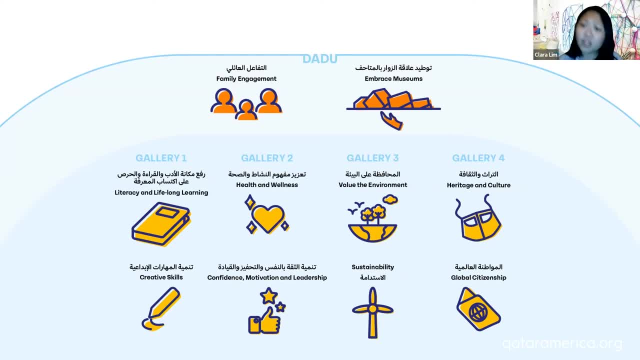 And then you have everything in between. So what does this mean to the Qatari children or the children who are here long-term to say goodbye to their classmates? every three years, Every year, half the class changes. What does that actually mean and feel to them? 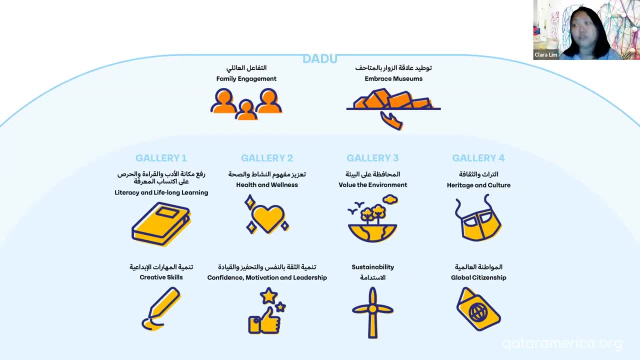 What does it mean for them? What does it mean to them? What does it mean for children who are born here and this is their world, but they're third culture kids, Parents, mom and dad both come from different countries. What does that actually mean when they're here? 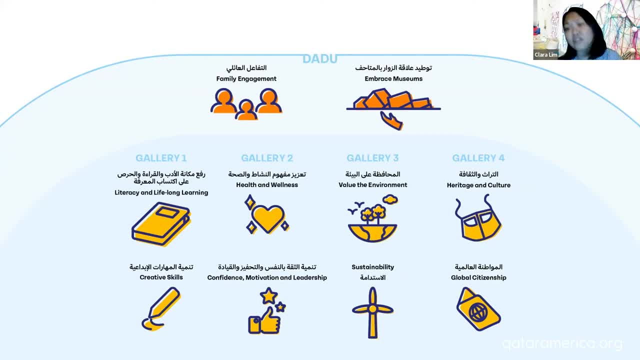 But then, whatever it is, we want to give children that confidence in their self-identity, in their family identity, in their community identity and also the Qatar national identity, so that they can be global citizens And they have that anchor from which they can confidently engage the world. 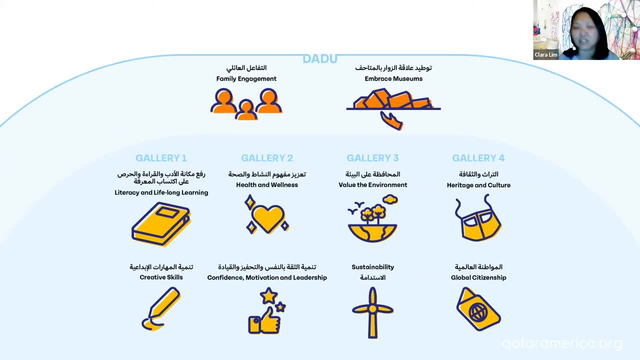 So you see that a lot of these things that we've addressed, there's a little bit of skills there in literacy and creativity, But really what we are articulating are values, And this is true a lot of consultation with people in Qatar. 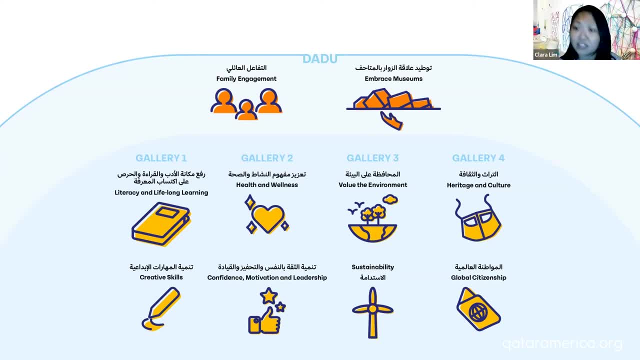 And it came true where parents and educators said: listen, the education system in Qatar isn't bad, You know literacy and kids are in school. What is really missing is how do we pass down these values that are really important to our country, to our family, to our communities, in such a fast-changing world? 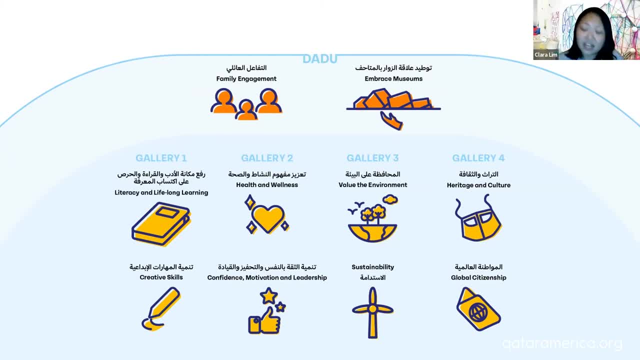 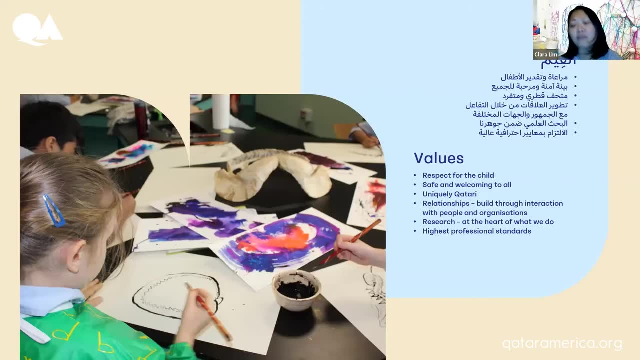 Some Instagrammers have more. you know, some parents say Instagrammers may have a bit more influence over some of my children than I do. So values comes into play Now. when we talk about values and when we want children to be developing values and family to be embracing specific values, we also have our own values. 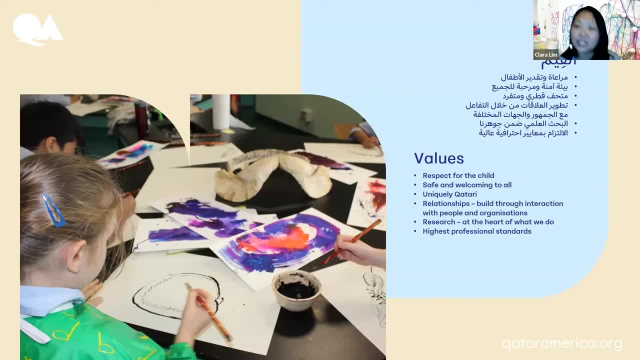 And we articulate this to say this is what we stand for and this is what we are working towards: respect for the child. So we have a great, immense respect for the capacities of each individual. Again, coming back to the statement we said earlier, you know, children are the future. 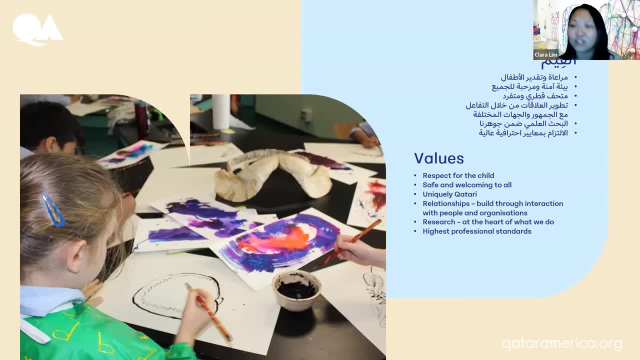 They are also the present And if we give them the platform, they can do great things. from today, We want to be safe and welcoming to all, So that's inclusive and accessible. We want to be uniquely Qatari, So while we have visited Hannah and her amazing establishment, we have taken a lot of her ideas. 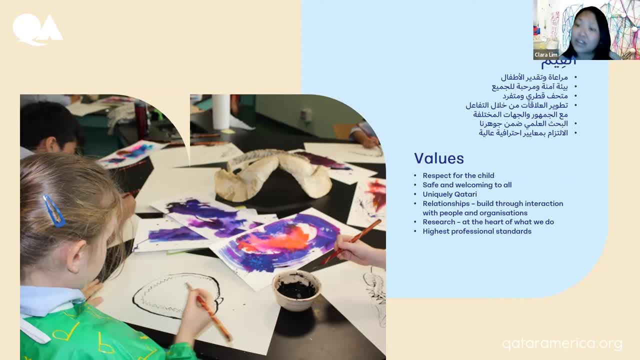 But they are made specific for the children and families of Qatar, Through the lens of which The families here will want to explore these contexts and these exhibits. For us, it's about relationships. Relationships is a huge part of what we do. So we talked about extensive community engagement and consultation with the communities. 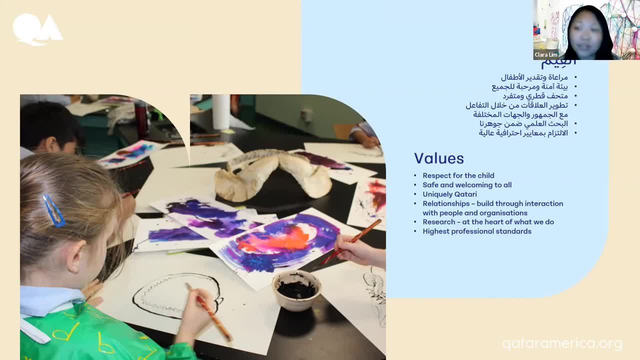 We also work a lot with allied organizations, whether they're schools, whether it's the Ministry of Education, or whether it's special needs groups or whether it's community leaders. We are very much open to working with anyone who has an influence with children. 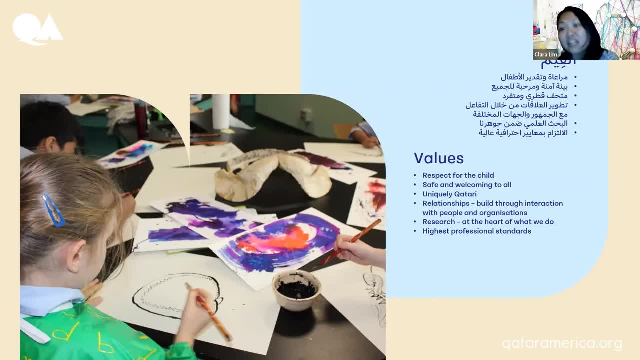 Research is at the heart of what we do. So learning from other organizations, Learning from Brooklyn and Boston Children's Museum, but also the Children's Museum in Singapore, in Korea, around the world, But also really looking at what does the latest play research tell us? 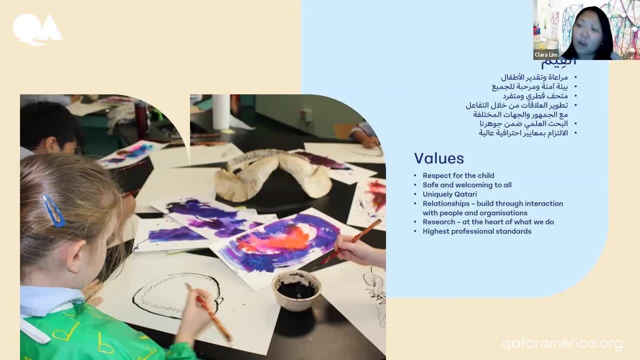 What does the latest child development research tell us? What are the latest thinking around progressive education? And we hold ourselves- we like to think that we hold ourselves- to the highest professional, The highest professional standards, And that may be either as an educator or museum professional or a designer. 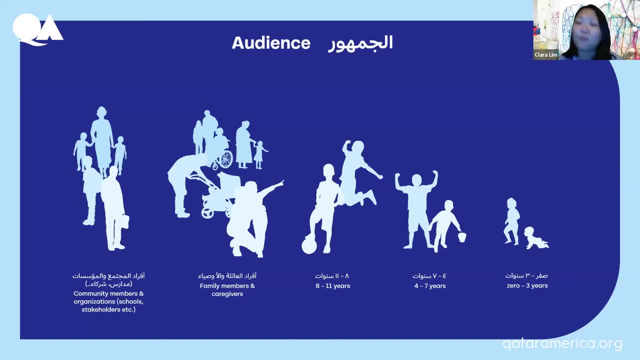 So who are our audience? When we talk about families, you know it's a catch-all term, But we are very specific For now, where we are still in development phase. we are focusing on children aged 0 to 11.. 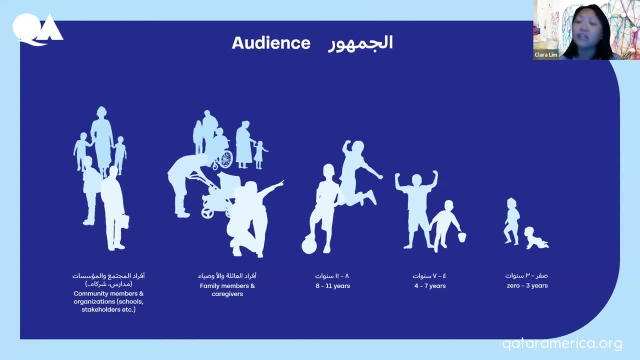 We do want to engage youth, but right now, we feel like this is the provision that is required in the country and where we can make the greatest impact. But it's not just children to 11 years. Well, this is our core audience. 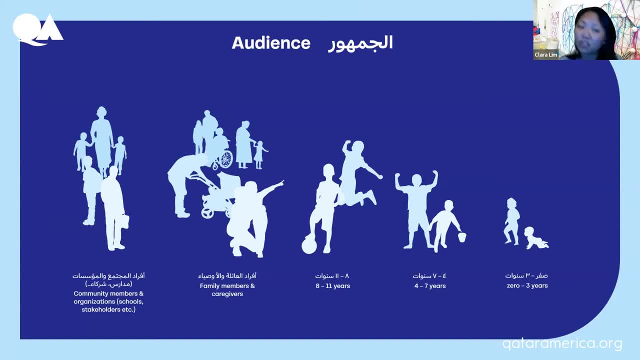 We are also looking at family members, caregivers, community organizations, the schools, carers, grandparents, nannies, whoever it is. These are people who have great influence over children's lives, So they are part of that village, just as we are. 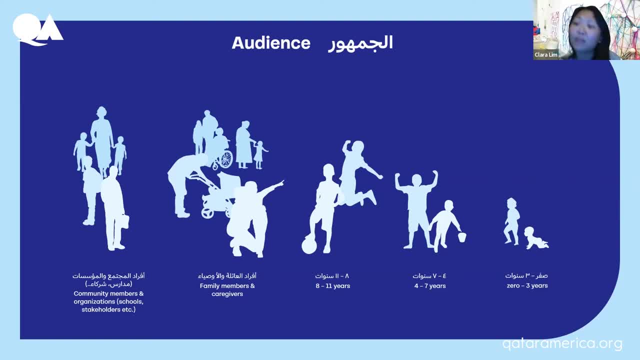 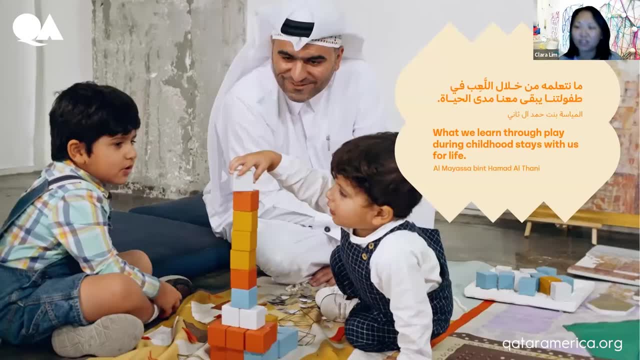 It takes a village to raise a child. We are all part of this village, And how can we support each other? So what is the one thing? that Children's Museum. you know what is our approach, What's our philosophy, What's our pedagogy? 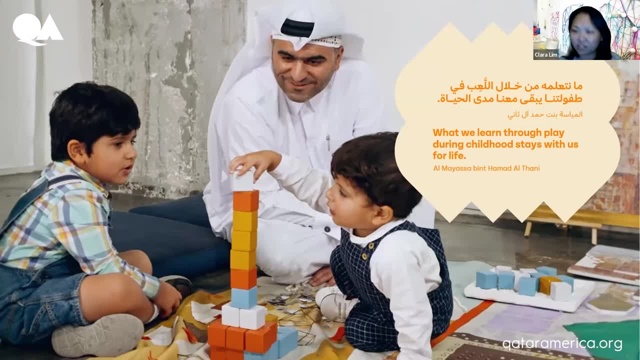 Shekhar Mayasa, our chairperson of Qatar Museums, says: you know what we learn through childhood. what we learn through play during childhood actually stays with us for life, And we firmly believe this. We believe that play is the way that children unpack, you know, experiences. 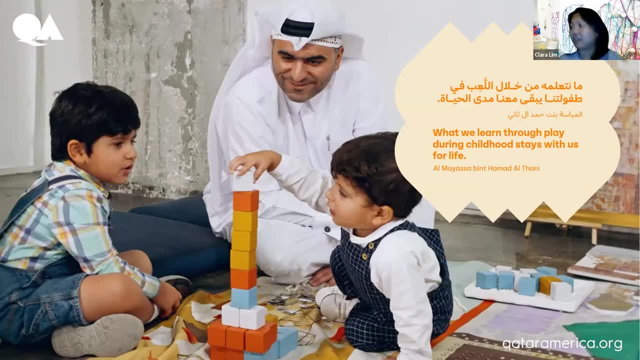 It's the way they express what they know, It's the way they experiment to find their boundaries And it's the way they will test relationships. So where does this take us? Our galleries, which we have been designed to be extremely playful. 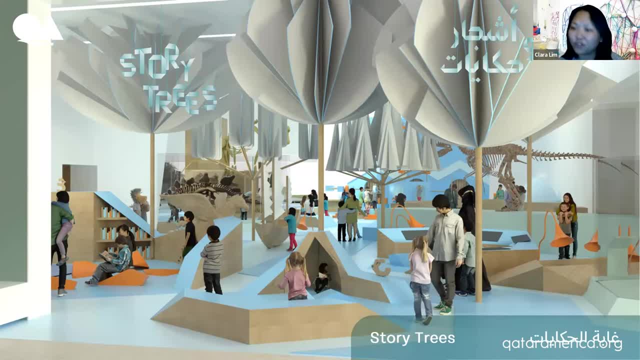 Now, Hannah said that you're one of the few collecting children's museums. We are not a collecting children's museum, So we have a null acquisitions policy, But we have an immense collection throughout Qatar Museums which we can draw on. 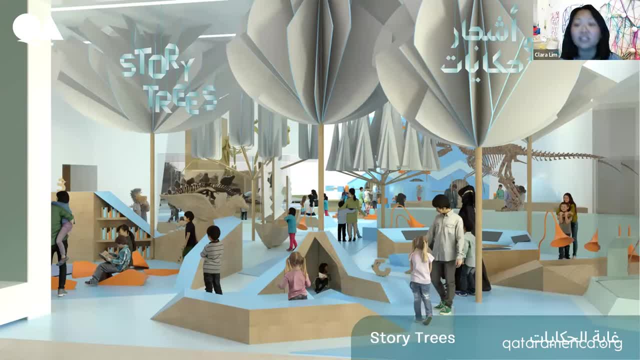 And this is what we want to do. So you'll see dinosaur fossils in the background, And we are, you know, using fossils from the natural history collection, But instead of interpreting them- and this is where the design and interpretation come from. 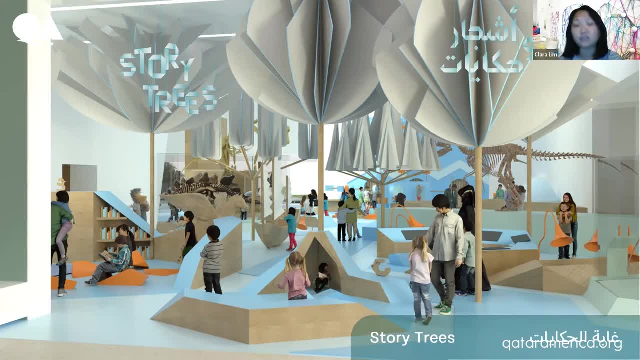 Instead of interpreting them by saying: okay, you know, in a natural history museum you talk about the name of this dinosaur. Which period did it live in? What did it eat? Who did it live with? What were its nearest, you know, living kind of relatives? 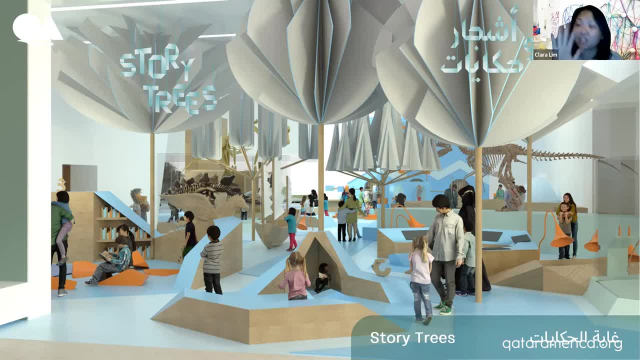 But we will have that information. But the information is foundational and it's basic. What we want to do is to link them to the other experiences. So in this gallery we're looking at just one of the exhibits- story trees- Where we want to give children the opportunity to have literacy-rich moments. 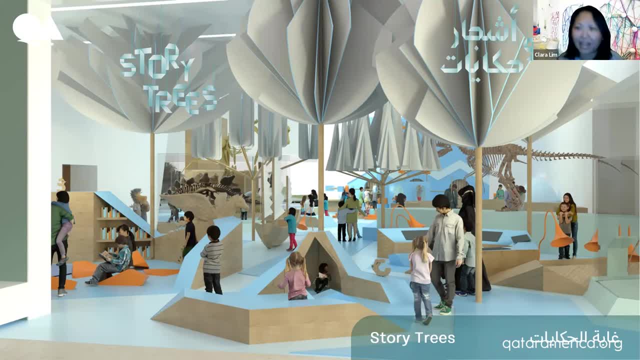 These might be reading books. This might be expressing themselves, putting on a costume and acting out a play. It might be sitting down at one of the scribble boards and creating their own storyboards, But we have a dinosaur there to encourage them to tell the story of the dinosaur. 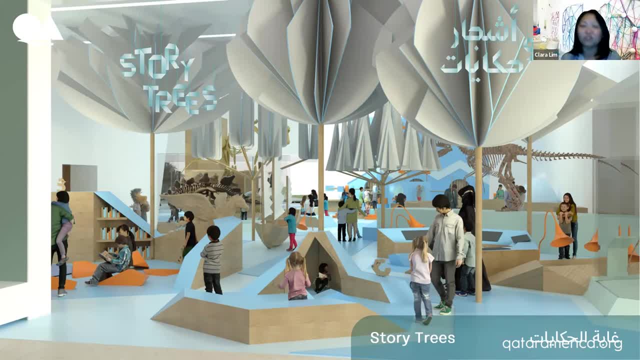 To act like a dinosaur To make up, To use this to create whatever story they may have to tell. On the right-hand side you see the myosaur that sits within the earliest area, And the myosaur is known as good mother lizard or good omelet eater. 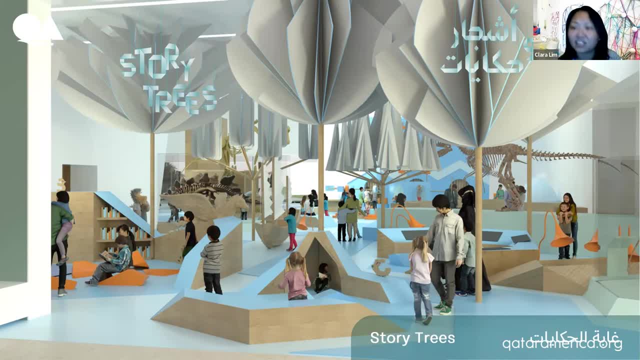 Scientists don't really know, But this dinosaur has always been found near nests of eggs And in this case, in this exhibit, we bring in the idea of stories and communication as well. So there's going to be a little interactive where you can say you can record something that you see. 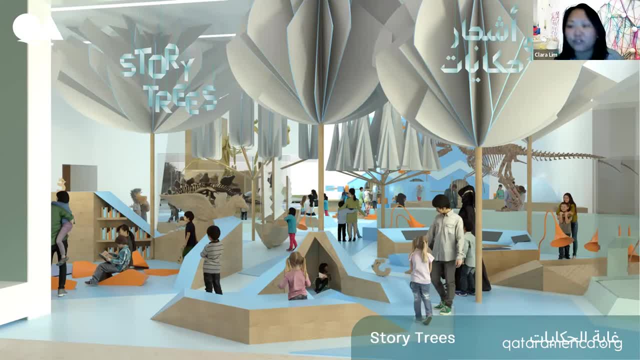 You might record to say hello, little one. And you can change the frequency, You can change the amplitude, You can affect the squash, You can put it through different kind of sound systems to distort it And you can make it sound really panicked. 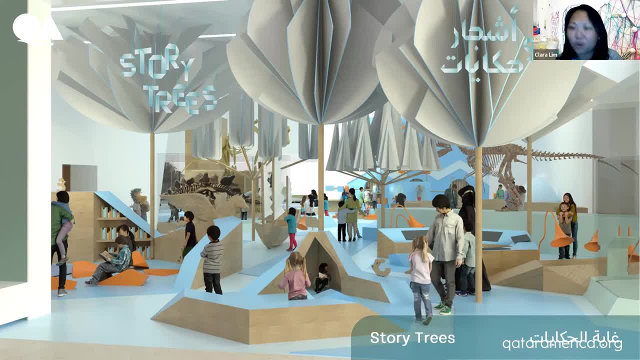 So that's, how do children think mothers who are warning of danger sound? How do mothers speak when they're trying to calm down the child? So these are the ways they can then express what they know about the world, But also what they think. 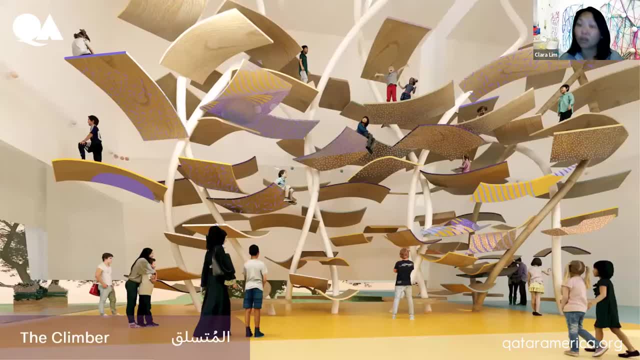 What are their ideas? We also are looking at physical activity. We have a big climber indoors. Before anyone panics and thinks about suing- because I know we have quite a few American audiences here- There is a safety net around the whole climber. 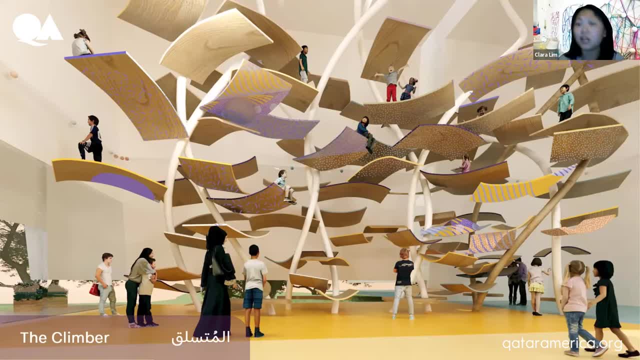 We just didn't put it in the renders because it just looks prettier. But in this instance, you know, having physical play indoors is extremely crucial. in Qatar Today it's 50 degrees outside. We've got dust storms for the last three days. 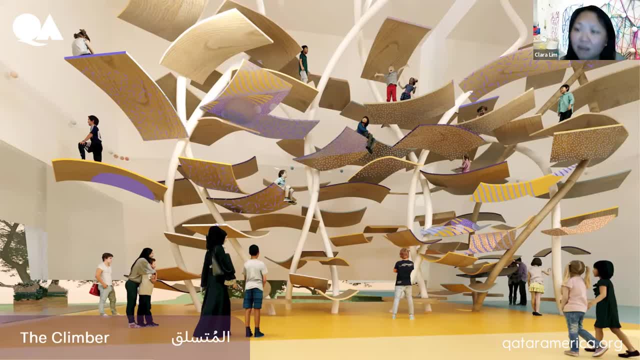 Ministry of Public Health has said: don't spend time outside. You can spend any time outdoors, as much as you can, So we need to have these opportunities indoors, Which is why we dedicate a big amount of space for this. Those of you who are familiar with this, this is the Lucky Climber. 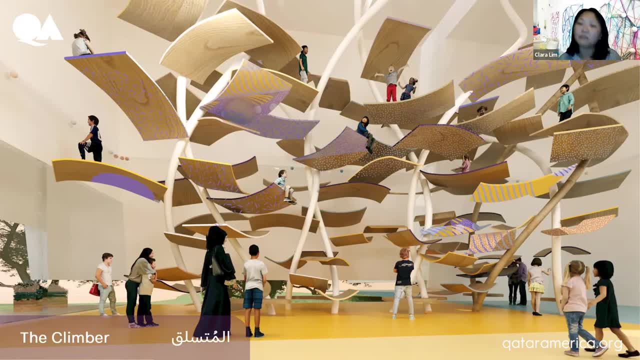 And the design of such a climber is that the leaves, the climbers on the lower level are actually closer together. Which means if you're a younger child, you have less confidence, less physical ability. you can climb up to a certain height. 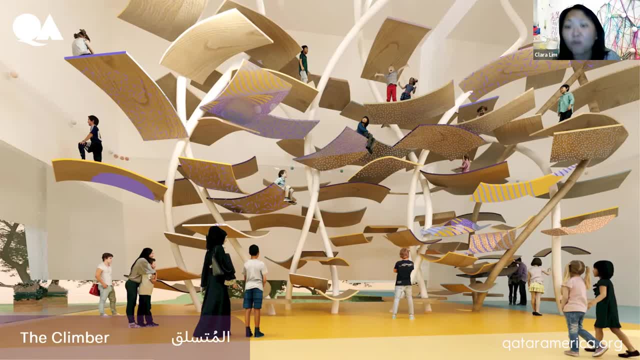 It starts to get wider, It starts to get harder. It needs more risk taking after a certain level And if you're a young child And if you don't feel that you're there, it's fine. Your body gets the message. 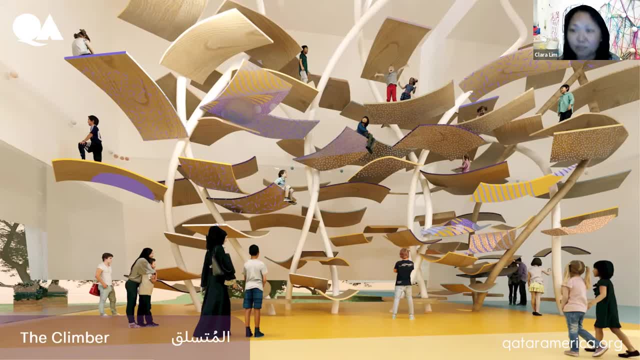 It's a visceral reaction. You can choose to come down at any time and explore a different path, And this is one of the ways we know that children will come back again and again. They're going to come back at age 2.. They're going to come back at age 5.. 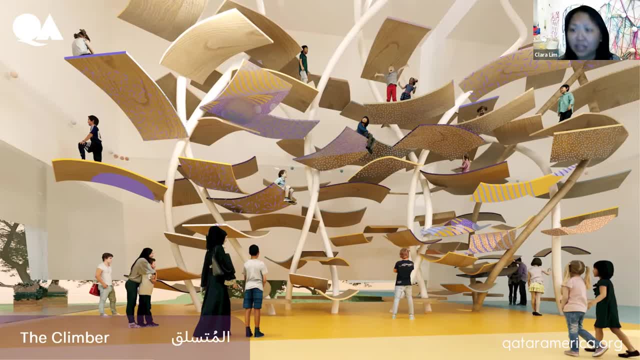 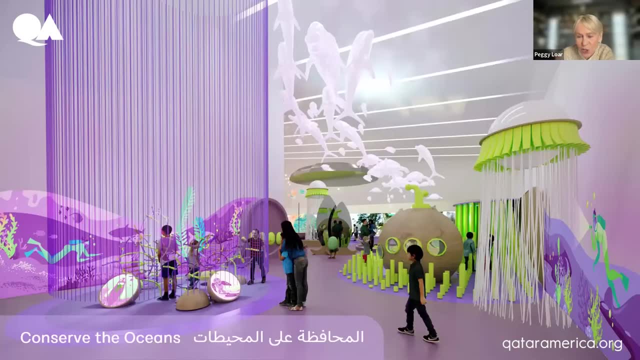 And they're going to come back at age 10. Because even the exhibit looks the same. it's going to be a different challenge for them. Clara, thank you so much. I'm afraid we're going to have to move on to our next presentation. 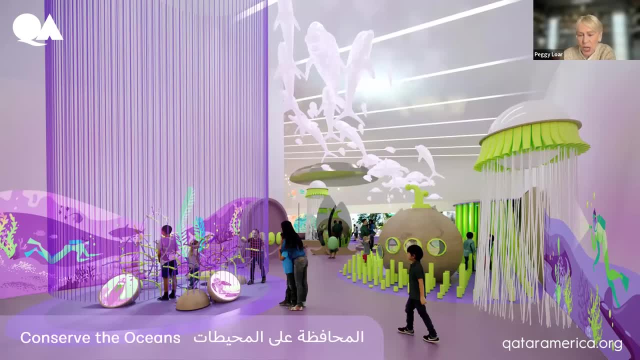 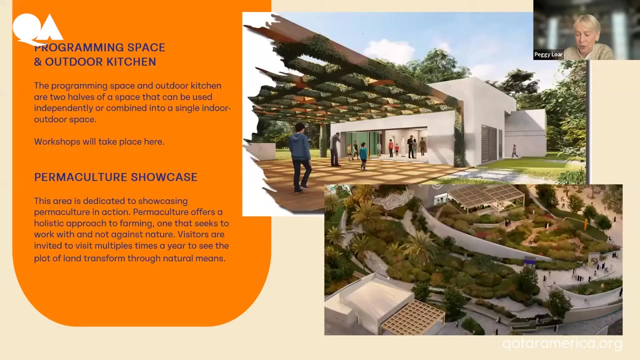 Maybe we can capture some of the other things in your comments afterwards. I want to give Sheikha Nosra an opportunity to present, But I am pleased that you covered so thoroughly the emotional and social support that children's museums and this kind of education provides, so that we have what we call good future members of society. 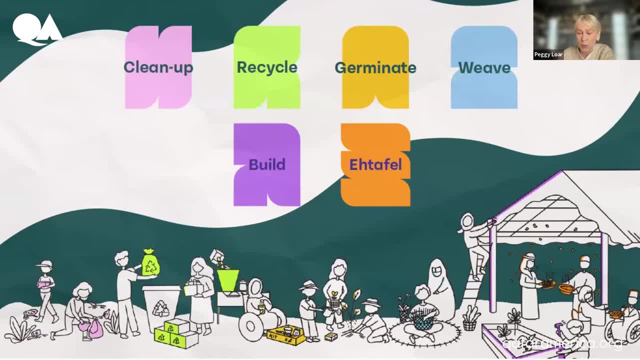 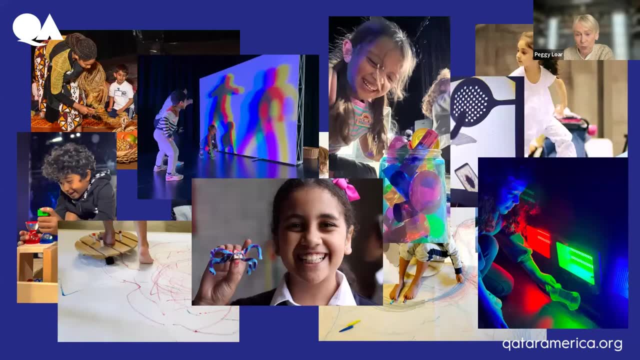 So hopefully we can touch on that. I'm particularly interested in what they're going to be doing with nature and the planet and the creatures that may not all be around when these children grow into adults. So let me move on to our third speaker. 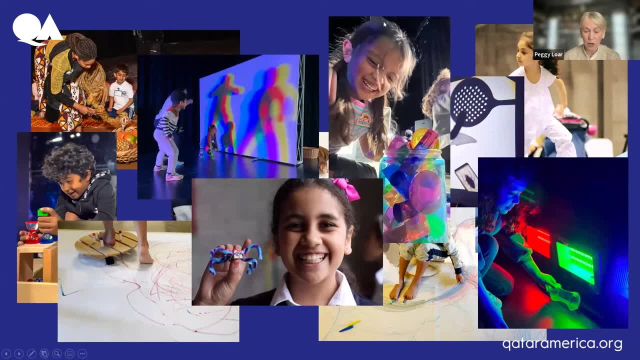 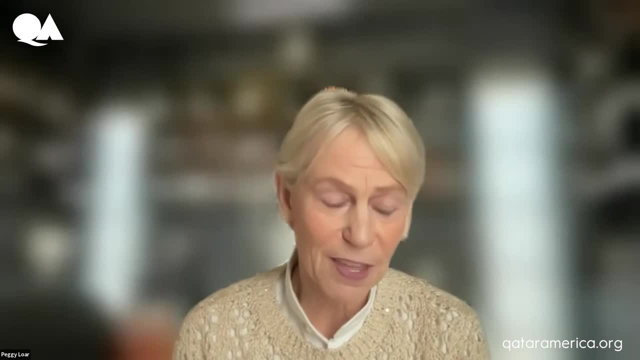 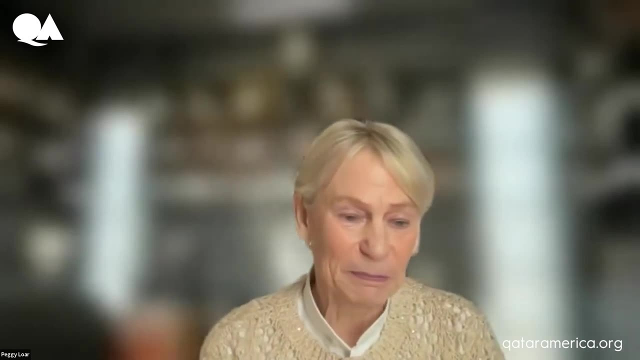 Sheikha Nosra of the Museum of Islamic Art in Doha. You have a special challenge. You have what I consider very sophisticated collections And you have to make them relevant for children. So, please, we look forward to your presentation. I think you're on mute. 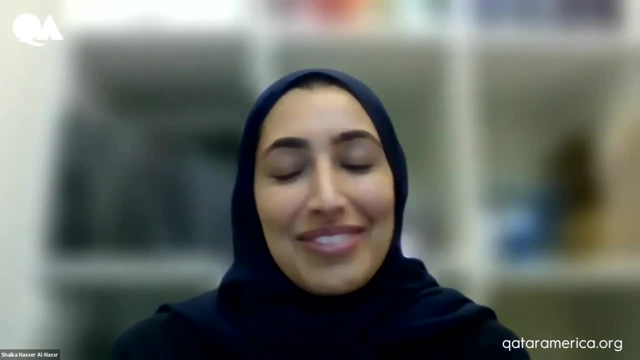 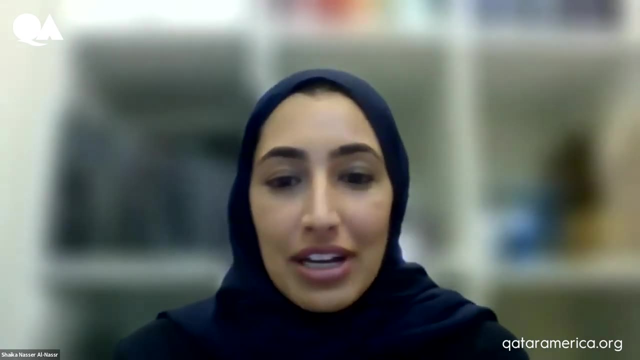 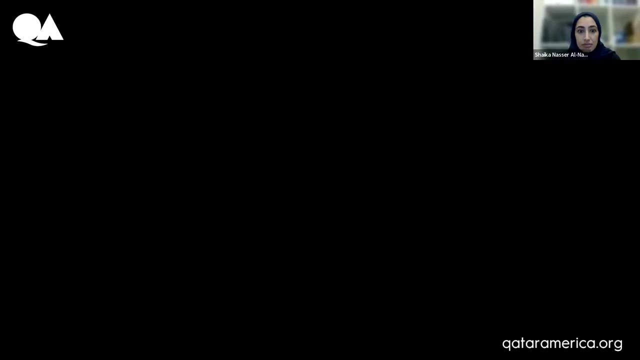 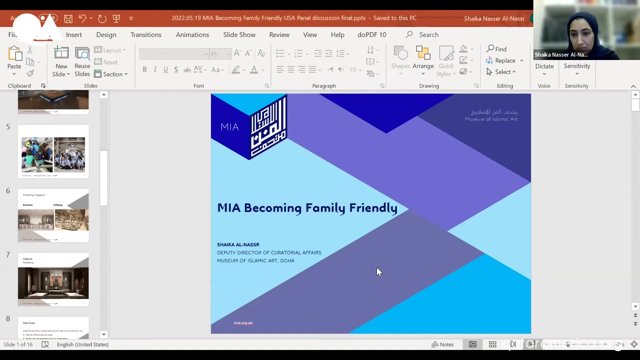 If you can hear me. Yes, okay, Thank you very much, Peggy, And good morning. Good morning to those of you in the United States And good evening to everyone in Doha, So let me start by sharing my presentation. Okay, 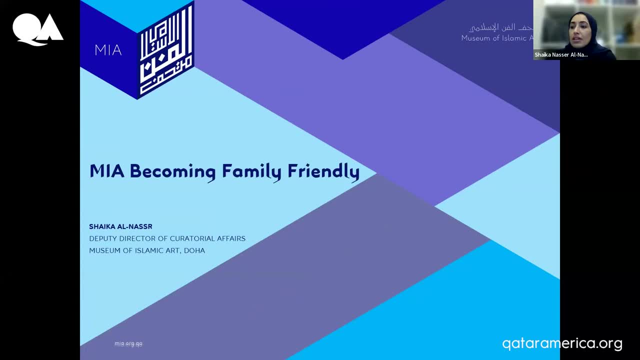 So It is my pleasure to be talking to you today About how the Museum of Islamic Art is becoming a family-friendly museum, Which is a key part of the major renovation project that is currently under construction And will be delivered in fall this year. 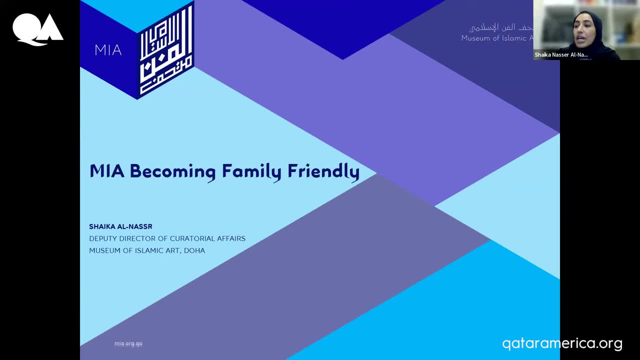 Just before the World Cup. I'll start by giving a brief background about Mia's main reasons for going under the relaunch, Keeping focus on families. Then I'll talk about our main aims of the project And after that I'll highlight the strategies we are applying to enhance the family experience. 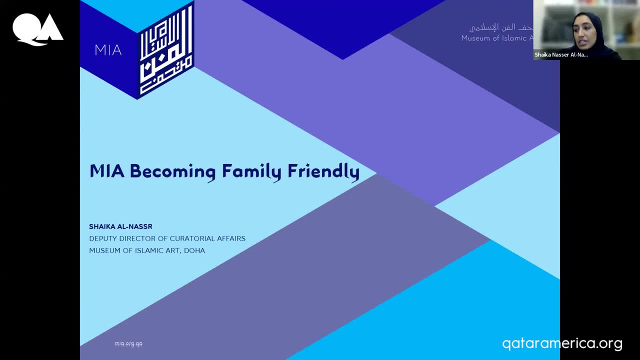 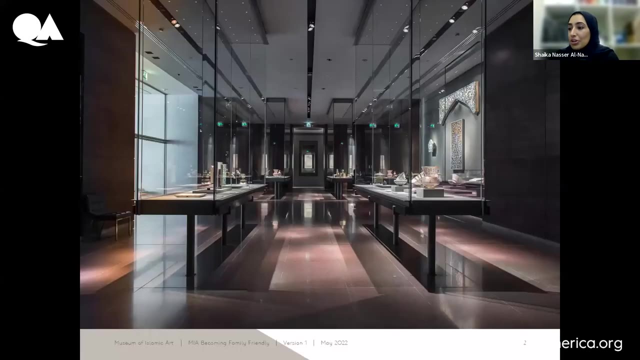 From the moment they enter the museum, starting with the facilities, then focusing on galleries, And finally, I'll talk about our plans to engage families through programming and reutilizing some of the areas on our site. I'd like to start with sharing an image of the museum galleries. 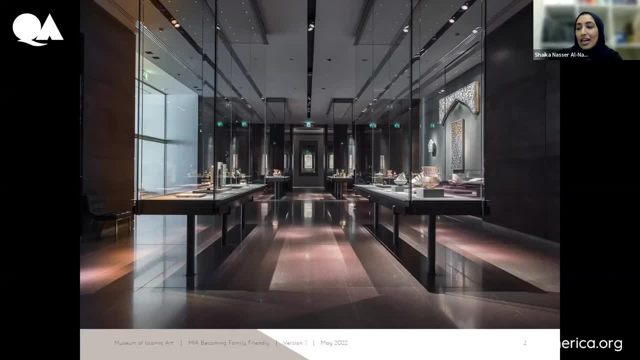 In case you haven't been or seen them before, And I'd like to ask you a question: How would you feel if you are visiting the museum with children aged 7 or 12?? Take a moment to look at these images And you can write to me in the chat box. how would you how the experience will be? 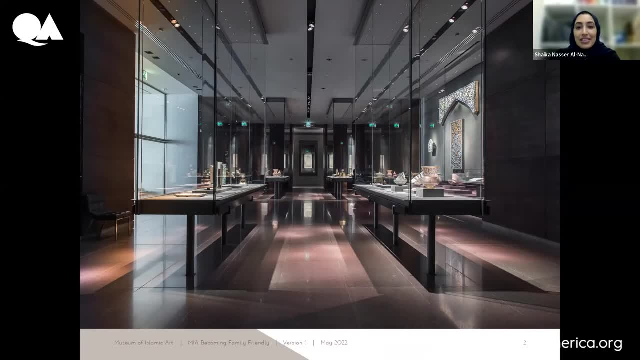 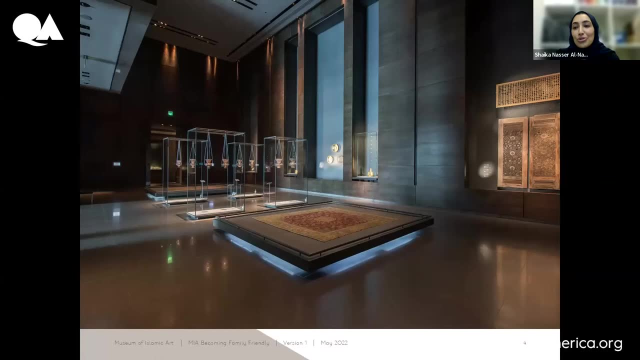 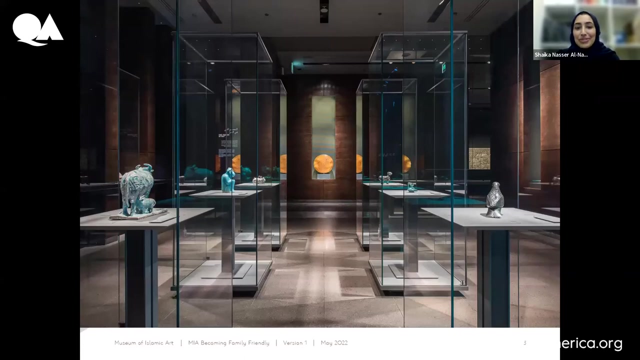 So I have a few images here. Okay, I can tell you one thing immediately: That they are so beautifully designed. There is no doubt about that, But how would you feel if you are with kids? So it is So our, our gallery maybe. 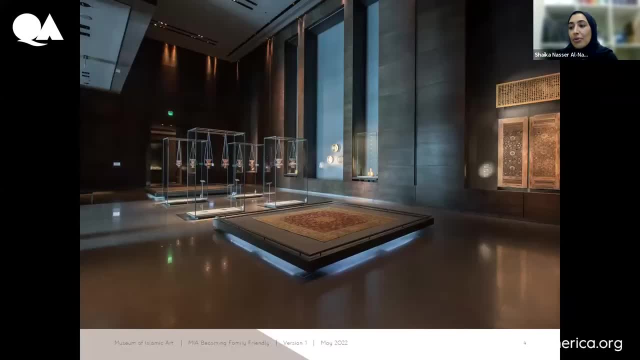 I can. I can say that Our galleries are designed in a theatrical approach, With the objects surrounding are being quite dark, And but here it's in the morning, That's there There is light, But at the evening that it's a quiet, dark galleries. 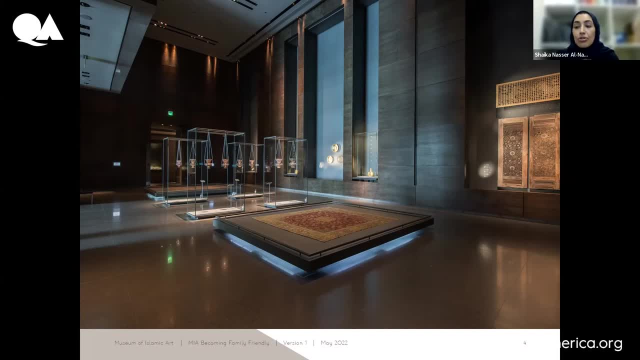 With the providing minimum information. So the beauty of the objects will speak for itself. So this was the approach of the designer. The content provided and then the labels is minimal, very limited. It's only tombstone information with the date, country and materials. 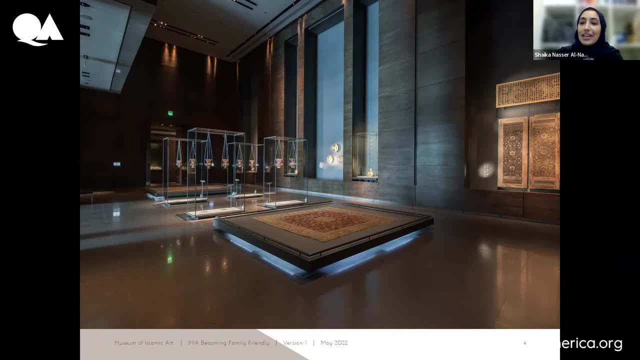 So after the opening, we began to notice some engagement issues, especially with family visitors, who are one of our main visitor groups in the first place, comparing to others. So we decided to conduct evaluations, Using different methodologies And with the assistance of international companies. 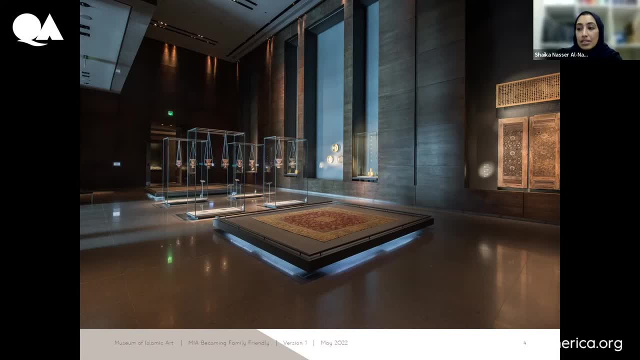 Specialized in understanding museums And improving the visitor experience. The results showed that the visitors have a fleeting level of engagement In some areas And they learn very little about Islamic art, history and culture, And some finish their engagement with an object Without knowing its significance. 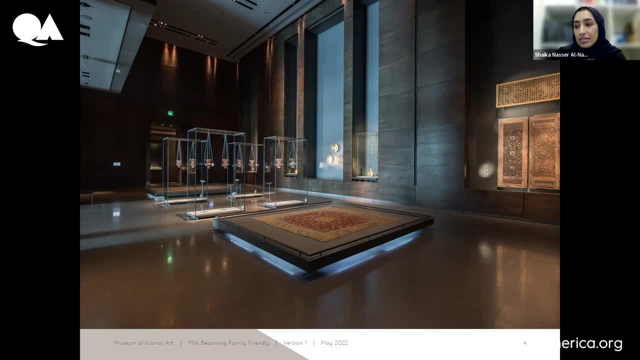 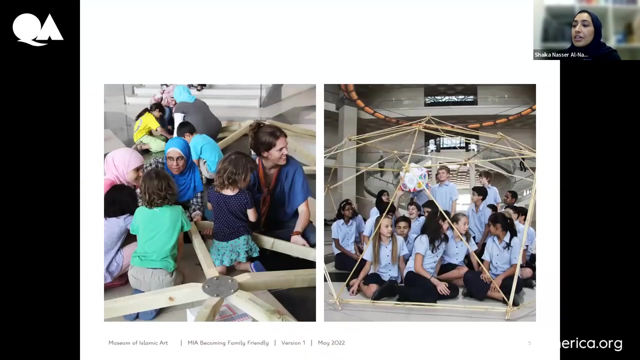 How or for who it's made. To the extent Some of them felt quite frustrated With a lack of information, Especially with families. They found that the museum visits were quite passive. Children and younger audience are core audience segment for us And they were not catered for in our permanent galleries. 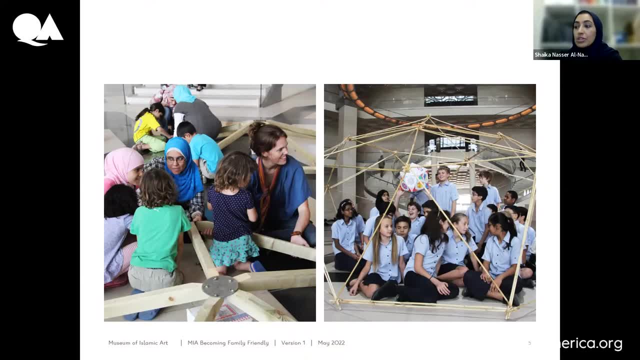 And we were compensating for this lack through our exhibitions and program Programs. But galleries remained an issue. After further studies and consultations for around five years, We've decided to embark on the renovation project To improve the museum facilities, Security, Access. 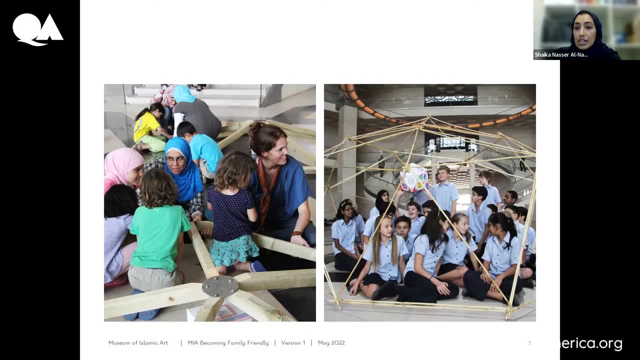 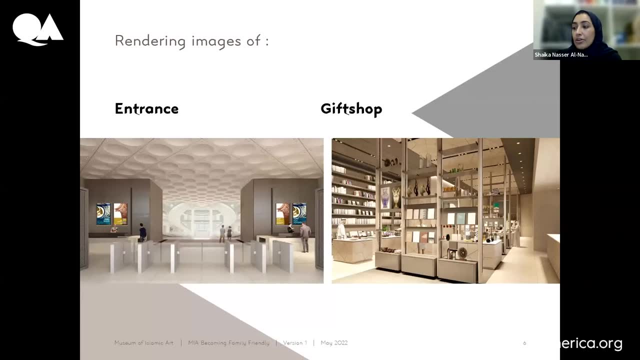 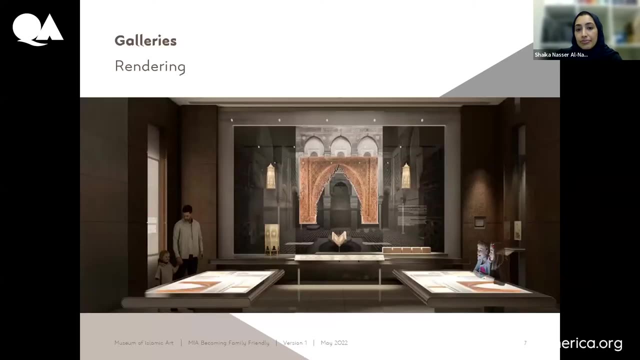 Improving the way, finding signage And utilizing areas that were not used before. Most importantly, Enhance the visitor experience inside the galleries By creating innovative solutions to attract families. Some of our main goals for families are To create a holistic, family friendly experience. 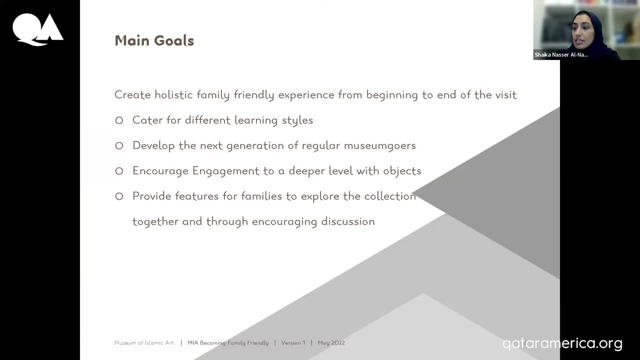 From the moment they enter the museum, with the facilities Such as the decaying breastfeeding and changing rooms. Providing suitable means. Selection for families in the cafe And inside the galleries that I'll talk about In more details. Cater for different learning styles. 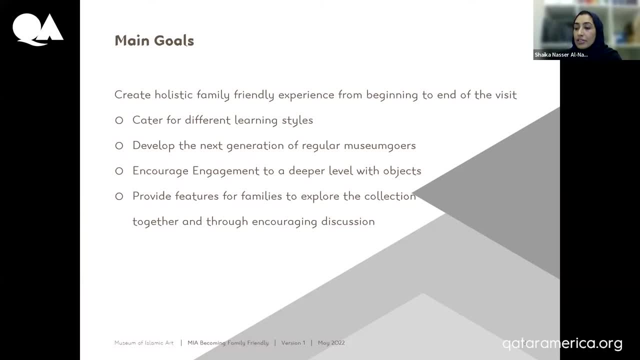 By incorporating a wide variety of learning methodologies Such as videos, Sound, Fragrance And tactile experiences, Develop the next generation of regular museum goers By creating memorable experiences, Encouraging engagement to a deeper level With objects related to personal experiences. 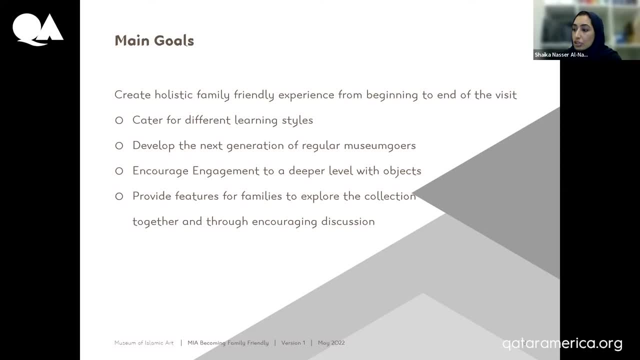 And, finally, Provide features for families To explore the collection together And through encouraging discussion. The museum experts have found that family visits Send messages to children that museums are important Part of life experience. So the strategies or the approaches that we have applied- 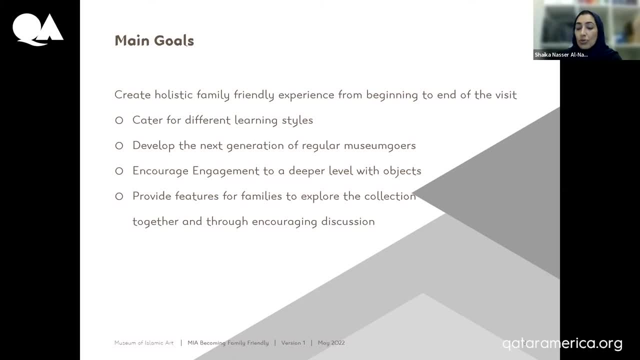 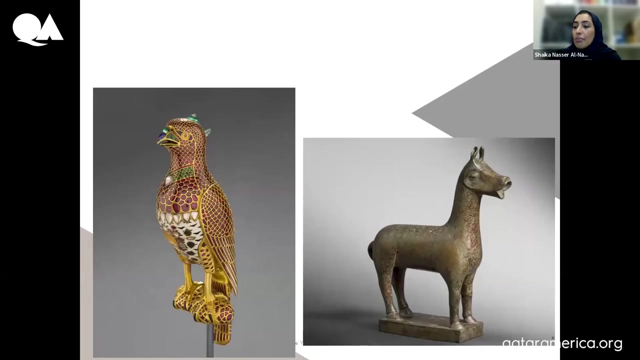 To meet these main goals are: We created a family trail To guide the families through the galleries, And And it included Three key elements. We came up with the idea of creating family character, Family characters from our collection, Such as the Falcon or the hint, which is the 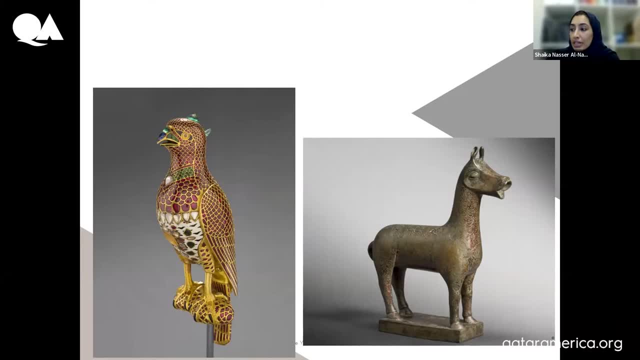 The female deer Illustrated in a distinct way For families to recognize, Recognize and guide them through their Their visits. And these characters will appeal In a special family label That will encourage reflection And discussion with some of the objects. 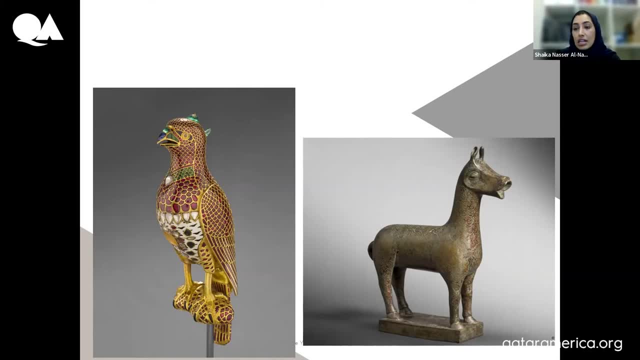 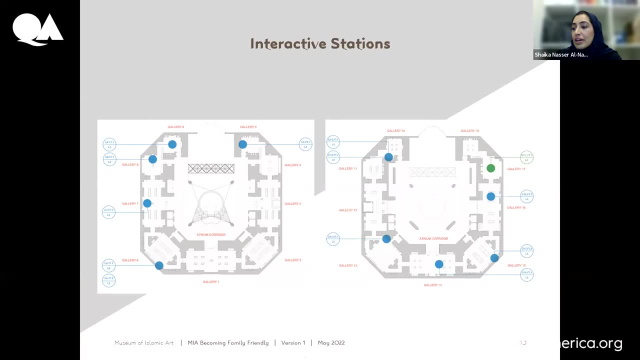 The content On the label will be written in a child level That is easy to read or to be read And understood. We all know that children will not read all the labels, So we have alternative Solution, And that is to create 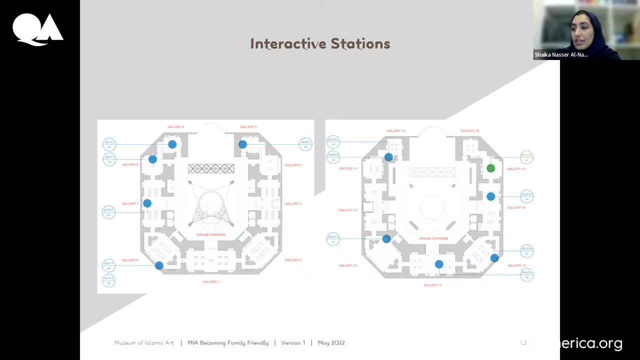 11 interactive Stations across the Across the galleries For families to learn About various themes related to Islamic arts, And the dots highlighted here on the In the slides are where the Interactive stations Will be implemented. It was quite challenging for us because the museum of Islamic art is 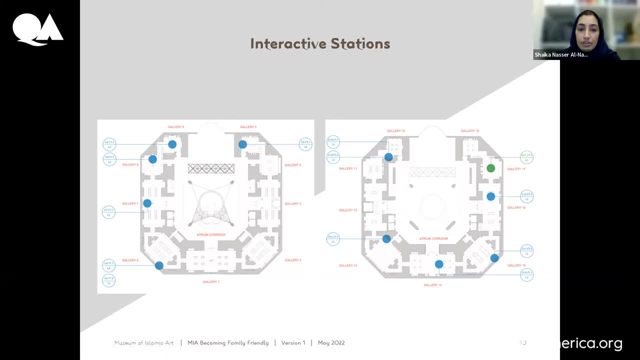 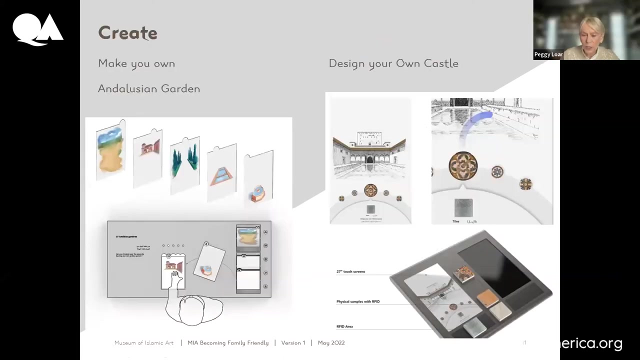 Not designed For for this station. So we had to find the places to This station And we have categorized them into four main Approaches. The first one is to create Jacob. We have some, Some feedback coming. I'm not sure if it's from your computer or someone else's. 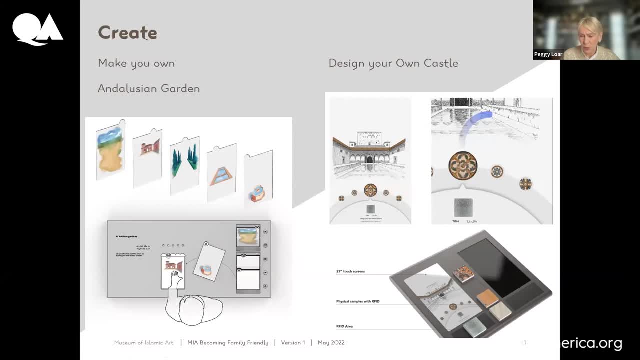 It's only when you're speaking, Do you? is there any button that's turned on that Could be turned off? I don't know, but now we have the call to prayer. Oh, maybe that's it All right, Okay, please. 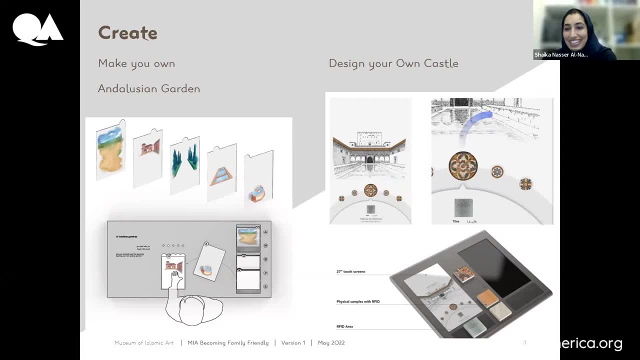 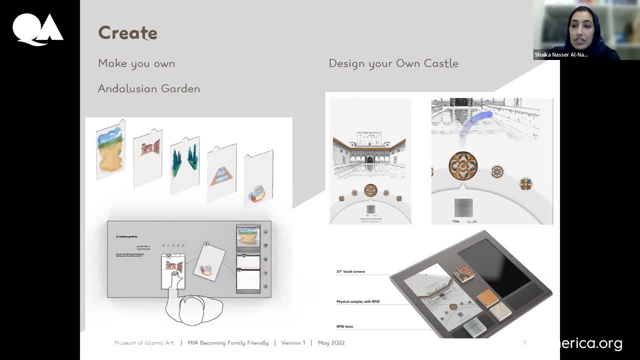 So we have to- maybe I speak louder- Using using imagination And when they're creating processes and activities such as Create your own Palace, Where children can select patterns, Design and material to create 15th century, And then 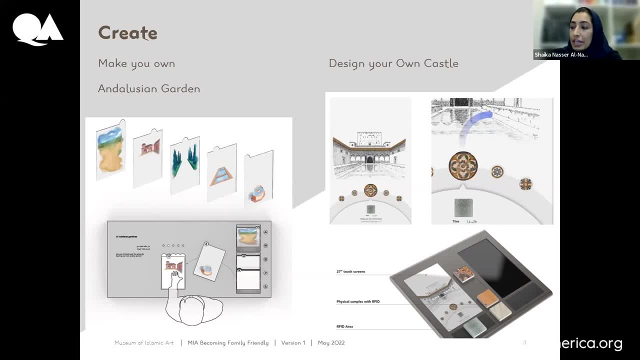 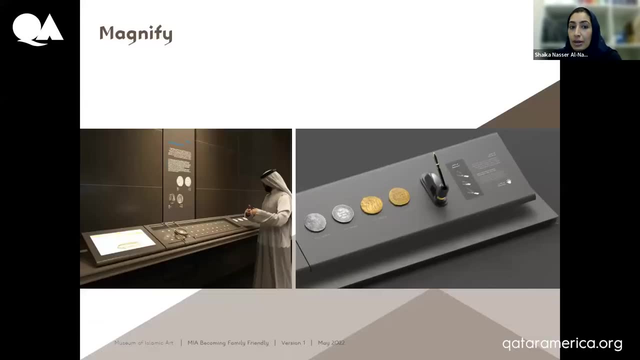 Families own garden by underlying the underlying the garden features to come up with the Alhambra garden. And then we have a magnify to encourage a close looking as in coin, a coin experience, to explore all the details and have even the opportunity to mint your own coin. 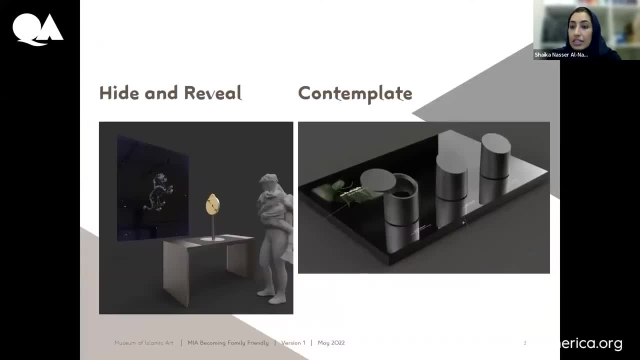 And then we have a hide and reveal to learn about astronomy navigation and use the Astrolab by directing a replica at the star map And then, once you point at the star correctly, a constellation will appear. Then we have finally to contemplate with the smell stations. 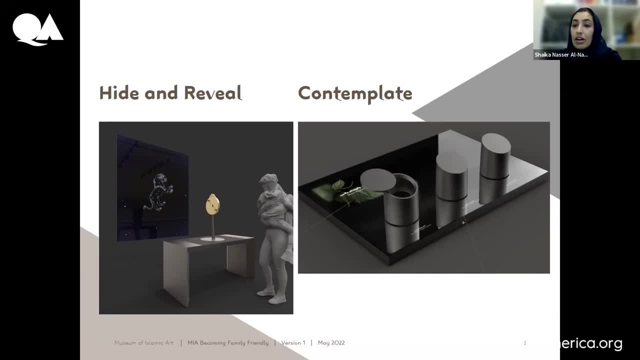 where visitor can, where visitor are asked to guess the smell, then the name of the spice will appear with the information that explain about the smell. And then we have the trading routes. and all These are just some selection of the family interactive stations, but we have more. 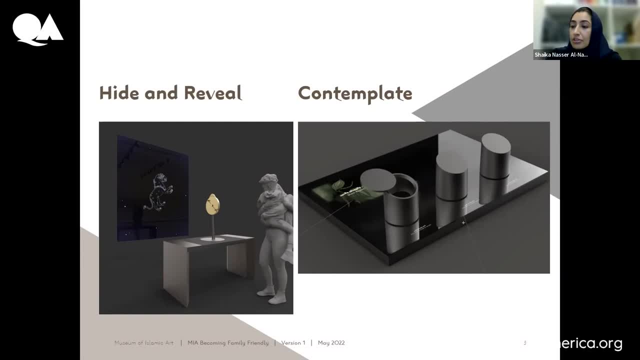 And then we have. we have developed a crook steps where we, where would? they will be placed across the museum to allow children to get the closer to the objects, objects and get a better engagement with them. These approaches will provide many level of engagement. 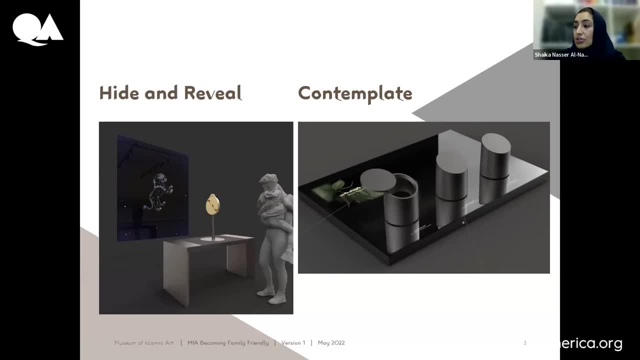 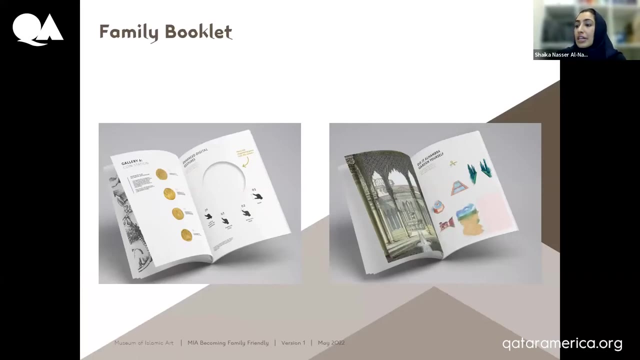 And give variety. that will allow activities to be used many times, each time experiencing a different outcome and encouraging repeated visits. The family trail will be supported by an additional booklet for visitors, as they can either use it during their visits or after. Outside of the main galleries, we have repurposed one of the rooms. 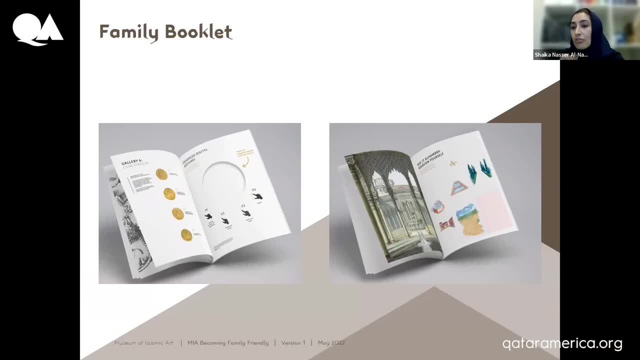 of the main galleries. we have repurposed one of the rooms on the fourth floor of the museum that haven't been used since the museum was open to create a multi-purpose workshop space to be used for children and teens. Being so close to the galleries, we allow us to extend learning spaces. 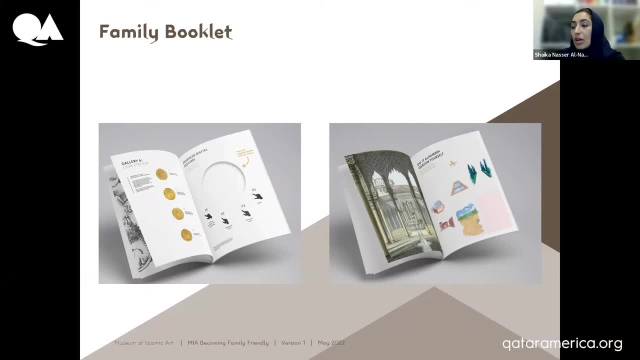 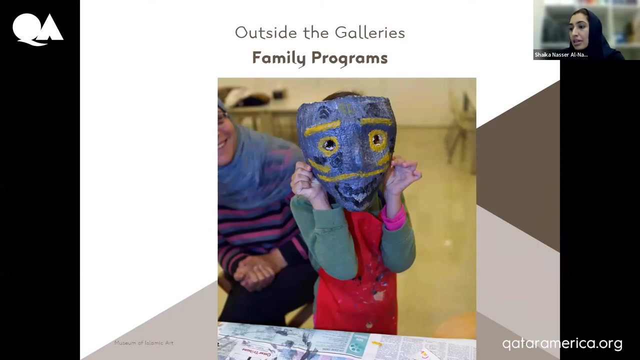 over several floors, giving incredible flexibility to our programs. We will also offer a long-term teen programs to encourage those who want to work on a broader field, as well as a space for them to meet and create their own activities. With the relaunch of the museum, we have taken the opportunity. 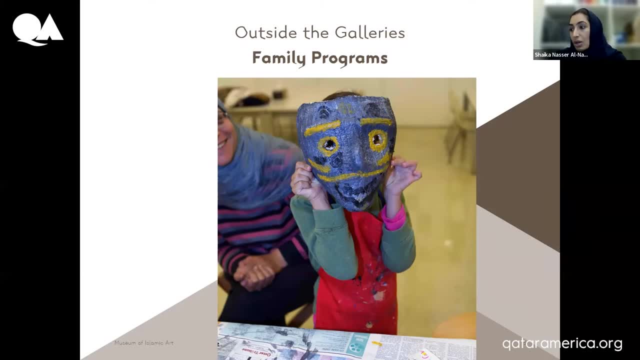 to create a new trail, and family activities, which put the whole family experience at the center of the program, as well as the family trail interactive, where we offer a family kids to enjoy the gallery. In addition, we also offer a variety of activities. 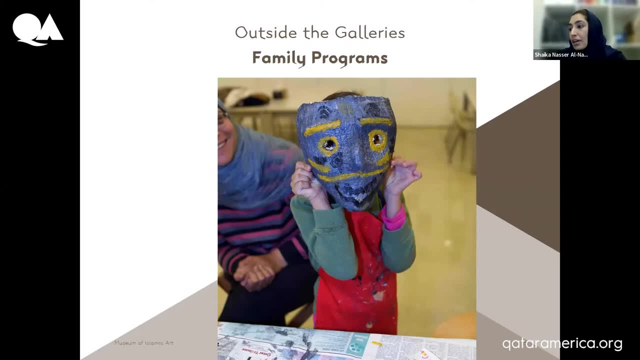 for children and teens, such as art galleries and art galleries in a non-technical way, such as the ice pie bag or the chatterboxes. There are not focused just on children, but on families enjoying themselves together. We also extend to our online offer with a jigsaw games. 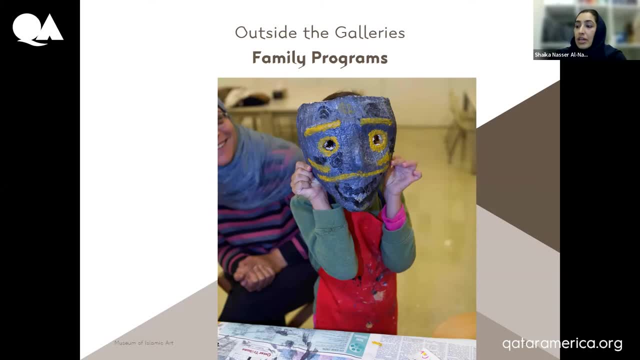 and family suggestions for post-visit activities. To conclude, children are our next generation of a museum and if they visit the museum with their parents, the experience will be a more memorable part of their lives. Families and children are one of the main audience segments. 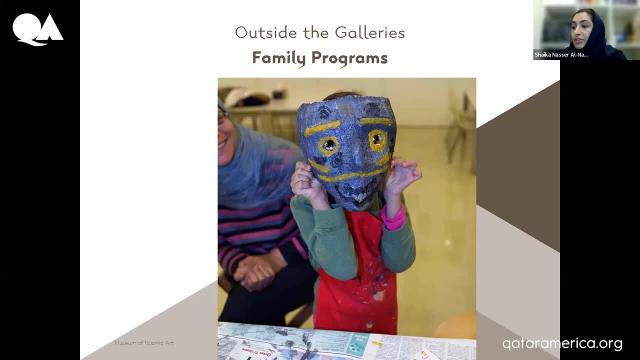 so it is our own role to provide different platforms, through programming, exhibition and in the galleries, for them to learn, engage, explore, to be inspired by Islamic art, history and culture. Thank you, Thank you so much. I want to ask you a quick question before we move on to all of our questions. 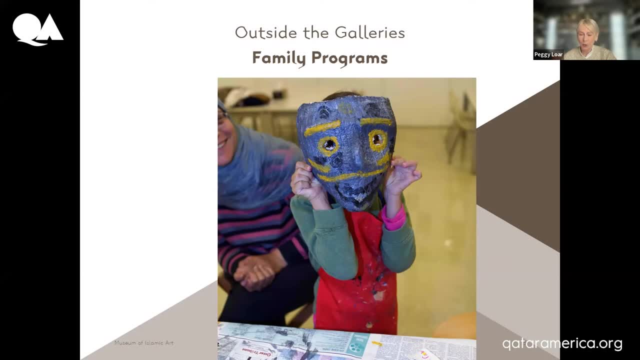 for everyone. Your title is Deputy Director of Curatorial Affairs. In the early days, probably before you were born, educators didn't talk to curators and curators didn't talk to educators. The curators now are very pro-education, it seems. 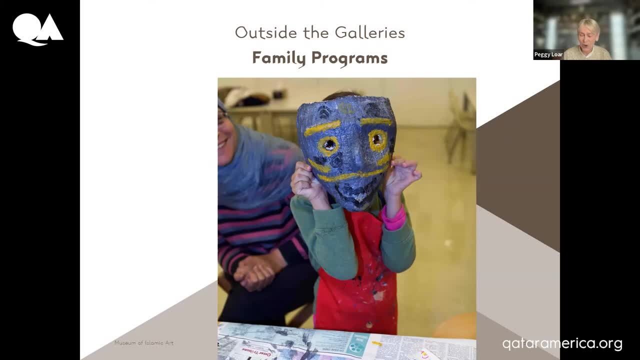 and educators are very interested in collections and research. So do you encompass education and collections in your role? Do both of those departments? Do both of those departments function with you? No, We have. so the museum. we have three divisions: Curatorial Affairs and Learning and Outreach. 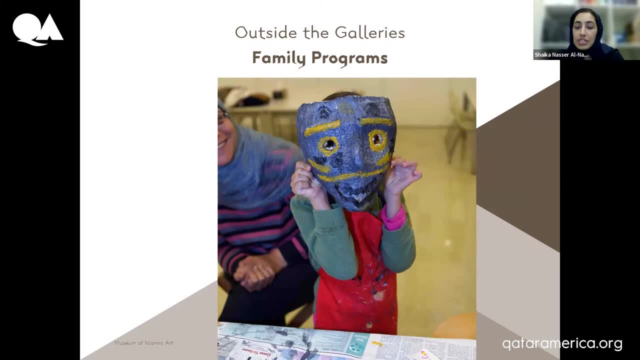 where they have the education department. But for this project, especially the relaunch, we work together and collaborate so much, especially for families and program where we become. we work very closely with the curators and the education team. So it's very important. 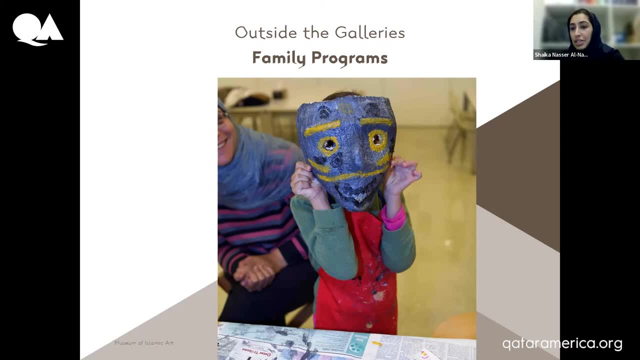 It's not. we are not, even though they are separate departments, but we are like one team, one project team, where they are involved in every stage of developing, especially the family trail. There are some, you know, curators have different approaches and point of views and learning. 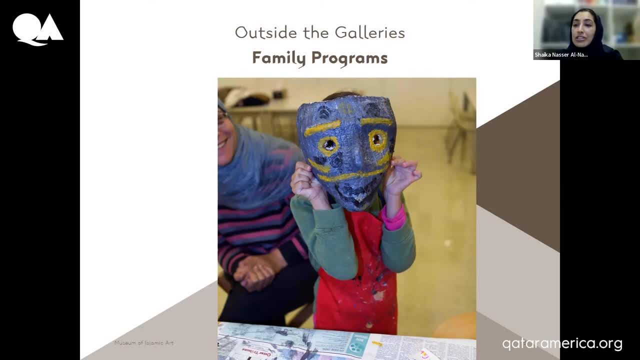 They have different, but we always focus that. the audiences and families are our main focus and we do what is best For them, And we have to compromise with some of the teams to make sure that we meet with our main goals. Well, carry on. 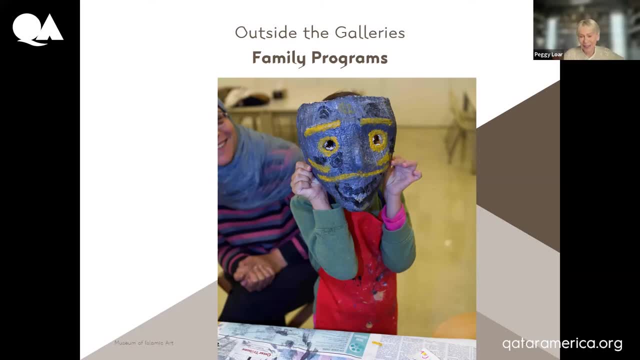 So far, so good, And it's so great to see the MIA interested in these programs and especially in those smaller interactive galleries that you're establishing around the museum. The first question from the audience, Hannah, I'm going to direct to you. 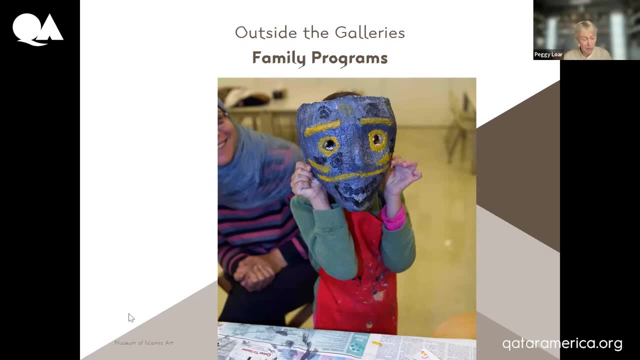 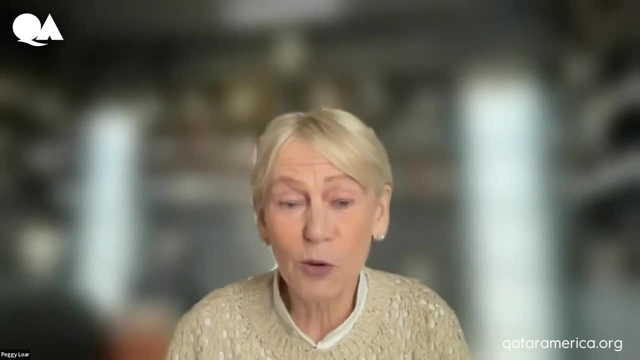 It's a very simple question, but it may be more complicated. Maybe it's more appropriate for us, Maybe it's more appropriate for a parent to answer it than for a museum professional. I'm not sure who of you are both, But is there a point in time when a child says: 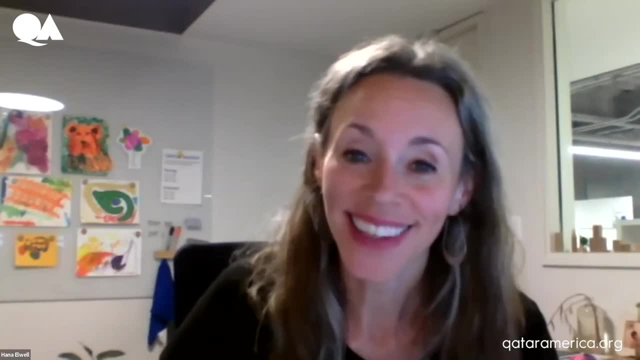 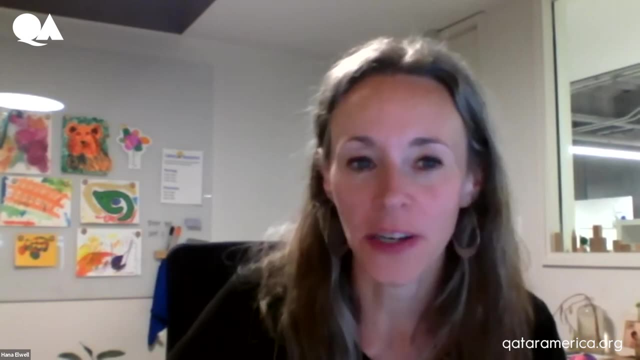 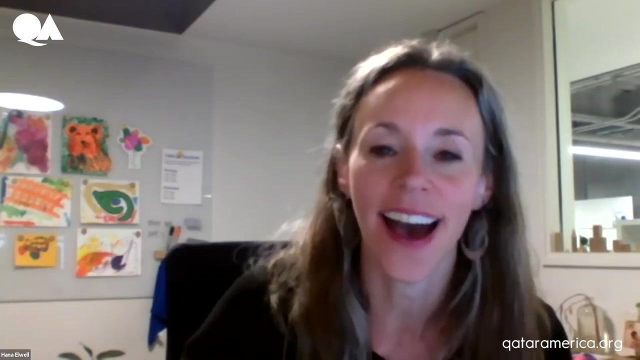 I'm too old for a children's museum. Well, sadly, that is a reality of this business. I recently attended the Association of Children's Museums Conference, their annual conference, And that is always a topic of conversation: how to extend the relationship with families of kids of early. 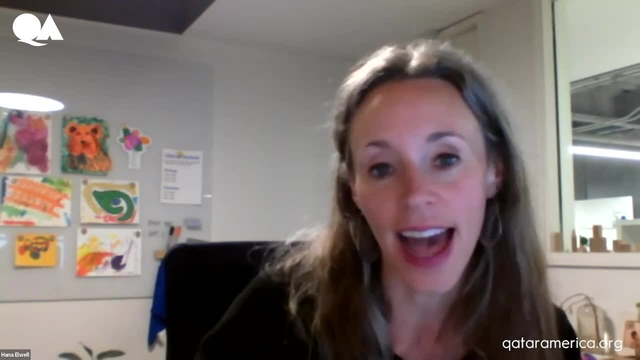 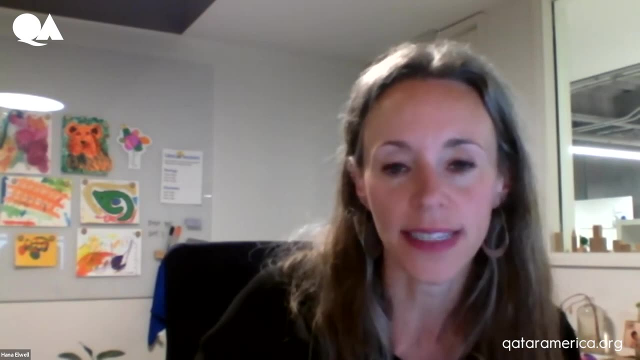 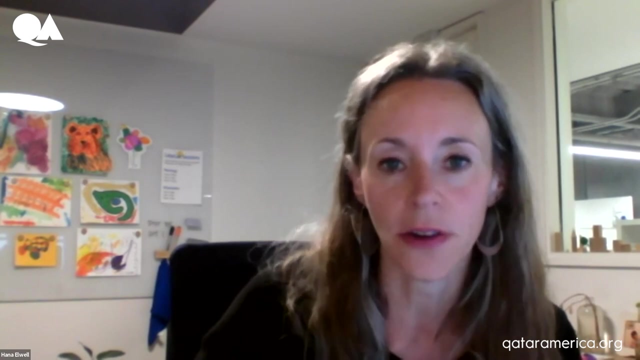 to the institution And there's some ways that we really have intentionally scaled up our exhibit development to reach a slightly older audience. Our new exhibits we're thinking as 5 to 10 as our target age, whereas historically we've defined early childhood as 0 to 8, with really 2 to 6. 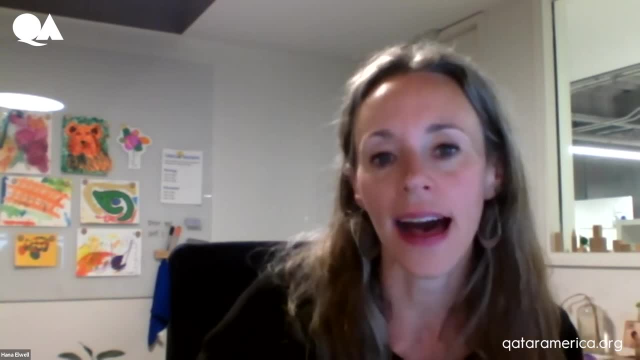 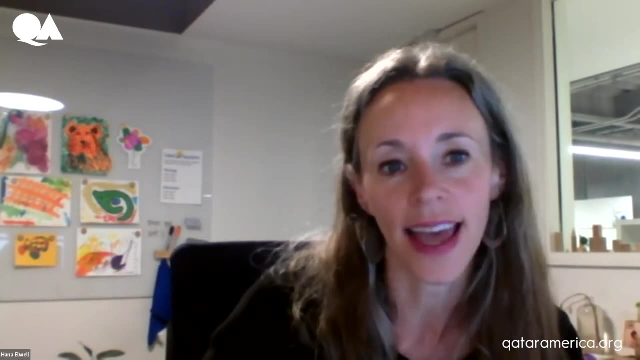 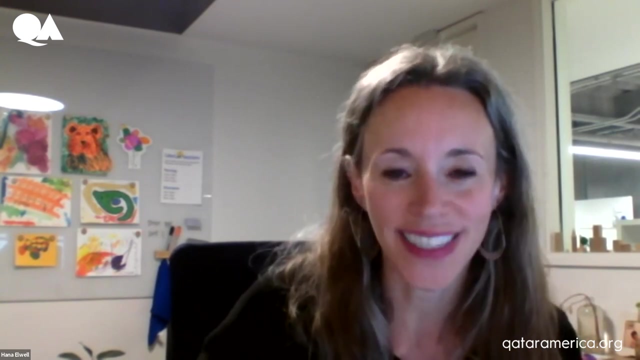 as our sweet spot. So I think that programming permanent exhibit development and then programming as a layer on top of that can extend the- you know, the age range of exhibits. We also have a teen program, So we engage high school age students. 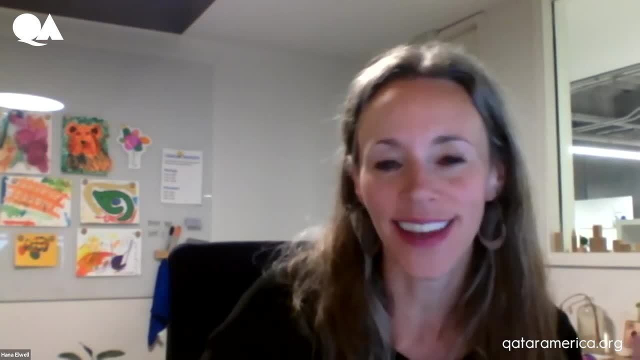 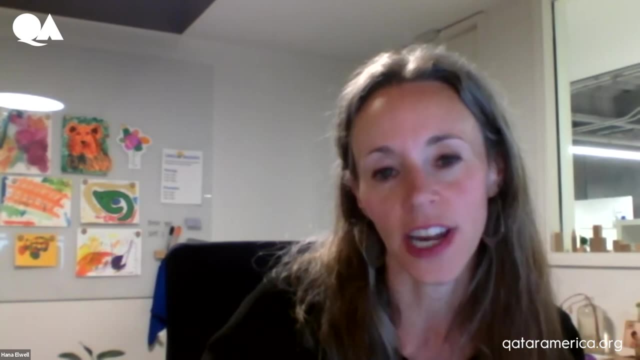 And even though sometimes they have a reaction to: oh, this place, I came here as a kid, It's not for me anymore. Our collection really is a point of great engagement for high school age students, who can also, you know, having their presence in the museum. 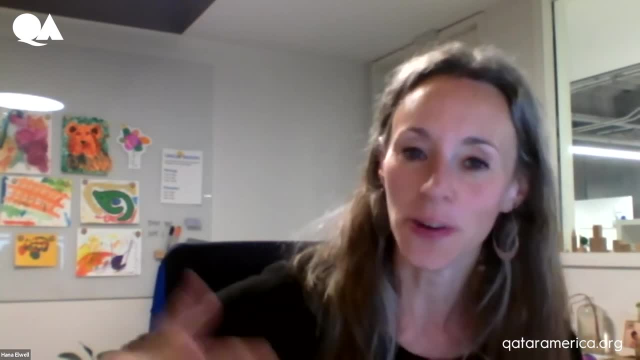 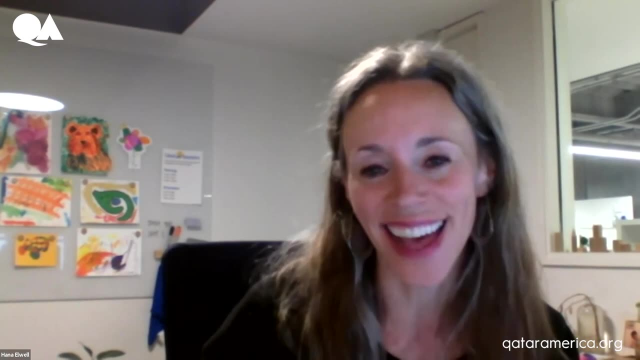 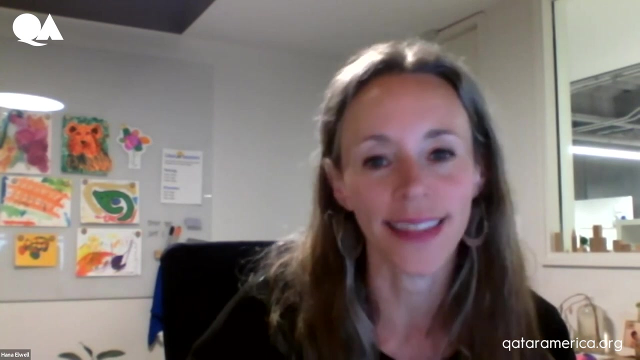 to serve as mentors and for younger kids to see older kids and sort of chart their own milestone path ahead. I think is a very positive thing, But the reality is that our core audience does change out over time in a more dynamic way than other kinds of museums. 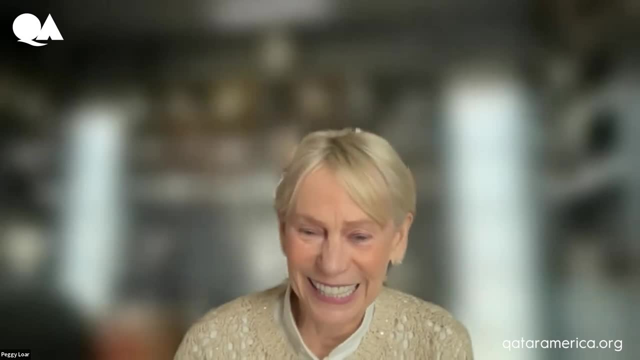 Well, thank you for that. I'm not surprised. That's good. This question is for anyone who wants to answer it. There are those in the audience who want to know how you would advise them to pursue a career in a children's museum. 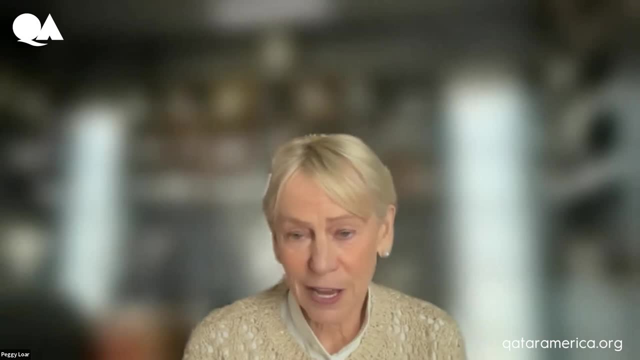 or working in programs with children. Should it be child psychology? Should it be museology? Should it be science? if they want to go into a science center, What would you advise? Anyone want to take that question? Well, I'm happy to take the first question. 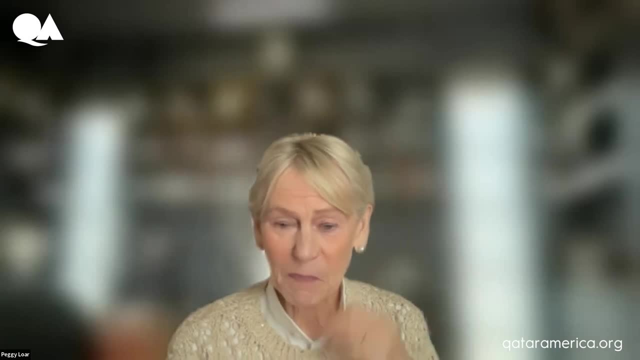 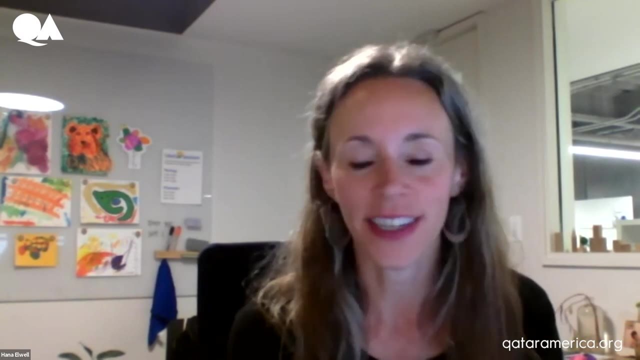 Yes, yes, yes. OK, There are quite a few and an increasing number of academic programs that are museum-focused, whether they're museum studies or the like. OK, But I think the truth is that people come to the museum world through many diverse and circuitous. 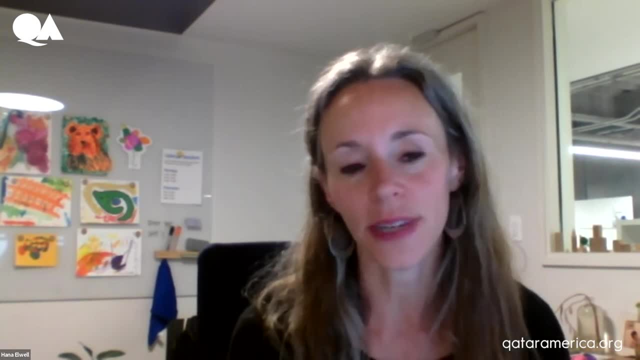 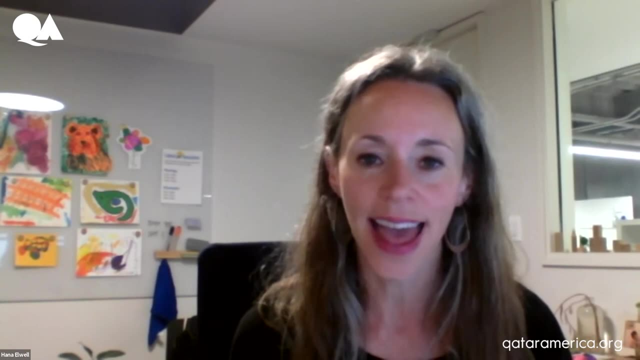 channels, And that's, in some ways, the beauty of museum work- is that it really is, at its core, interdisciplinary work that combines so many different fields and disciplines. And so, while traditional academic programs have so much merit and really introduce you to so many different facets of museum work, 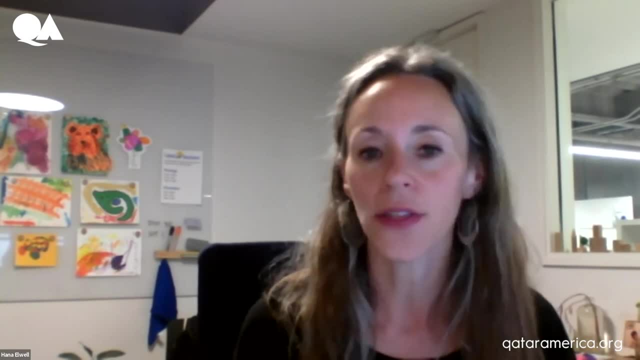 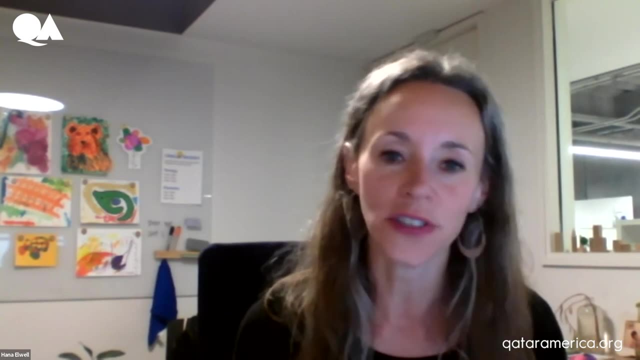 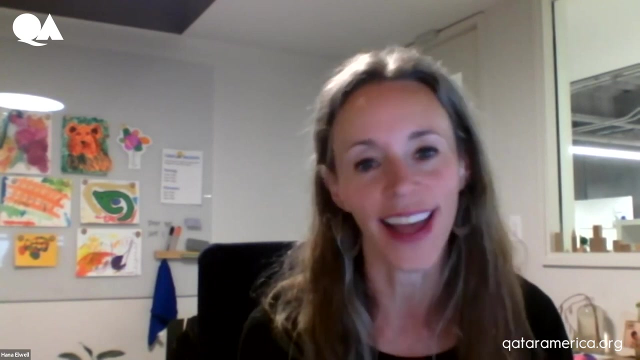 there's also so much practical experience to be gained in a hands-on way, Through different informal learning environments, whether that's through volunteering at a museum or another cultural site that does family engagement, or it may even be through a different mode, through a community center, through a library. 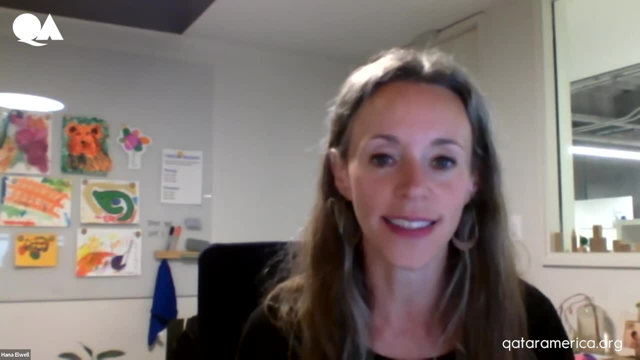 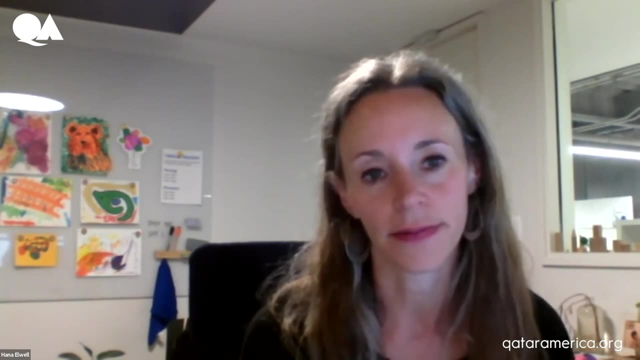 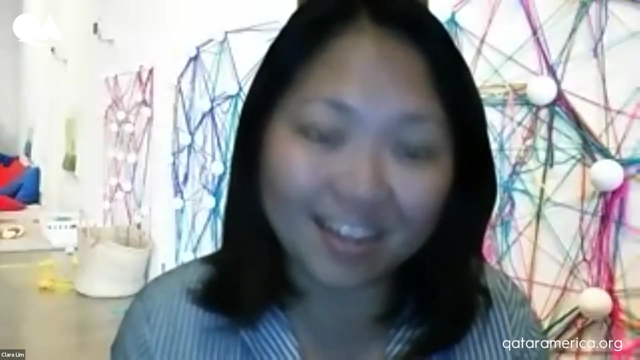 Any place that's interacting with families or kids of young age will give you some really valuable experience that can then be applied to the museum context From the Dadu Children's Museum's point. there are very few programs here. OK, We have a lot of programs here in Qatar. 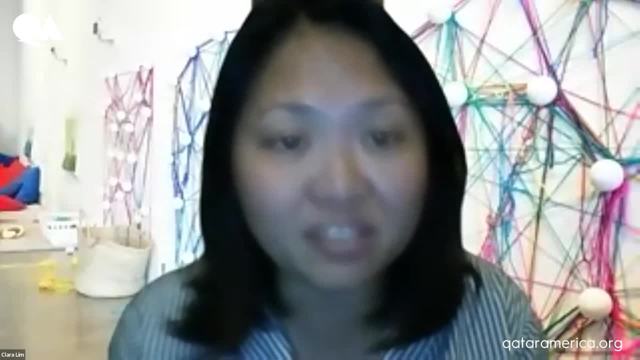 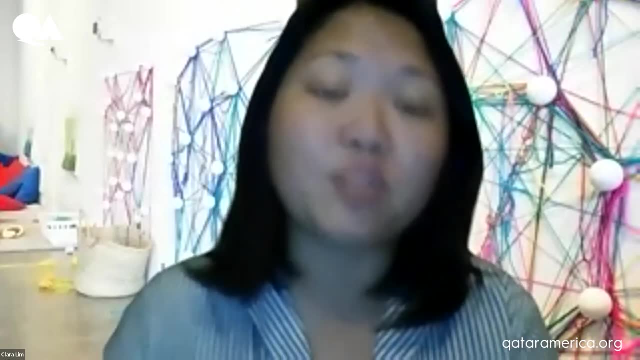 that there's no in terms of museum education or even child development psychology. there is a teaching university, So you can train to be an educator, You can train to be a teacher. So we do not have the same wide range of programs. 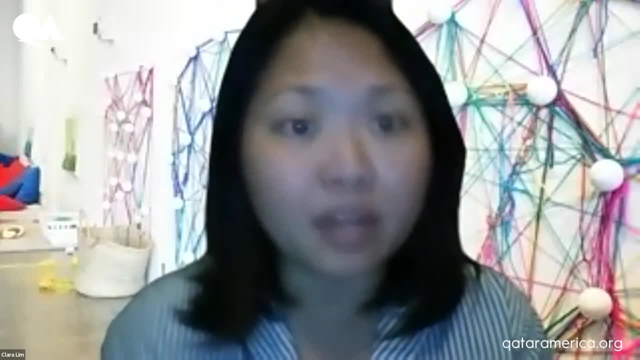 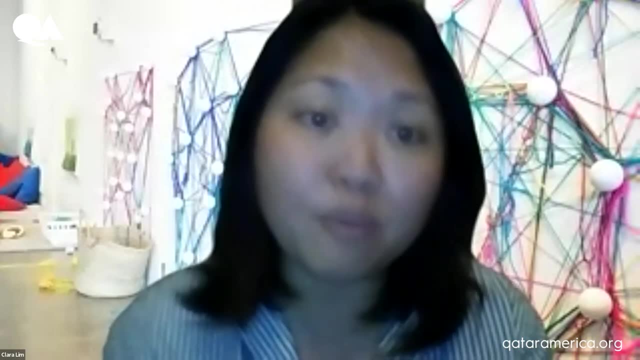 that's available in, perhaps in the USA, But the team, the Children's Museum team, the Dadu team, it comes from a vast number of different backgrounds. We have design designers, we have graphic designers, we have interior designers, we have a couple of engineers. 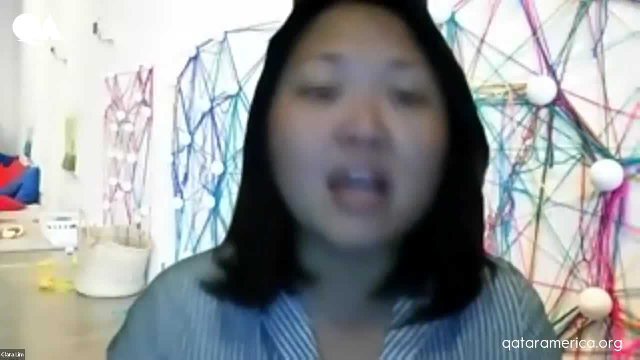 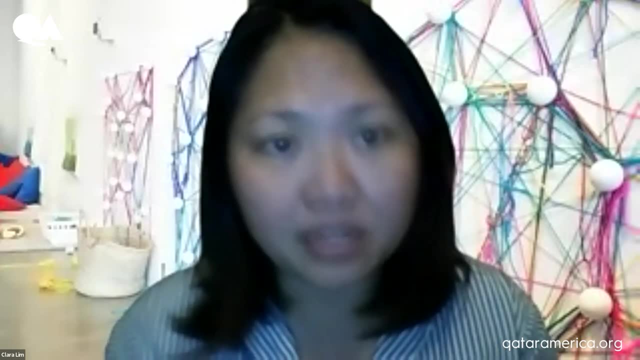 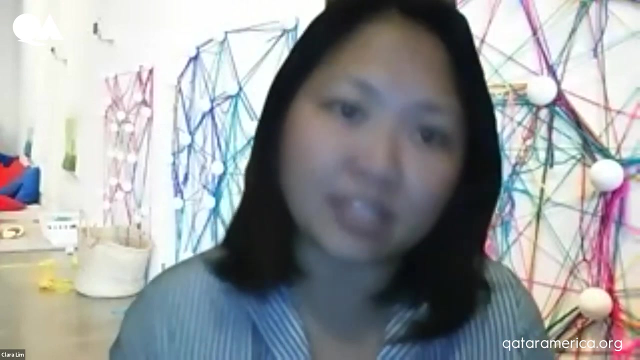 we have chemical scientists. The important thing we feel is the passion for the beliefs of the museum that we are working for children, we are working for families and we are able to be role models. We're able to bring the skills and our knowledge. 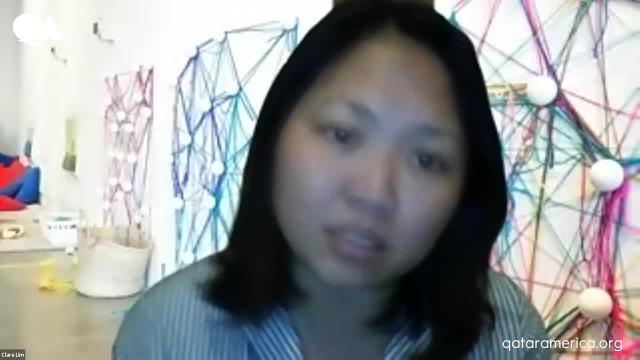 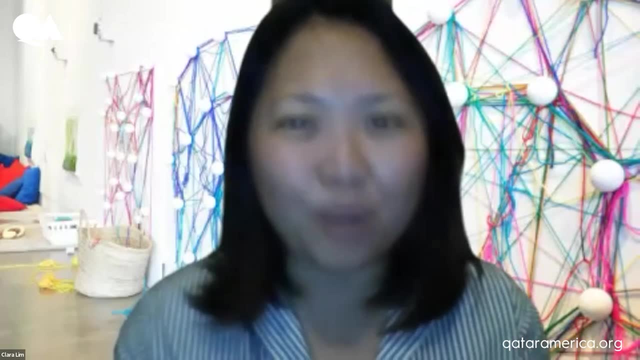 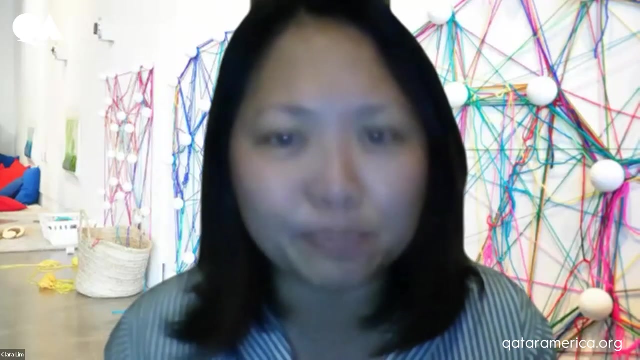 but we also have to bring an incredible capacity to learn, not just from each other but from the people outside of the museum, outside of the field. We also talk about, within our museum, working for children and working with children And the way we sort of look at it is not everyone who is as passionate. 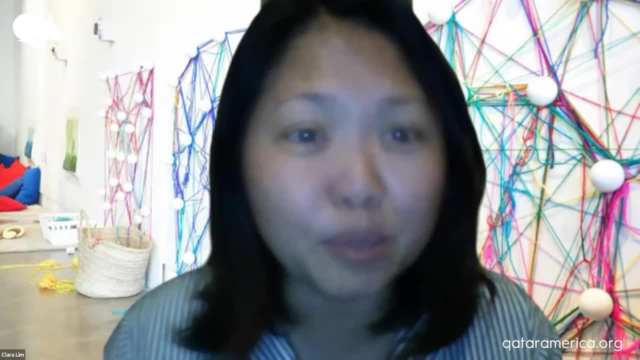 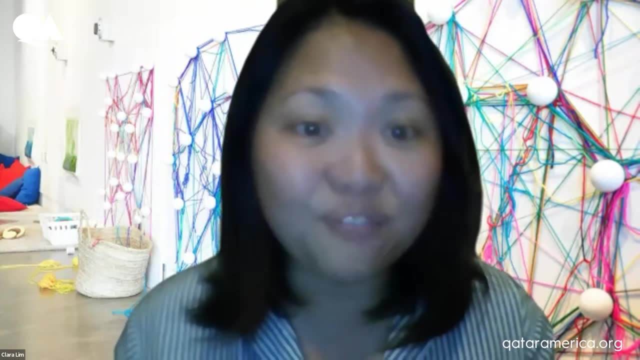 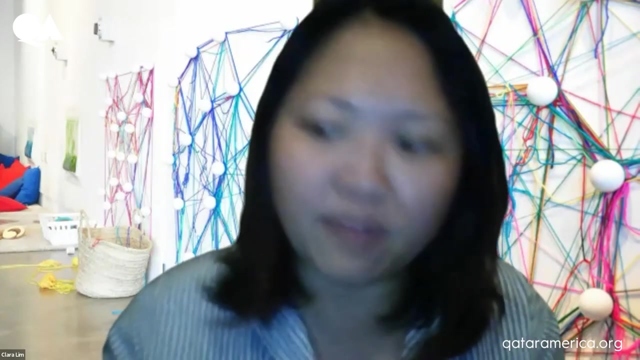 and has a lot to contribute, is actually natural and comfortable to be working directly with children, And that's okay because we have a lot of work to be doing back of house. If you do understand child development psychology- or you do understand it is- you know certain things that can support in curriculum development. 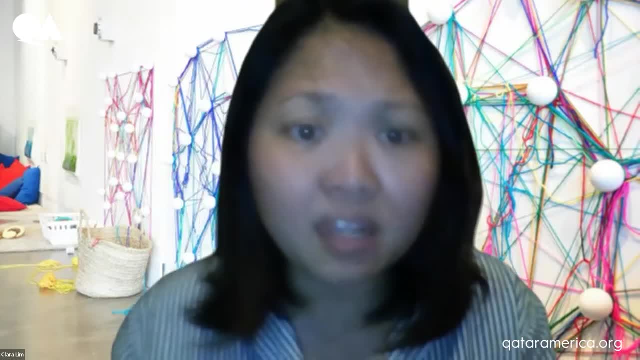 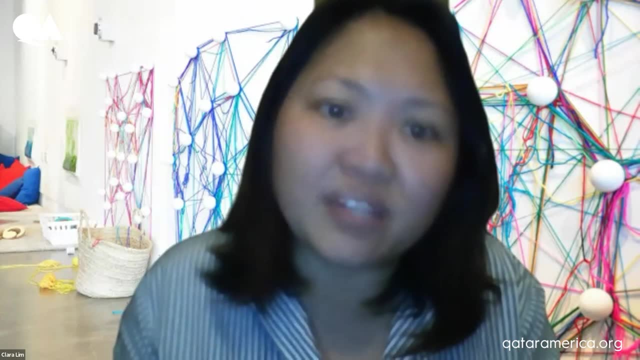 design of a workshop, engineering of an exhibit- great, You don't have to be front and center working with children. So a lot of times people say: you know, do I have to work with children directly? We'll go, no, but at some point you will have to interact with children. 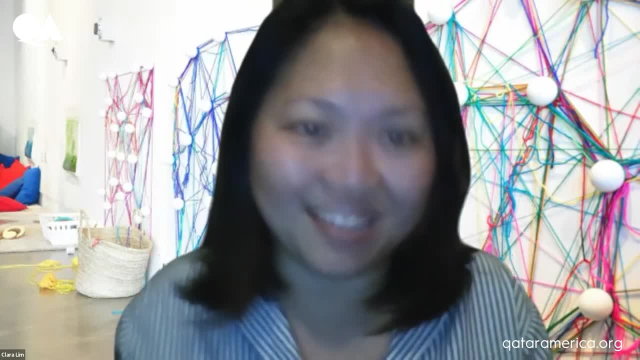 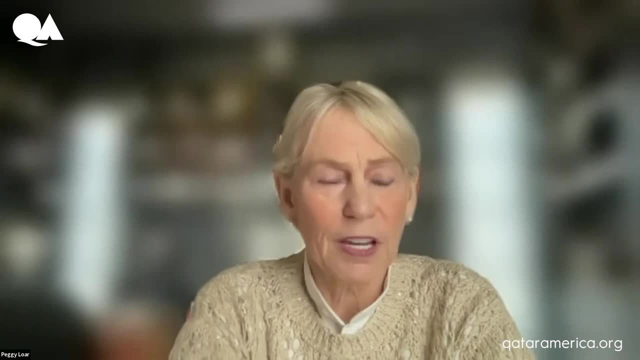 You know, when you're prototyping, you have to see how the children are taking it, but you do not have to be there with a child every day, You know. the other thing that comes to mind is: are we staying ahead of these kids with technology? 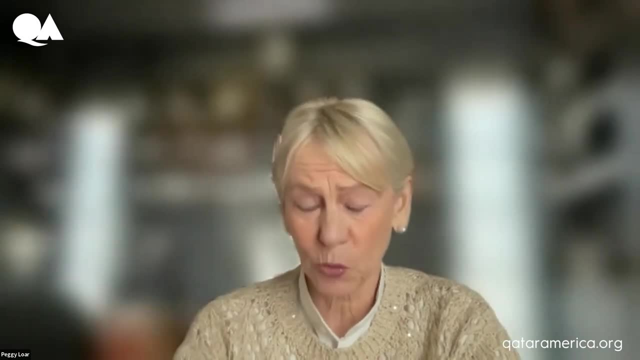 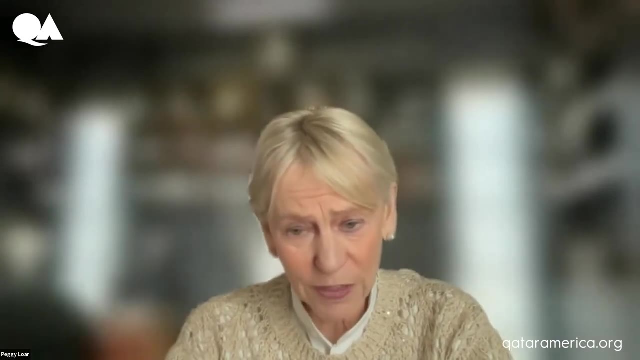 They are so smart today- smarter than most adults- And you're doing design, Clara, So you really have to stay on top of all the IT issues and things, But how's Brooklyn doing with the interactive situation that you've got there, which is expensive? 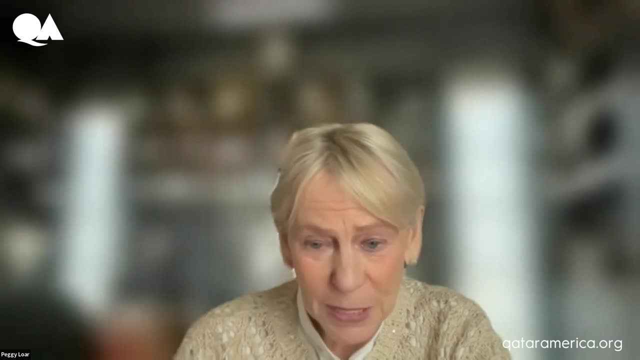 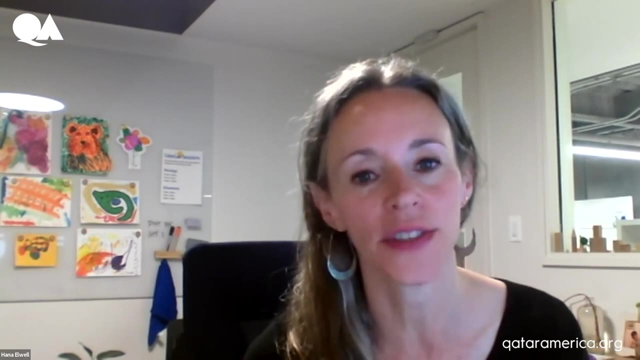 Did you hear me, Hannah? Yes, yes. So we've determined that really we think that our strength is to really focus our design and our exhibit Interactive experiences on the most tactile. So we have, over time, really taken out a lot of the technology. 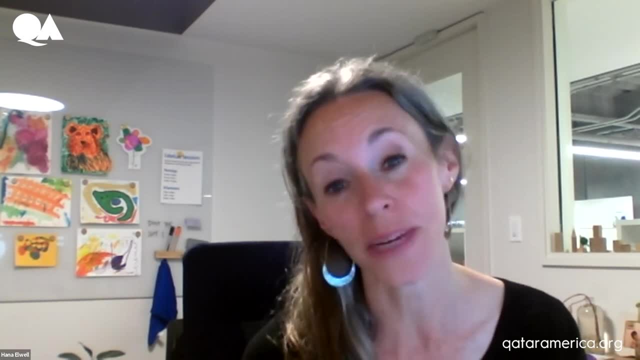 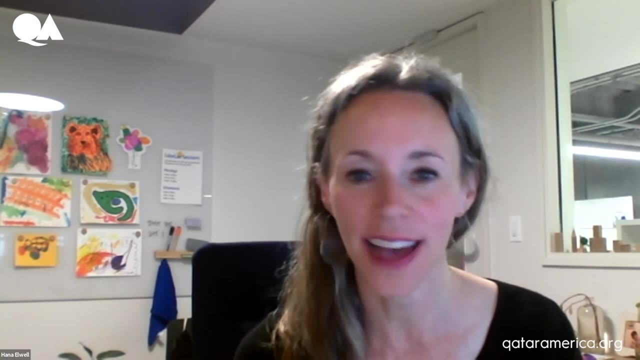 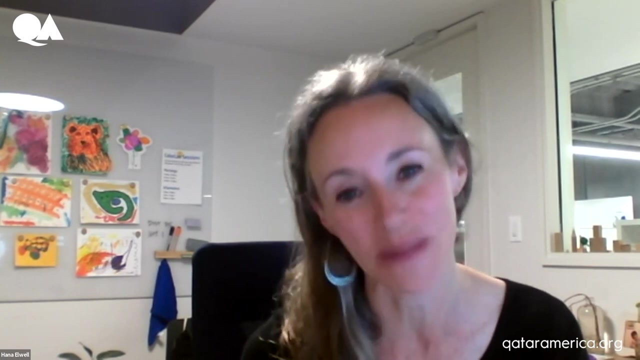 which, quite honestly, our current permanent exhibits were developed in 2006 and opened in 2008.. Between that time, the iPhone was introduced and the technology that was presented on the floor and the software that was developed was really outdated the moment the museum opened its doors.